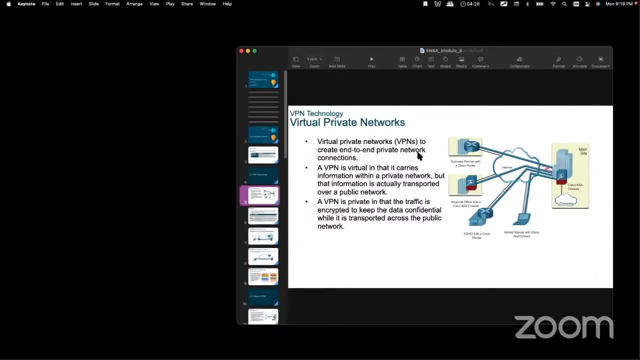 VPN is a virtual private network to create end to end private network connection. Okay, So let me give you one example. So a VPN is basically like a vpn: that we can go to a remote place and connect to the internet and the mobile service. 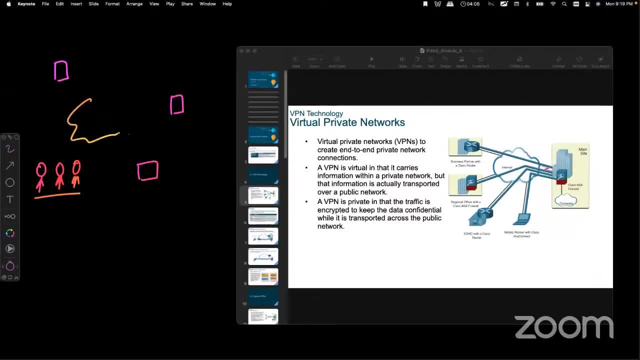 You have an office in Delhi and you have office in Mumbai and you have office in Chennai, Okay, And maybe some of your users are working from home, Okay, So they are using vpn for connecting with their office, So over the internet. So when you want to connect to Delhi branch, 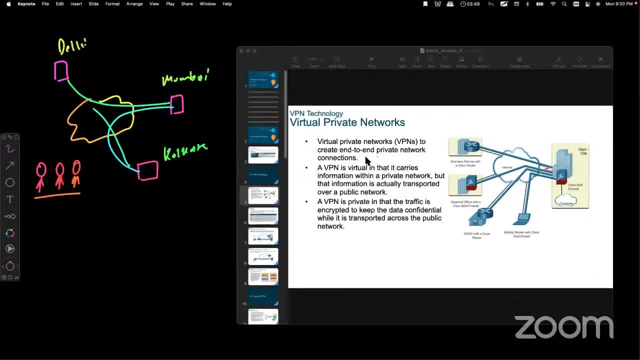 your Mumbai branch, Kolkata, Mumbai and Kolkata, like this. So this is called VPN. Okay, So VPN is a virtual circuit. Okay, VPN is a virtual circuit which will help us to make our private van. Okay, So, because private van is a secure, so tell me if we are. so suppose this is a bank, Okay? 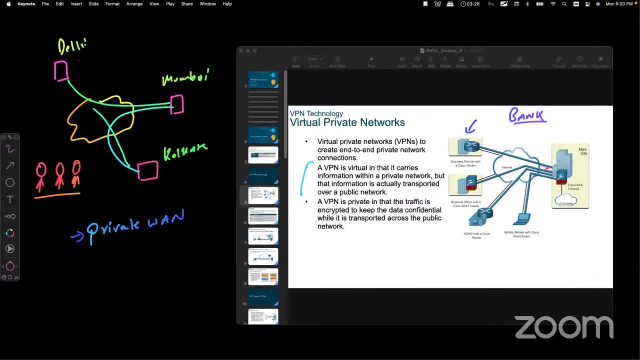 We, we, we are working for a bank. So if we have a branch in Delhi, Mumbai, Kolkata, so we can we share all the details, transactions, everything over the internet on with internet public van, So can we share everything about our. suppose we work for HDFC bank, can we? 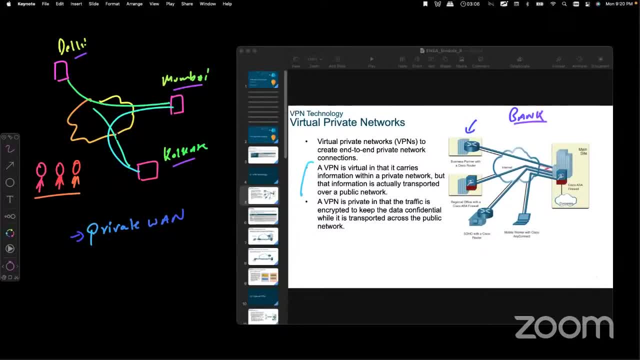 share all our Google sheets and customer data over Google drive? No, Right, We want, we want security, right, We want security, Correct. So these are worth. private van is very important. So you have two types of van. One is private one. 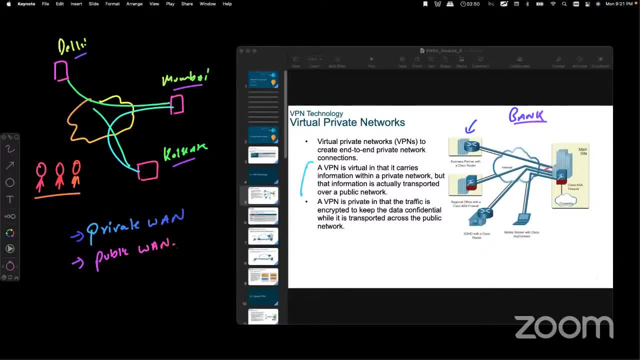 And one is public one. So public van we all are using right now, which is called internet and private van. We use multiple concept in private for private van. We need VPN. So VPN is basically end to end private network connections. So you can see, this is a business partner. 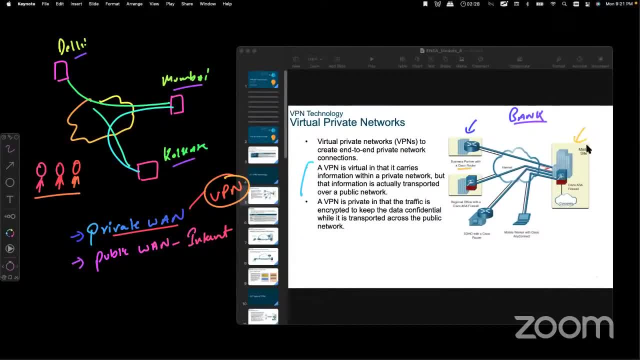 Okay, So over the internet, this is the main site, Maybe this is the head office and all these branch offices are connected with this head Office And there is a mobile worker, like, who is doing work from home, So he can also connect to this office. Okay, So, these type of van guys, this type of connection is called. 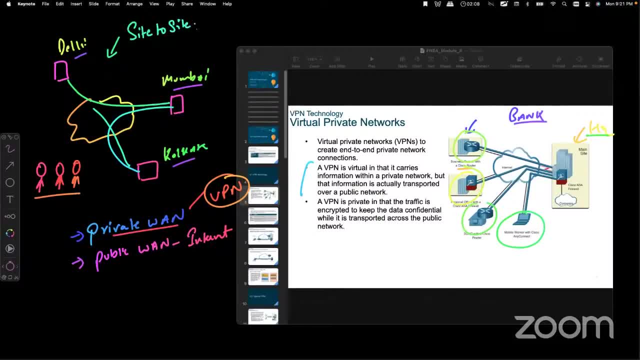 site to site VPN. Okay, When we are connecting our location to location, that is called site to site VPN. And when, when my employees, or maybe the mobile workers, they are using their laptops and connecting the VPN From any software which is connecting to the head office, So that VPN is called remote. 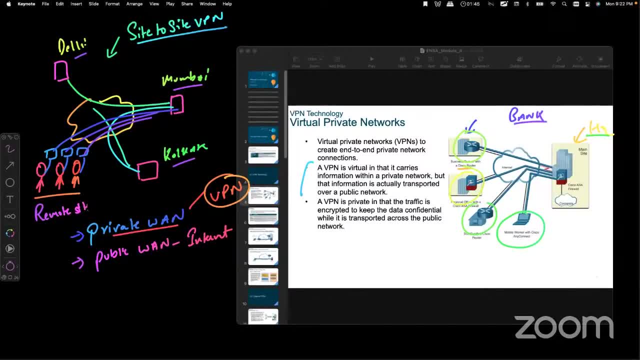 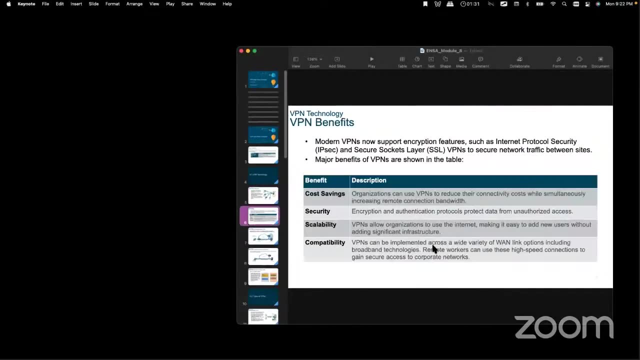 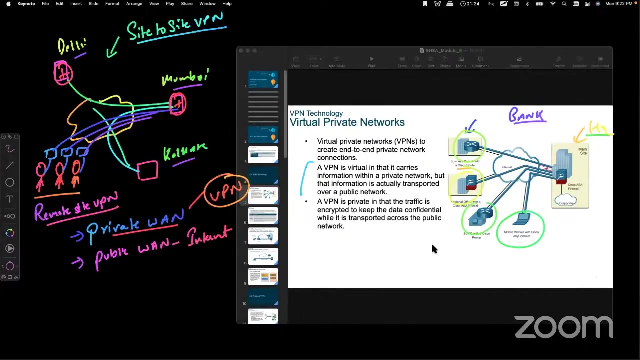 site VPN. So what is the difference? So when we connected our daily and Mumbai location to location, that is called site to site VPN, And when the users or employees connect to the office, that is called remote, remote site VPN. Okay, So usually when we talk about VPN, so VPN is. 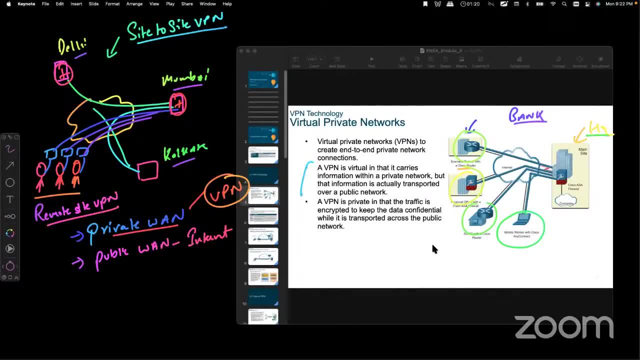 also encrypted the data so that nobody can access the data publicly. So if we are sharing data over the internet, the data is not secure, So we will use secure VPN tunnel so that my data will be confidential. Okay, Clear everyone. Yes, I'm not getting your voice. 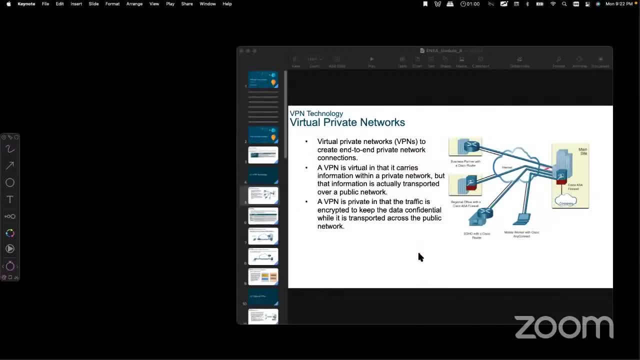 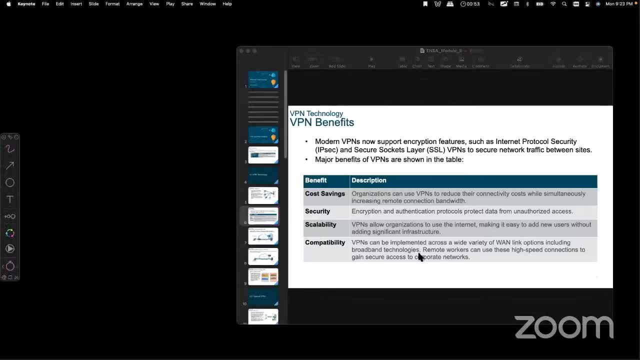 Yes, sir, Yes, sir, Yes. Okay, So, when we talk about VPN benefits, so what is the benefit? So, first of all, the cost benefit. Okay, So the first the benefit is: So we do not have to buy private connections, suppose, if you want to connect a delete to Mumbai or maybe. 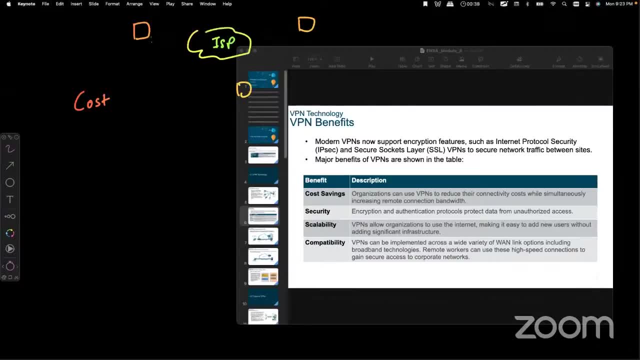 Kolkata, If you ask the internet service provider to connect to my Delhi office, Mumbai office, Kolkata office. So this solution is very costly, Okay, So this solution is very costly, Okay, But when we use a VPN, because VPN can be used as an, as a seeking a receiving a return, Okay. So check that if you want to connect a delete to Mumbai. Okay So, this solution is very costly. Okay, So, when we use a VPN- because VPN can be used to ID your feed, right, That's a cartoons to do a connection, Queen, where the user can see this here to Australia. Yeah, And so I've been. 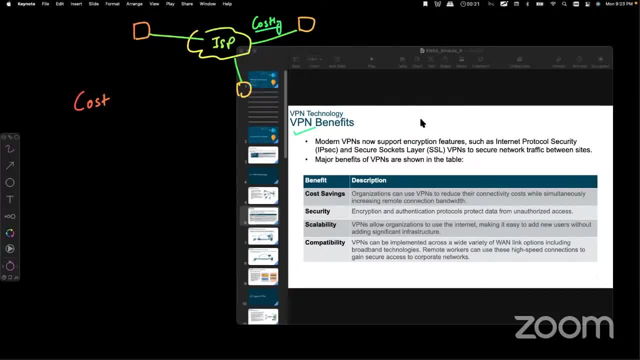 be used over the internet. okay, we will use one protocol which is called ipsec. okay, so we will use this protocol, which is called ipsec, over the internet to secure my connection. so what is the first benefit? cost saving. second is we are getting security, and third is scalability- scalability- 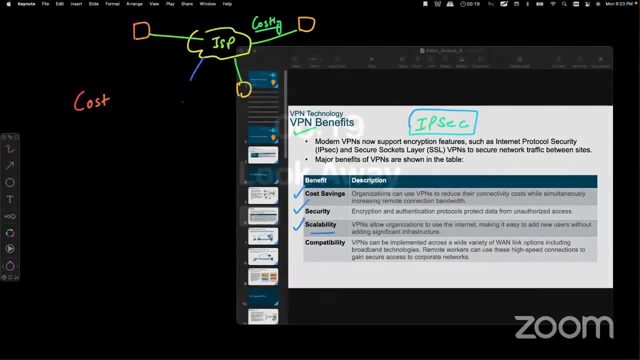 means, suppose you have three branch offices, maybe in future you have five more branches. okay, so over the internet, just you have to connect your offices with the vpn and vpn can be like, implemented across a wide variety of van links. okay, you can have a vpn on the 4g links, you can have vpn on the internet links, broadband links, so you can use any type of 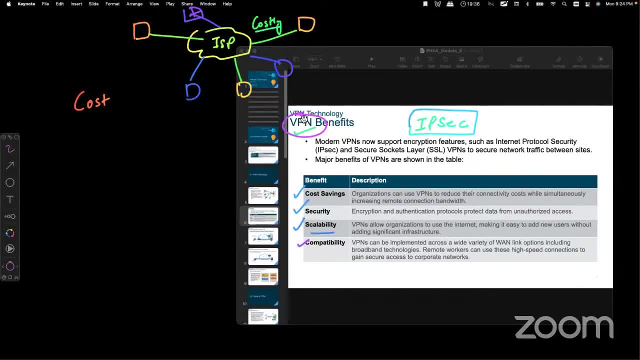 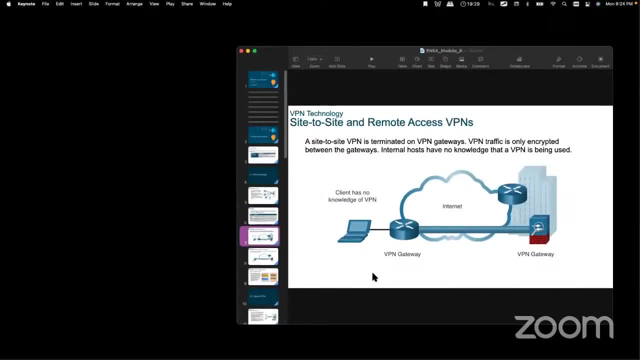 connections to use the vpn. okay, so let's go ahead. okay, so this was the first vpn. i told you guys what is this vpn? this is called site to site vpn. so when my company, my company router, is connecting to my head office router or maybe a firewall, 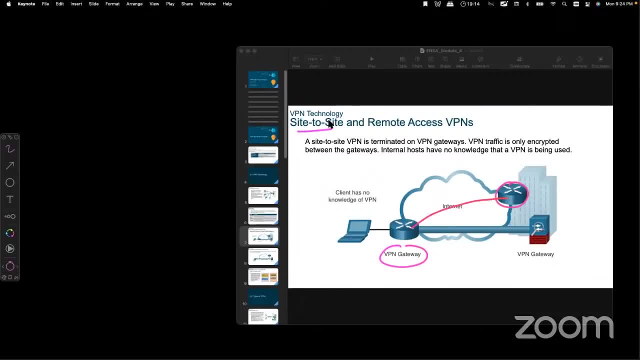 okay, so this type of connectivity is called site to site vpn. okay, so a site to site vpn is terminated on vpn gateways and it is only encrypted between the gateways, so internal computer will not have any information. suppose you have, you guys are working in a delhi office, okay, so maybe, uh, you are working as an accountant or 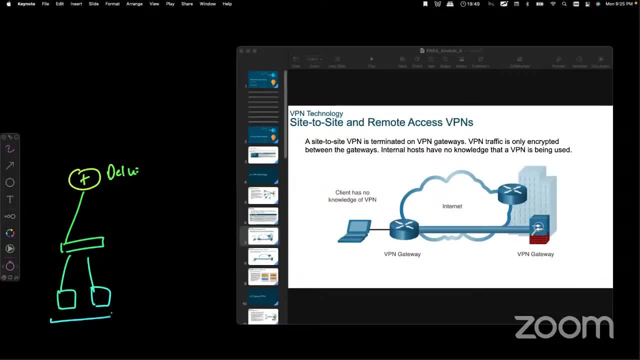 maybe a sales team member. so when he, these employees, never come to know, okay, what, how my traffic is going because delhi router, on this delhi router we have configured vpn and on the mumbai router also, we have configured the vpn. so this type of vpn is called site to site vpn. 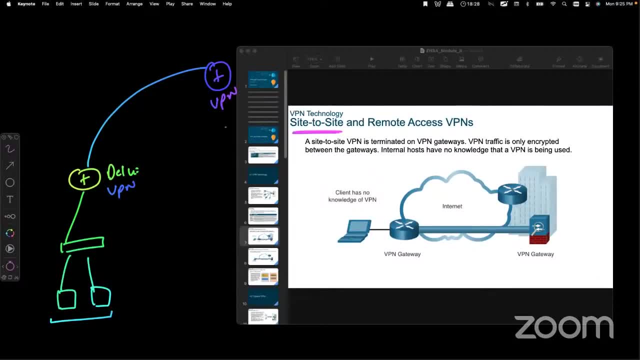 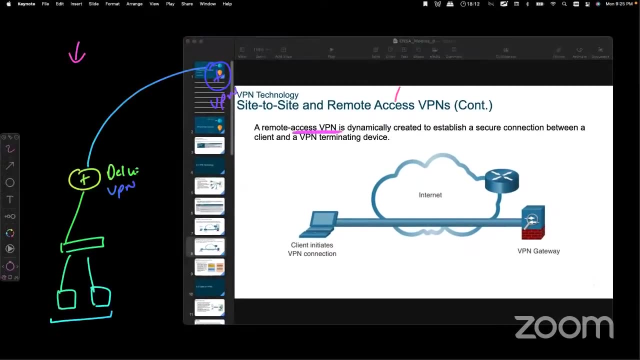 uh, i'm on my full screen because i want to write here. this is why my ppt is on the small size. okay, so when we go further. so this is a remote site. vpns also. so when the client: okay, when the client is going to create vpn connection with the routers. so this is usually. 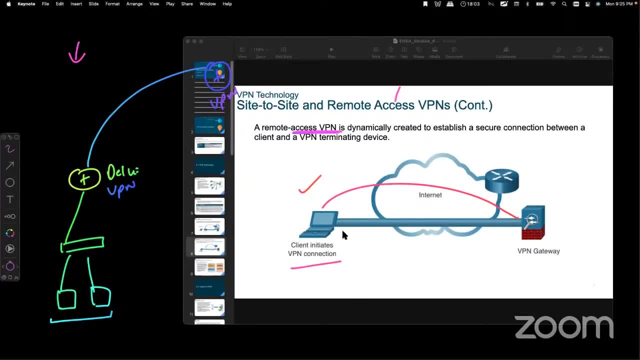 happens when i want to connect to the office while doing work from home and i want to connect to the home or any kind of suppose. i want to suppose there is a company server over here and i cannot access server over the public network. this is my private server, so how i will access this server? 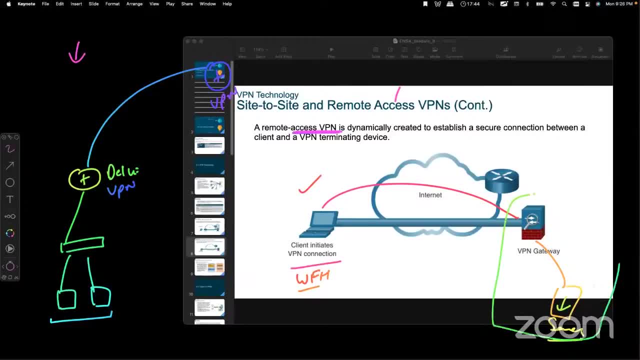 because this server is in my office. so i will how i'm going to access this private server. if i, if i connect with the vpn and if i am virtually present in my office, okay, then i can connect to this private server. so, okay, let me give you one example of a private server. 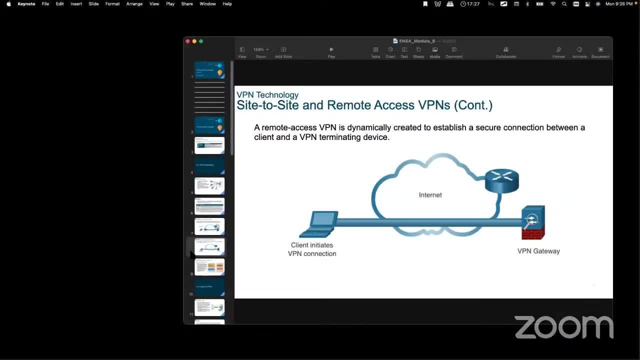 okay. so guys, uh, suppose my this is my laptop. okay, i'm currently connected with the broadband connection. okay, this is a normal wi-fi, so my computer ip is 192, 168, maybe 1.3, so this is connected with this broadband. and this is 192, 168, maybe 1.1. okay, so this broadband is over. 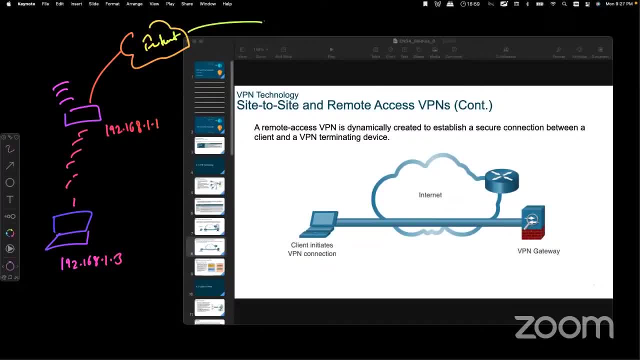 connected to internet. okay, and we have a office- maybe a different location- and in this office we have server here and this server is working on 10.1.1.1. okay, so this is our office, just hold up, okay. so now, if i connect this laptop, okay, over the internet, i. 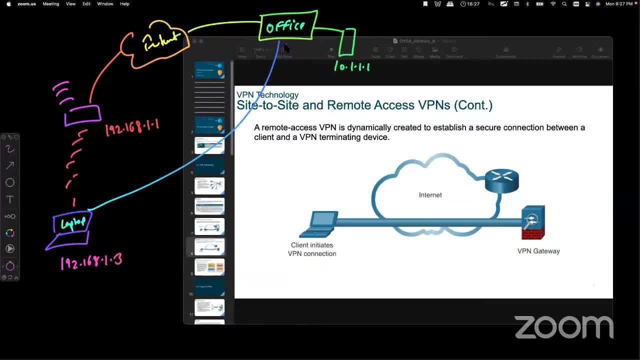 connected this laptop to the office router, so i will be virtually present in my office and i will get a different ip. maybe i will get 10.1.1.2. so now this is my vpn ip. so when i connect to the office vpn i will enter my username, password and i will be virtually present in my office. 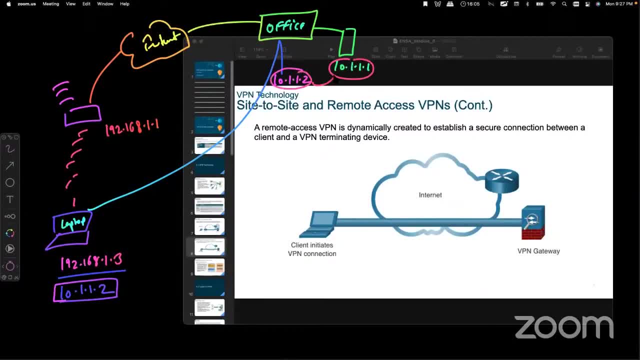 and now my laptop and the server are in same network, i can access this, my private server. okay, so this type of connection is called remote access vpn or remote site vpn. okay, remote access vpn is a better term, so let's go ahead. okay, now. this is very important, guys, like when we talk. 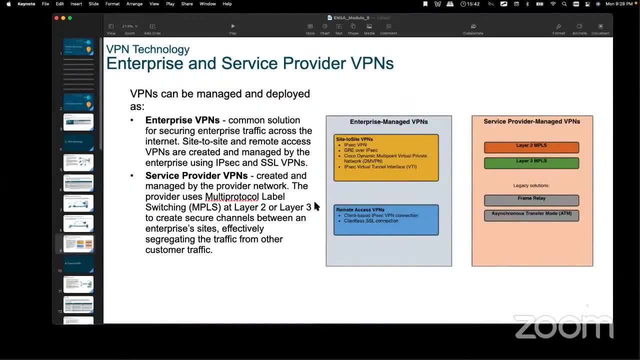 about vpn technology. people get confused. this is why i'm taking this session on youtube also, so people think that vpn mpls is also vpn- then why we are using ipsec. okay, so let me tell you, as you guys are from ccna, i'll not actually confuse you. so this is enterprise managed vpns. 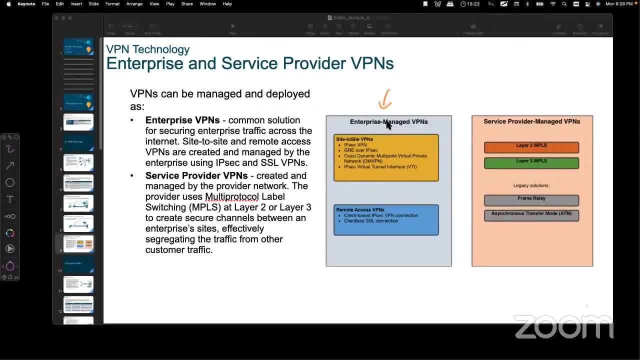 so, like, suppose you are working for a company like nestle, cadbury, dabber, these kind of product based companies- okay, then you. then, if you configure vpn, you will configure these vpns which are called site to site vpns, or you configure remote access vpns. okay, but when we talk about the service, 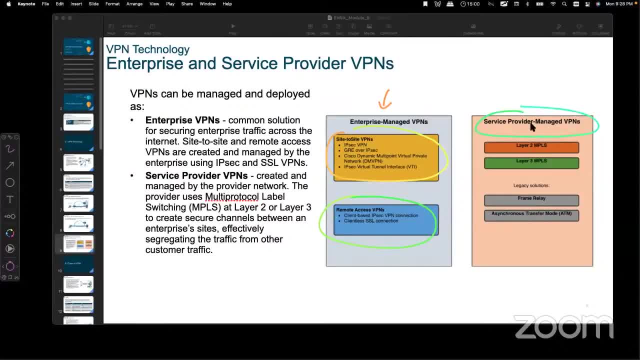 provider vpns. so these are different vpns. so these are different vpns. so these are different vpns, different ones, so these are not actually vpn, these are called vpn services. okay, so so this is called mpls technology. so we have layer 2 mpls, layer 3 mpls. so as a customer, you will not run. 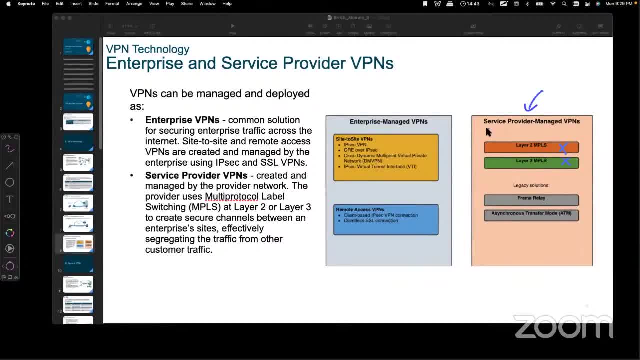 mpls. so when you become a service provider, so if you are, if you are atl, if you are reliance, so these companies uses mpls okay. so if you learn mpls you will be able to apply to the service. but if you want to stay with the enterprise companies, like product based companies, then 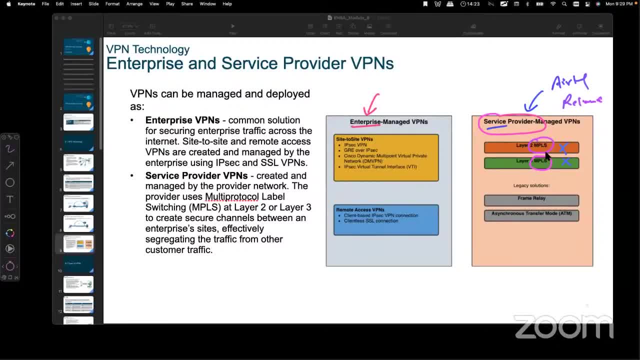 you might do not need require the mpls knowledge also. okay, so yes, various companies are looking for both mixture. okay, that's the different case, but yes, so when we say about enterprise vpns, so these are the normal vpns, which is actually over the internet, we connect our office. okay, 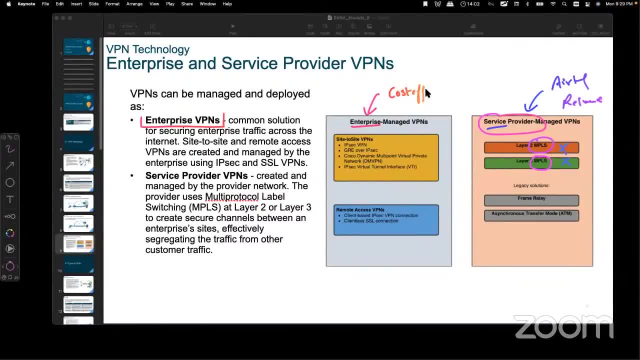 this is a cheap solution, the. this is cost effective. but if customer wants to connect his delhi, mumbai, chennai, all the branches with the isp, that is called a service provider, managed vpn, this is called mpls. so in short, let me give you one more. 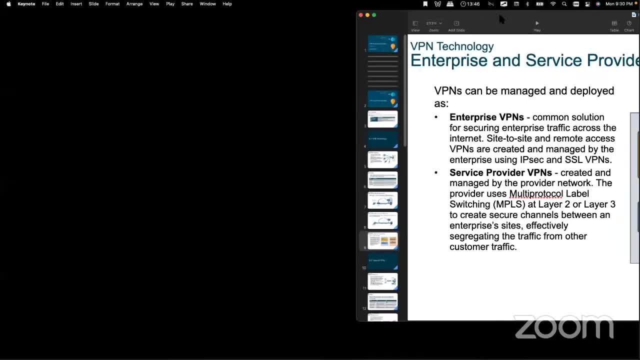 idea. okay with the practical. suppose i have 100 employees. okay, so i have four or three branches. okay, i have three branches, so maybe this is my delhi office, this is mumbai, this is chennai? okay, so over the internet, i will buy the normal router and i will buy the normal router and i will 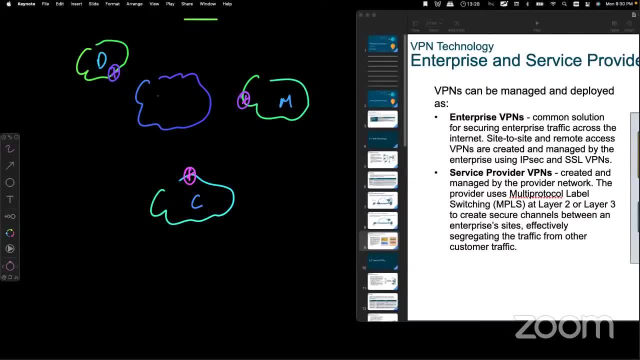 buy vpn, so over the internet i will buy. over the internet i want to connect all my office with the internet. and over the internet we are going to make, we are going to create all, or we are going to connect all the offices with vpn. so now the question is why we want. 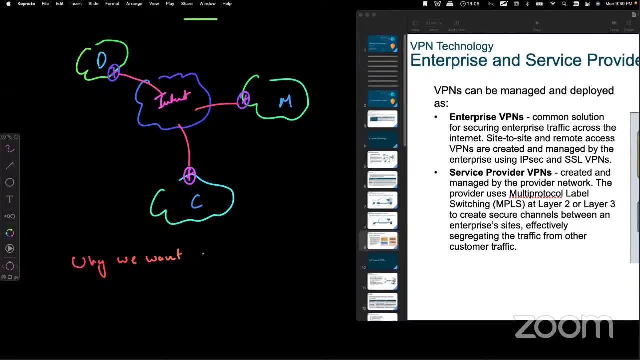 to connect with vpn. why we want to connect with vpn? yes, anybody from the company. why we connect with vpns guys? yes, show your vision. using vpn, where my friend is sitting, let me show you my vision of life, your knowledge. yeah, Dinesh, so that we can. 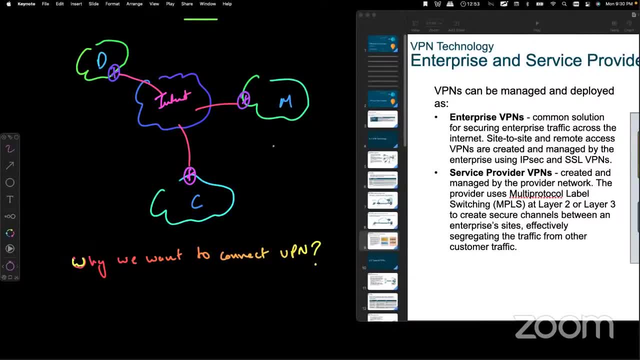 we can access internal server. yes, yes, so maybe in Mumbai we have server, okay, so maybe in Chennai we have some different, maybe different, maybe like some another server, okay, and maybe in Delhi we have a tele server. so we have different, different servers at different, different location, okay. 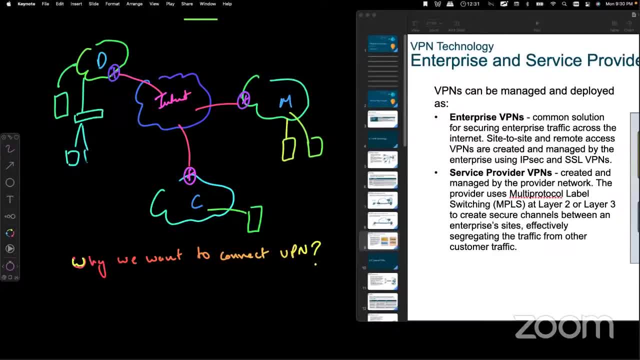 and we have a LAN network here. we have hundreds of users available in Delhi. okay, so now all these users, they want to access these tele server. okay, suppose these are accountants. so tele is basically a software for accountants. suppose these all four accountants wants to. 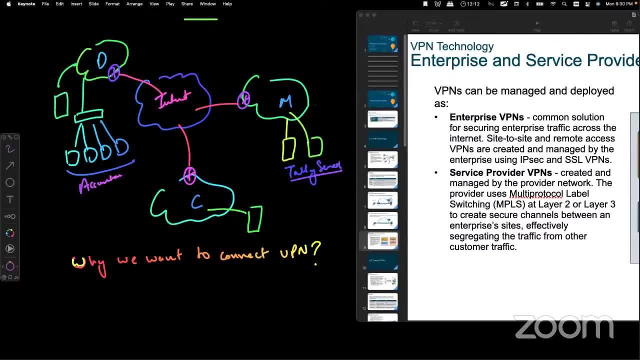 access the tele server which is in Mumbai. okay, so tell me what we are going to do. so we are going to connect my office with Mumbai office with the help of VPN and with the help of VPN, what will happen? my private network- suppose this private is 1.0. 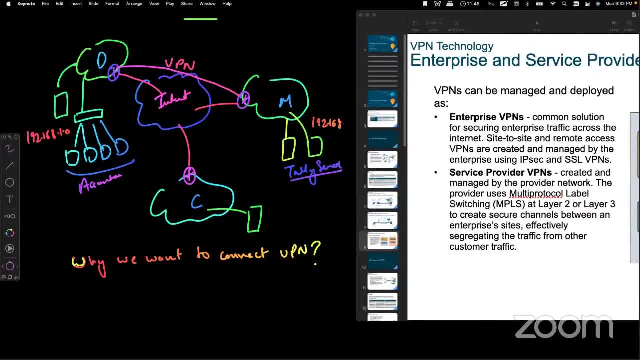 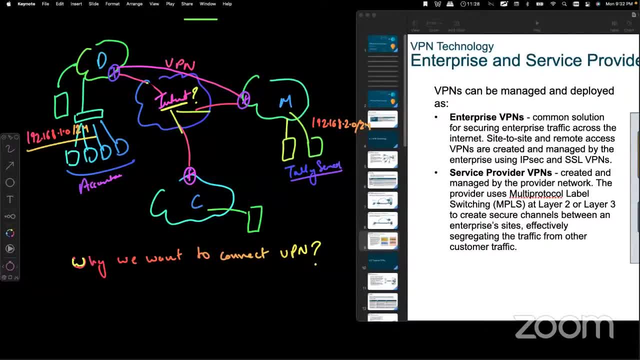 No sir, no sir, because yeah. so let me tell you the reason. because the routers which are used by ISP, so ISP routers block private IPs, so their ISP routers block private IP. so if the ISP routers are blocking private IP, so then how this VPN technology is able. 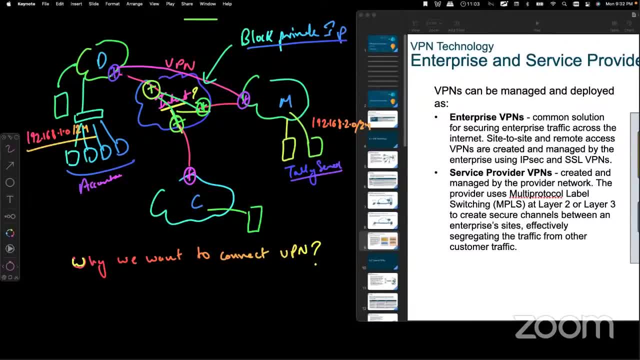 to connect what is happening. so we are actually building a tunnel. okay, we are going to build a tunnel and we are sending our private information inside the tunnel. that is basically called VPN. so we are hiding the information from public that we are not actually dealing with- the private. 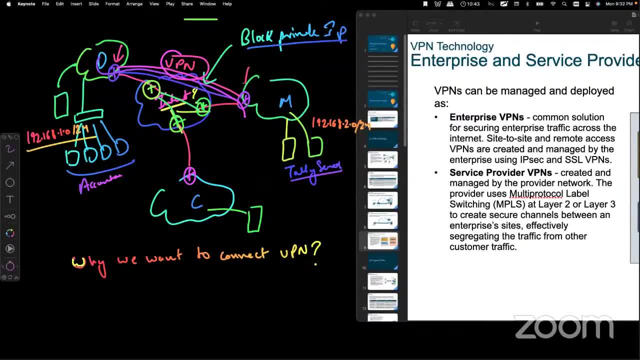 to private IP. we are dealing from this router to this router. that ISP will come to know. okay, the traffic is going from the Delhi router to the Mumbai router, but in actual we are sending my internal traffic inside the tunnel where tunnel is built between R1 and R2. 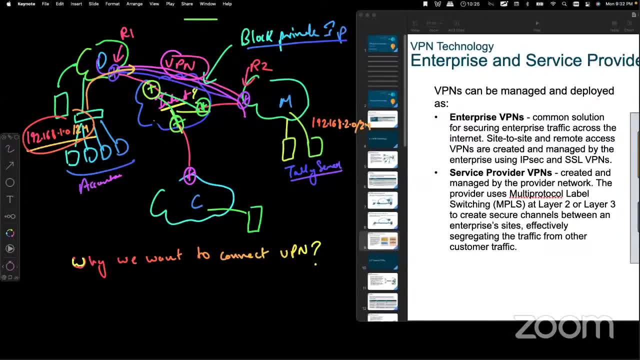 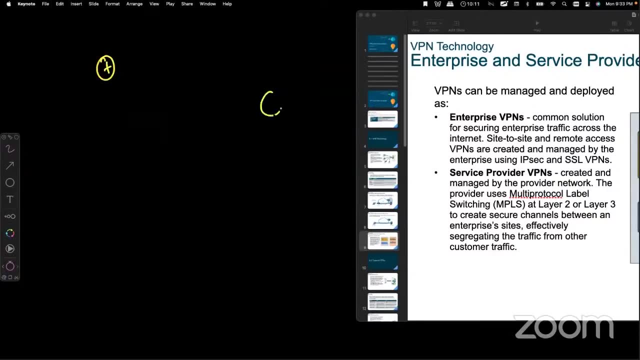 right between Delhi and Mumbai got an idea. yeah, this is. this happens when we talk about enterprise VPNs. but let's, let's understand now, service provider network. suppose you again, you have Delhi office, Mumbai office, Chennai office, okay, but now, this time you do not take internet. 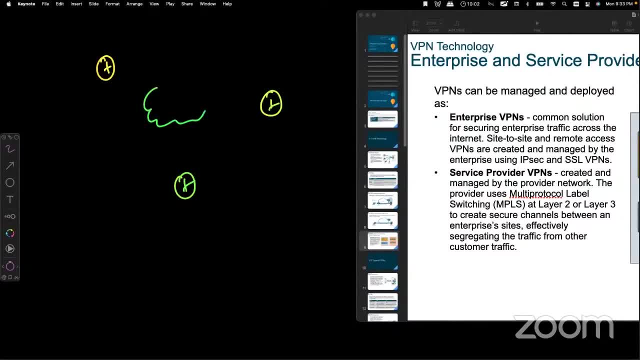 connection. internet connection is different. but you ask what isp? so you call ISP ATL. okay, that I want to connect my three offices. so ISP will use MPLS technology. okay, MPLS or other technologies also, so MPLS, so they will give you connection from their Delhi office. 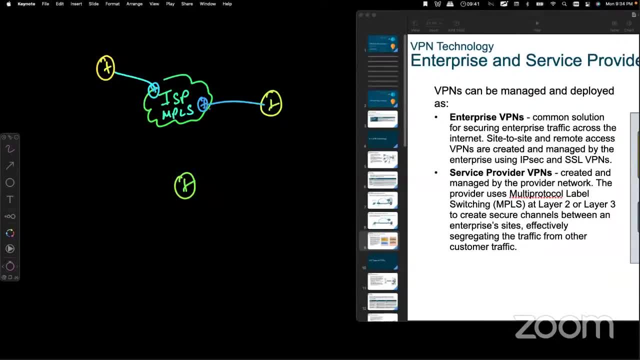 so they will give you Mumbai connection from their Mumbai office. so they will give you connection from their Chennai office, so over. so now you can see: ISP, internet service provider, ATL or any company has given me connection, so now they are going to create tunnels inside their network. 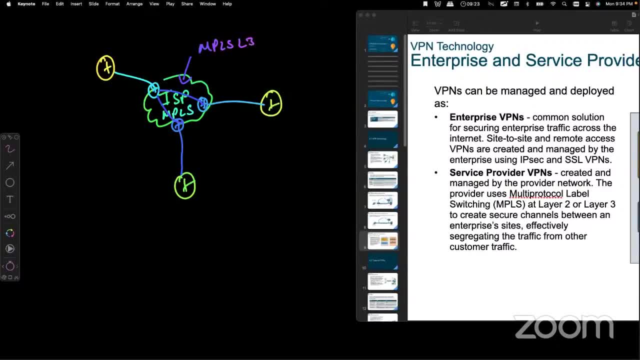 that is called MPLS, L3 VPN or L3 or L2 VPN. so L3 is basically when they make the tunnels with IP addresses. that's called L3. L2 VPN is basically when they use some VPLS or some advanced technology. okay, so means. 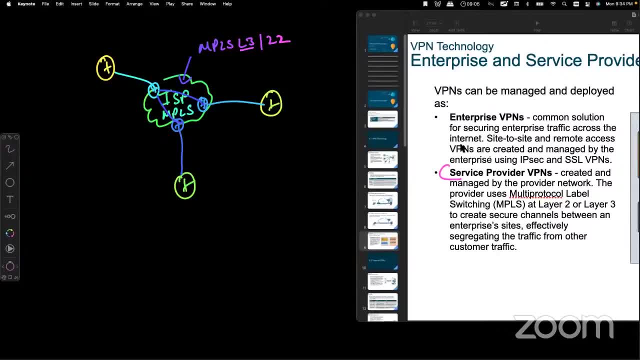 when we talk about service provider VPN, who is making the VPNs service provider? and when we talk about enterprise VPN, who is making the VPNs? the companies or we as enterprise customer? is that clear? everyone, yes, yes, okay. so what do you think? what do you think? 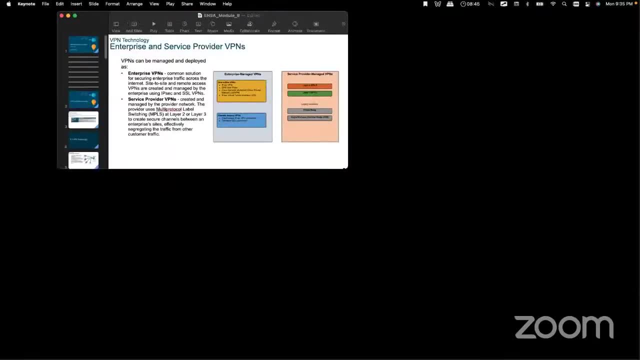 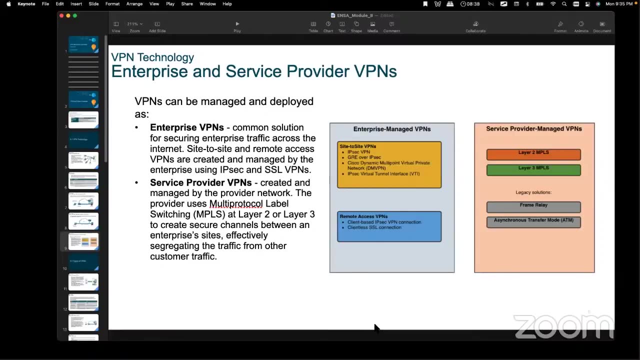 which is more reliable if you want to send a lot of bandwidth, if you want a high speed? so which VPN is more reliable? enterprise or service provider? service provider: yes, if you have heavy applications. if you have, yeah, so if you have very heavy applications, okay, suppose you. 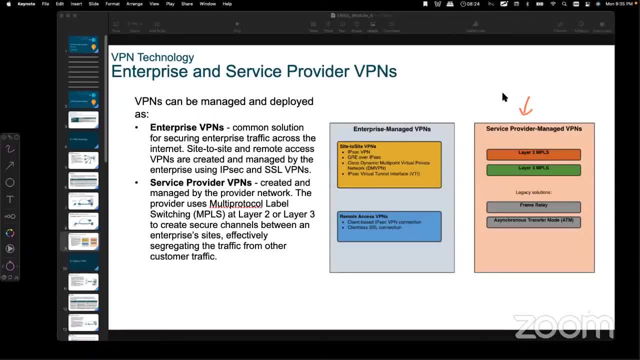 are working for a very good company like Facebook, LinkedIn, Apple, these kind of companies. so they do. they do not worry about the money, right? so they worry about the bandwidth, they worry about the speed, they want high reliability. so, if you want high reliability, which VPN is better? 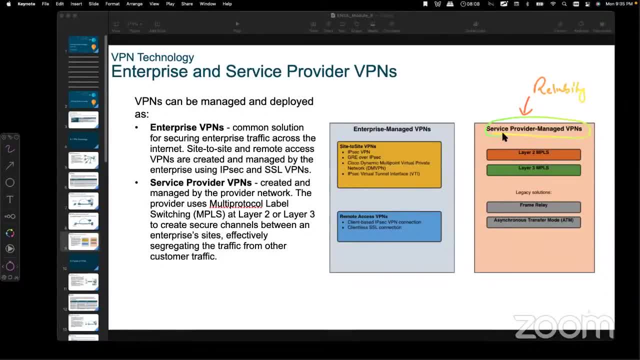 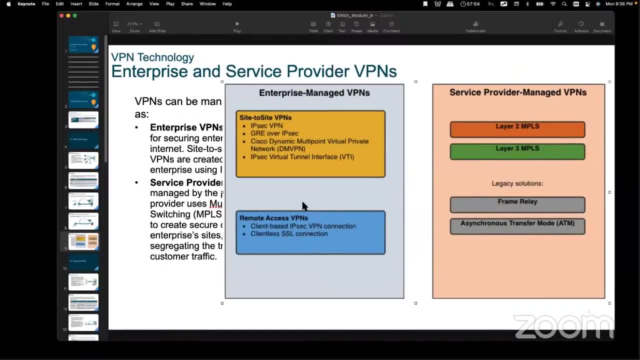 the service provider, okay, but if you want cost effective solution, which VPN is better? the enterprise managed VPNs, and there are a lot of VPNs. let me zoom in so that you will get to know what VPNs. so these are the VPNs. so first type of 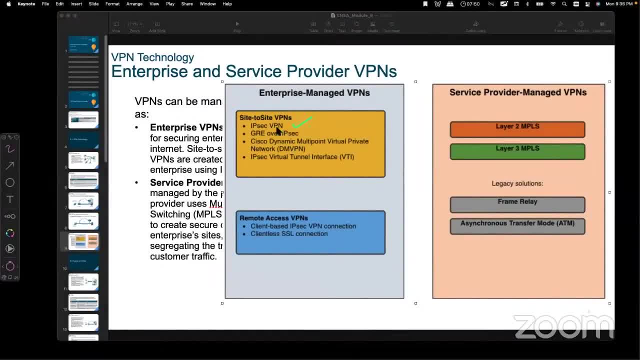 VPN is IPSec VPN, which is popular. so then there is a GRE over IPSec, okay. so then there is a Cisco DMVPN, which is called dynamic multipoint virtual private network. so this is another method: IPSec, virtual internal interface, VTI. I never use this. 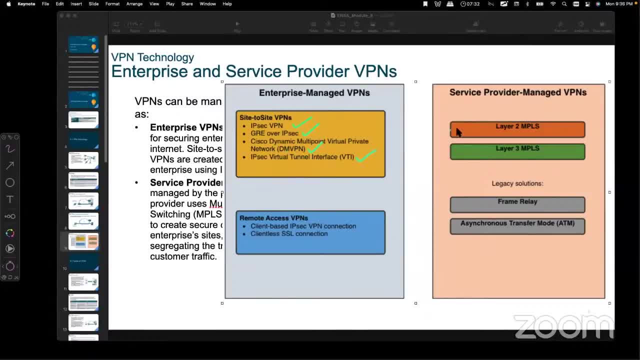 but yes, this is also a site to site VPN and when we talk about remote access VPN, so here this VPN is called a client based IPSec. this is over the IPSec and there is a client less SSL connection, secure socket layer connection. okay, so normally people 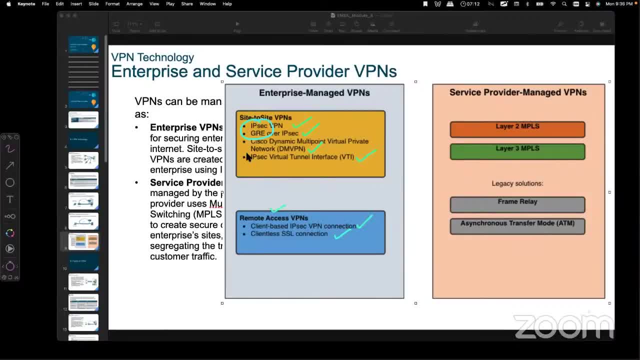 configure IPSec and GRE for their connectivity. but when we talk about the service provider network- layer 3- MPLS. layer 2- MPLS- okay, which is also known as VPLS- okay, virtual private line service- MPLS is multi protocol label switching. so these are the. 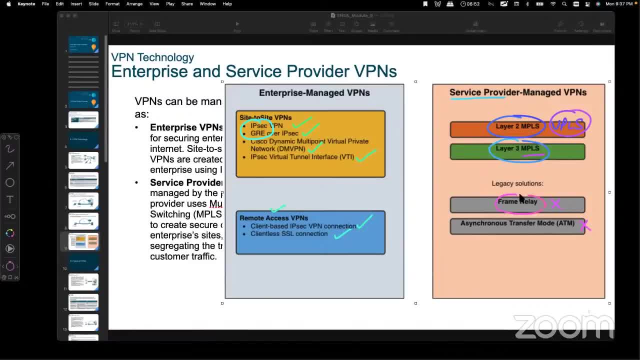 technology which are no longer. you can check frame relay video on our YouTube, but this technology is no more in the world. almost I think 1 or 0.1% people still uses frame relay, but still it is gone, so you do not have to waste. 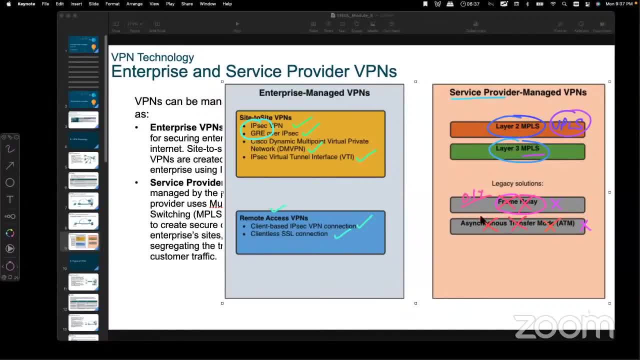 your time to learn these technologies: frame relay and ATM. so after this CCNA program, when you go for CCNP. so I am just giving an idea: this IPSec and all and DM VPN, so these two tunnels are in CCNP, okay, and this layer 3. 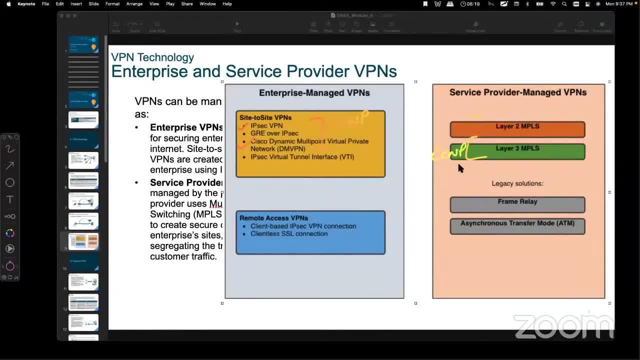 MPLS is also in CCNP enterprise. I am talking: okay, so this is not in MPLS, this MPLS is not in CCNP. but yes, we have added as a bonus topic in CCNP. but if you want to learn the complete layer 2, layer 3: 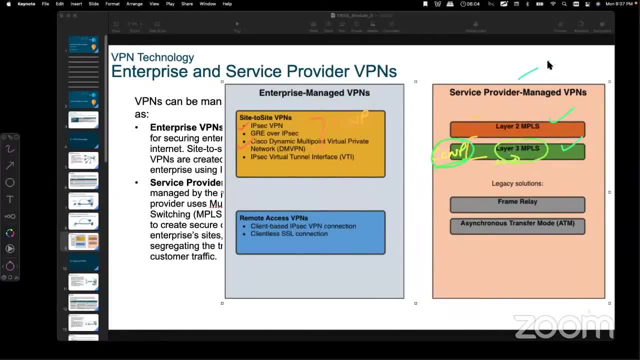 okay, these MPLS, so that comes under the CCNP service provider. so I think if you learn IPSec, if you learn DM, VPN, if you know about layer 3 MPLS, still you will become a very good engineer. okay, so the batch maybe after the CCNP. 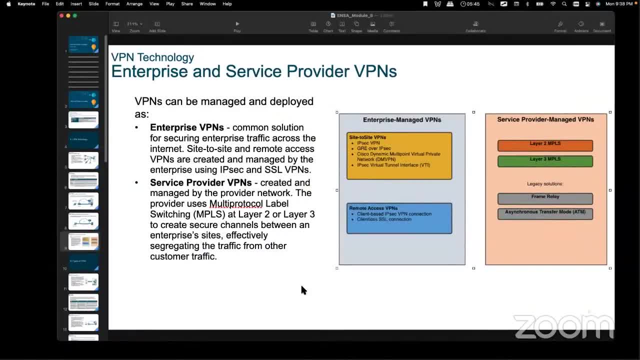 batch when the CCNP is coming, so you will be going to learn these topics also: IPSec, DM, VPN, all because, as a network engineer, you should know these technologies, because all the companies are working on IPSec, DM, VPN, GRE, so these topics okay. so when it? 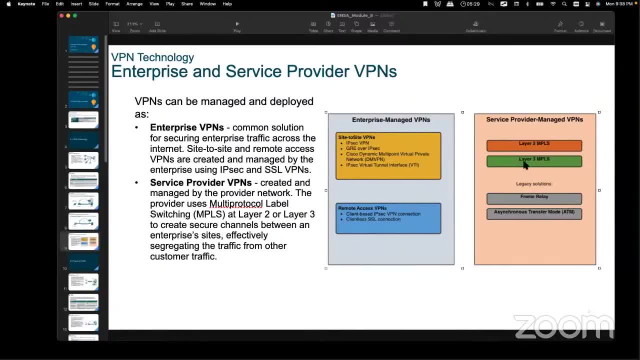 is when it comes to the service provider. so there it is known as layer 3- MPLS, and layer 2 MPLS is also getting popular, but it is a very advanced stage. when you learn layer 3, then you can go for layer 2, okay. 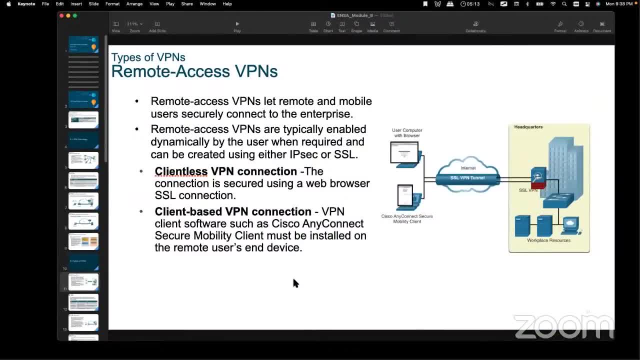 so let's go to VPN. so, as I told you, remote access. VPN means when your client okay, means when your worker, when your employee can access the office, okay, so so that they can access their private server. so what they have to do so they can go to. 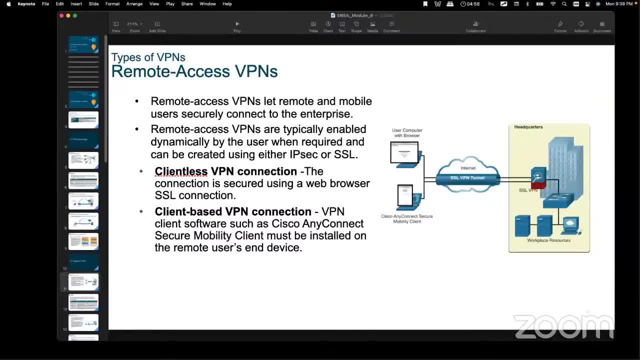 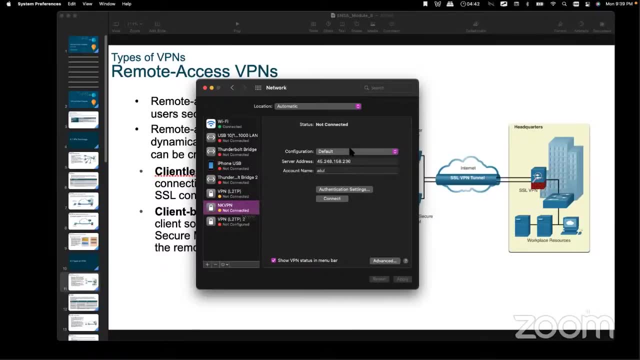 the VPN connection. so let me show you practically. okay. so let me go to my system, my network. so I have already created a VPN. so I'm using MacBook for Windows. I think you need to connect so you can see I have connected. so this is a VPN. 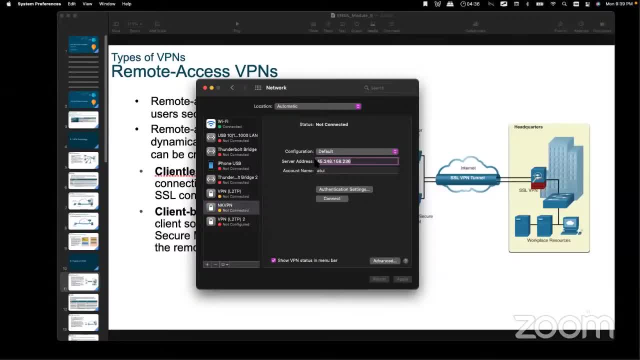 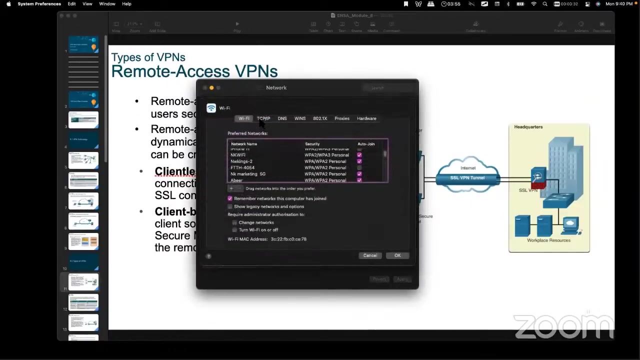 connection I have made. this is the router IP of my company. okay, so I'm going to click connect. okay, so I just wanted to show you guys. so I am getting here. you can see here. so what IP I'm getting here: 192, 168, 1.3. 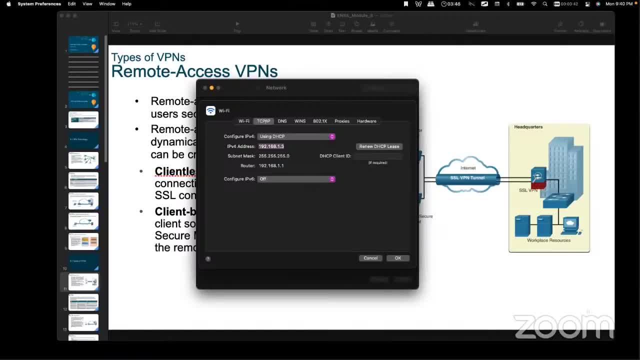 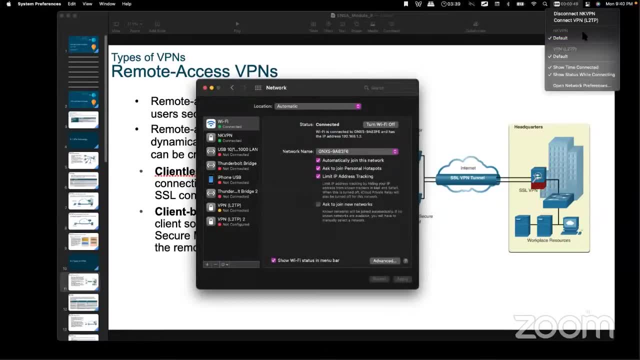 yes, hello. yes, okay, and I'm now connected to VPN. this was now you can see. so there is a timer going on in this laptop. you can see 0052 second. so I'm connected to my office VPN. so what IP I got from VPN 172? 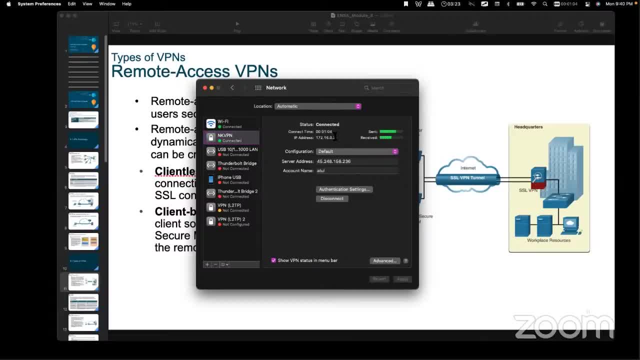 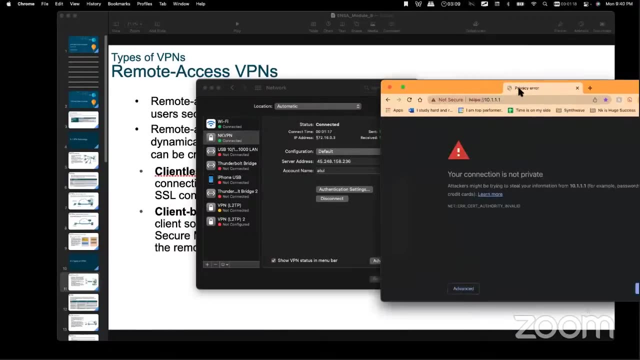 16: 0.3. can you see that my IP got changed? yes, yes, yes, okay, it means I'm in my office network and I can open my any internal server. okay, so the office network, I can access my internal network so you can show, let me. 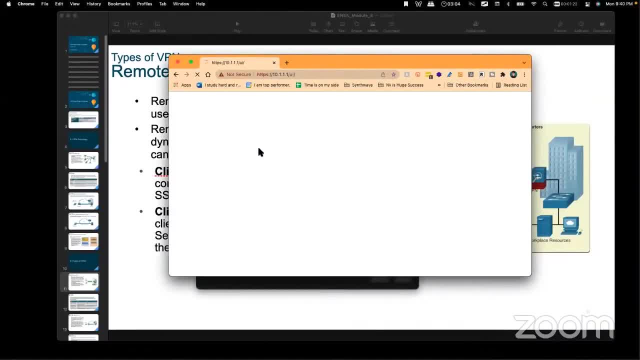 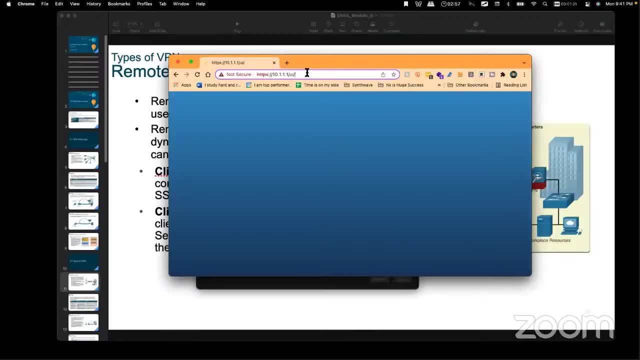 show you. so this is a VMware installed in my office. okay, I am able to access this server, so you can see 10.1.1.1. okay, this is in my office. I'm able to open this VPN, this private IP, from my home. but 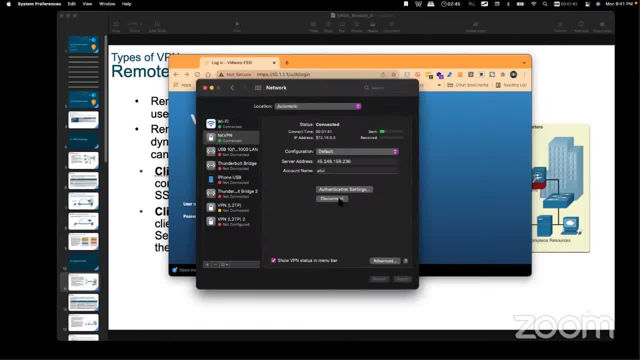 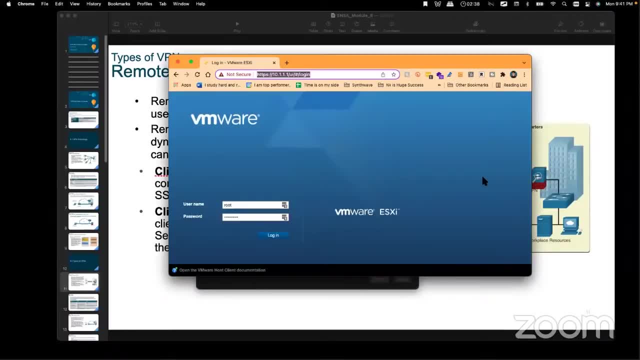 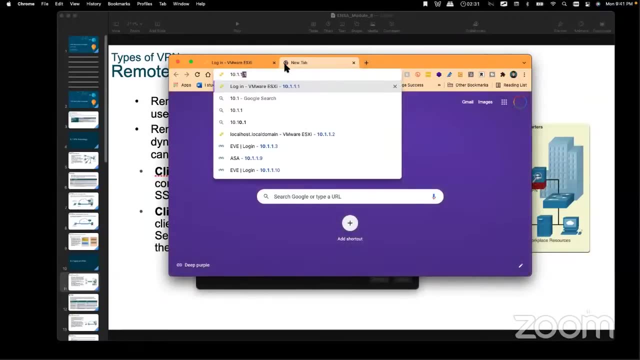 if I disconnect my VPN. let me show you: if I disconnect this VPN for one second, my connection will reset. so hello, I'm audible. yes, sir, okay, now I have disconnected the VPN. if I try to open this IP again. okay, if I try to open this IP. 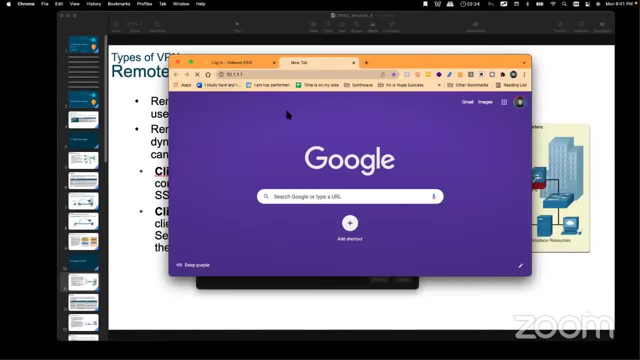 again. let's see what will happen. so now you can see this website is not working. now you got it. why we connect remote site VPNs? yeah, yes, sir. so you are saying it make a tunnel. so is it make a tunnel on it? dedicated IP or single? 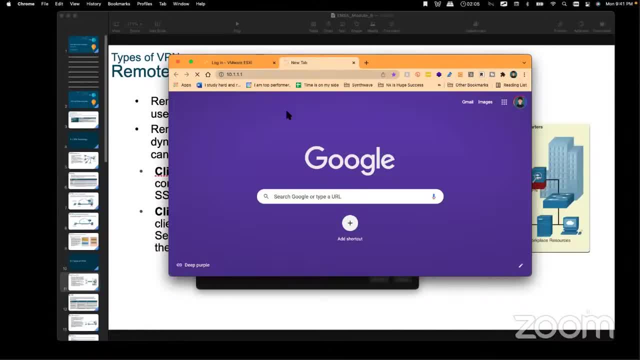 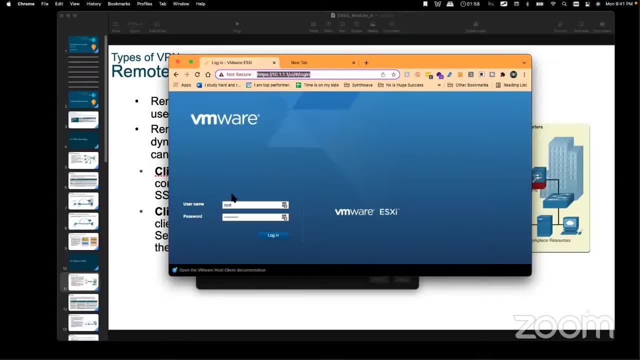 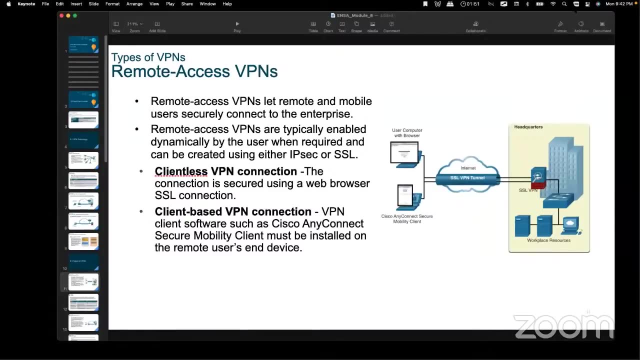 IP. yeah, you need to buy public IP, okay, so you need a public IP, which will be on your router, and then you can create the username and password of your employees and give them username and passwords so they, whenever they are in at their home, they have to. 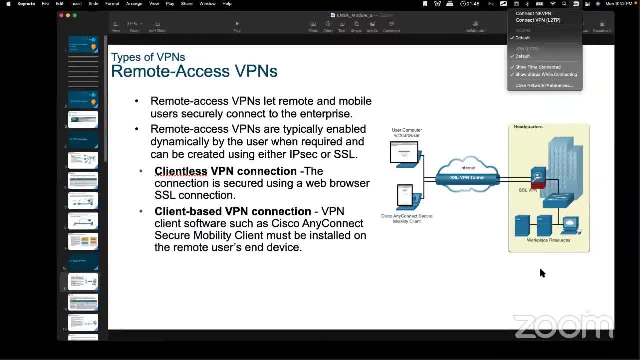 connect to the office VPN and then they are virtually present in my office and they can access the OK. so there are two type of remote access you guys also using daily, which is called client less VPN connection. so whenever you open a website, like maybe a googlecom. 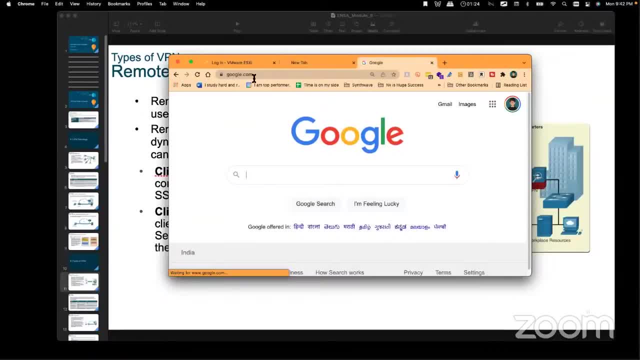 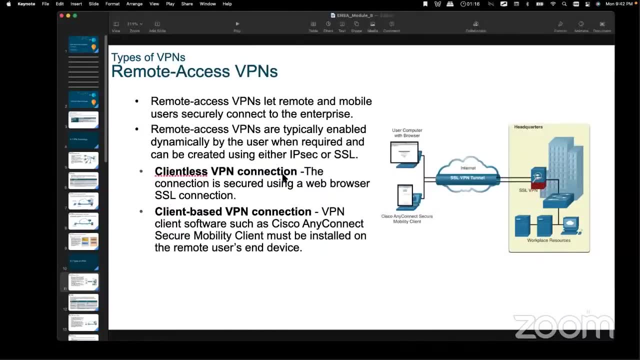 or something like that. so whatever connection you see here over this, so this is called a VPN also, but this type of VPN is called client less VPN connection. OK, we do not need any software. the web browser is helping us to build Bhupender. can you please? 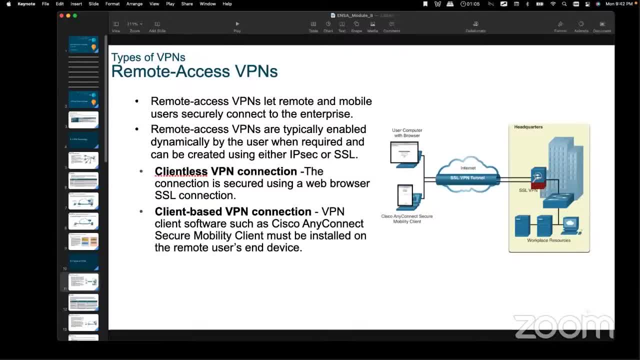 turn off your mic, thank you, OK, so the connection is secured using a web browser. so generally when you use any bank website and all. so that is called client less VPN connection and when you use a software. but in macbook I have not installed any software, but 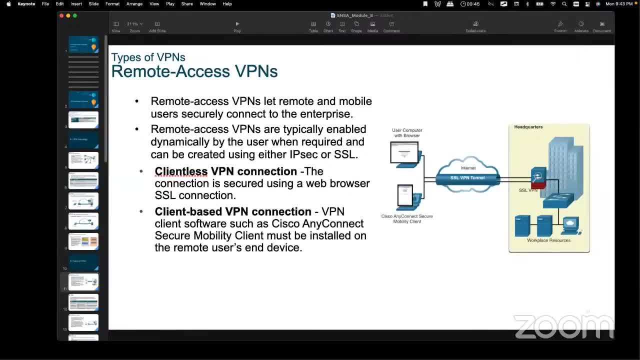 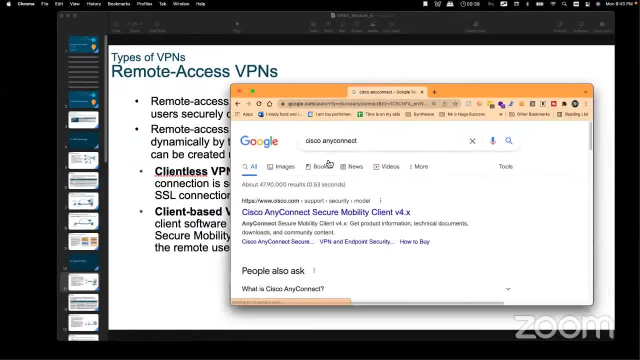 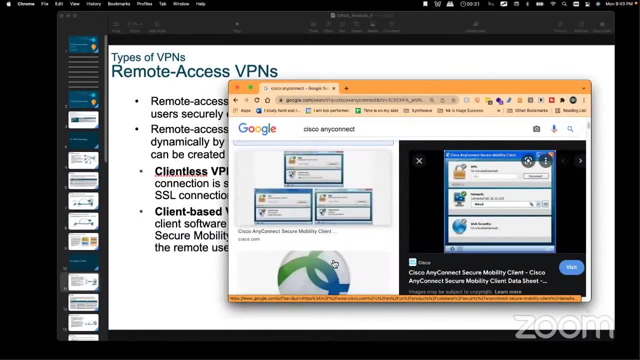 when you use a mobile, what we call windows or something like that. so there is a Cisco software which is also used popularly, which is called Cisco any connect. OK, the software name is Cisco any connect, so you will enter your public IP here and once you enter, 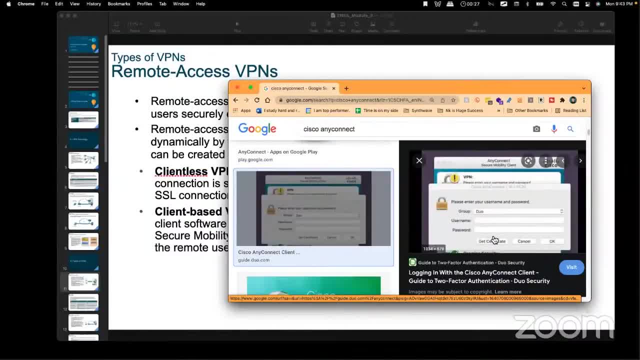 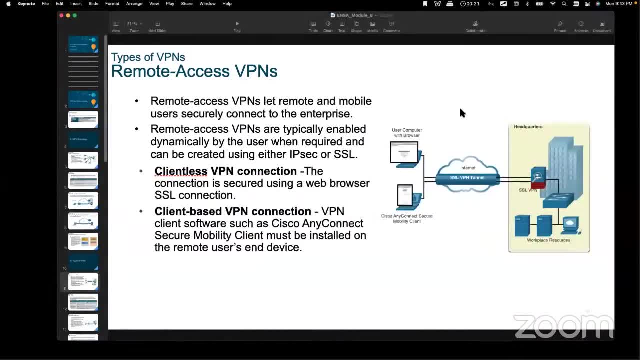 the public IP. it will ask your username and password of your company VPN and then you have to enter and automatically you will be connected to the office. OK, so this is called client based VPN connection, but in macbook I do not require because I can create. I. 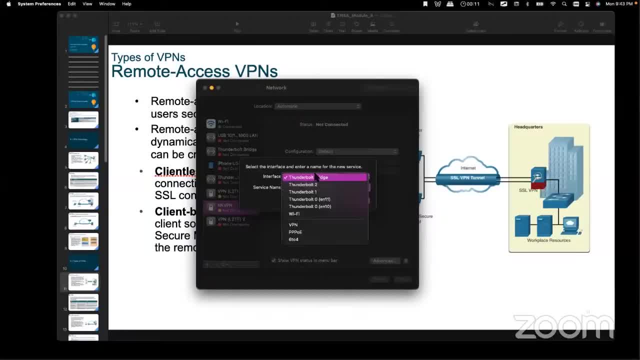 do not need extra software. I can create a VPN from here. I can go: I want to create a VPN like this, and which IP seg, which protocol you are using like IP seg, and then I can enter my username and password, server address and then you will create. 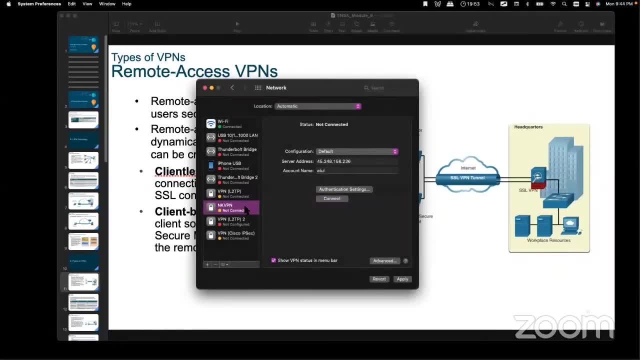 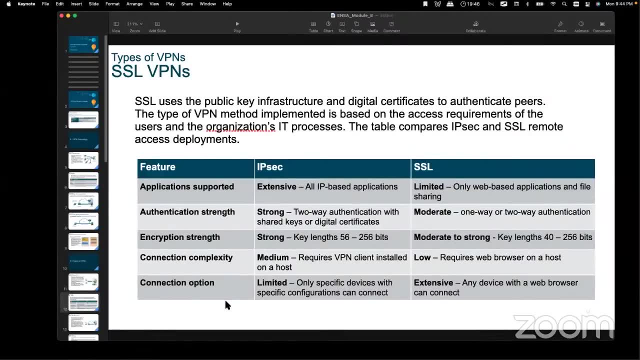 the VPN. just after that, you can connect to the VPN. OK, so this is OK. so, when we talk about this VPN guys, OK, so the IP seg: there is a protocol called IP seg- internet protocol secure- and then there is one protocol which is used over the website. 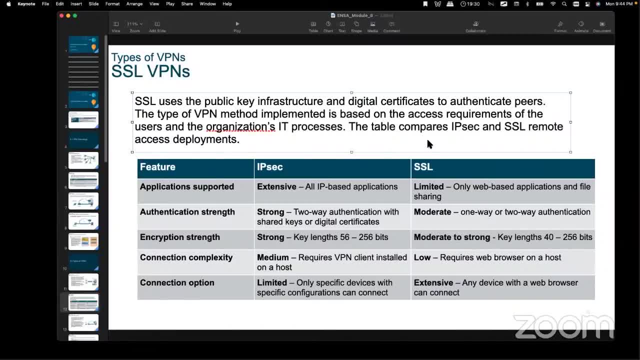 which is called SSL. OK, so the websites are using this mechanism, which is called SSL, secure socket layer. OK, which is limited. only web applications can use this SSL, like websites, and all but IP sec can be used for almost all IP based applications. OK, so this is also. 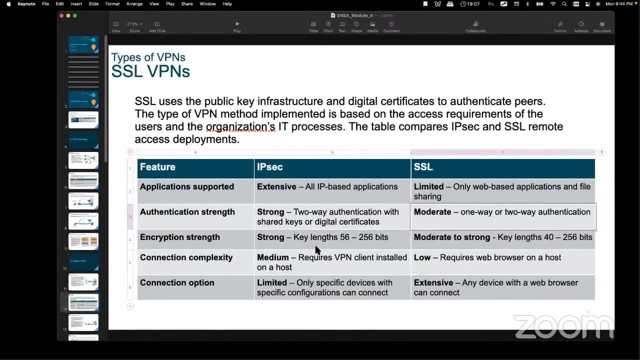 strong, but SSL is not that strong. OK. so when we encrypt the data, the data will be encrypted between 56 to 256 bit. OK means this is a high encryption, so SSL is also providing you 40 to 256, but in IP sec we need to. 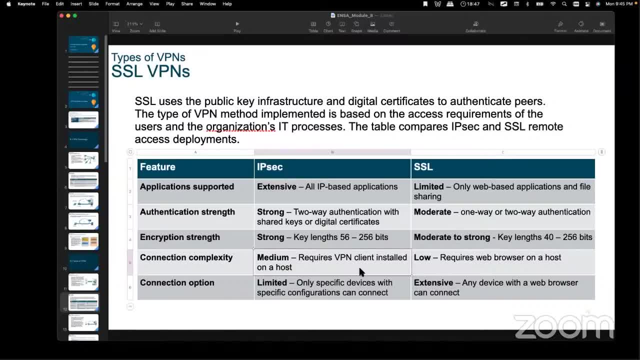 install some softwares or maybe we need to connect, configure this between router to router. OK, and where SSL is Urvish, ask support team here- OK, so requires web browser on a host and so when we go about a site to site VPN. so normally when we 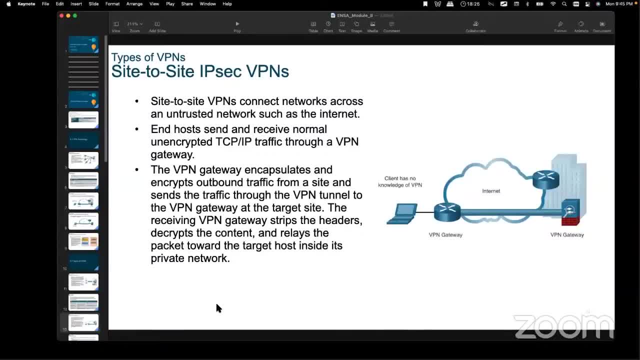 connect the site to site IP sec. OK. so this type of connection we use normally in companies. we use IP sec protocol, internet protocol security. so site to site VPN. again I told you guys, this is when you connect your company router to company router or company firewall to 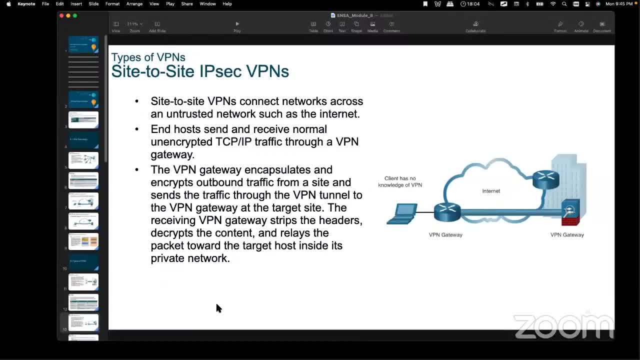 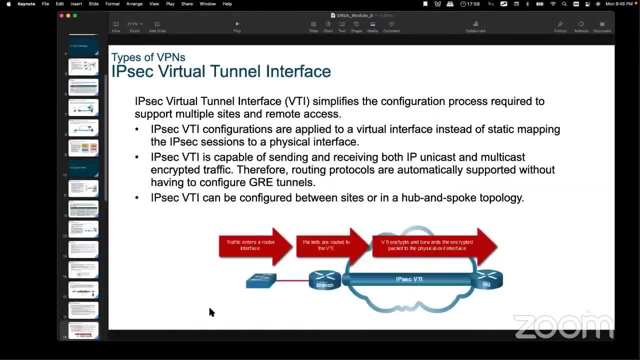 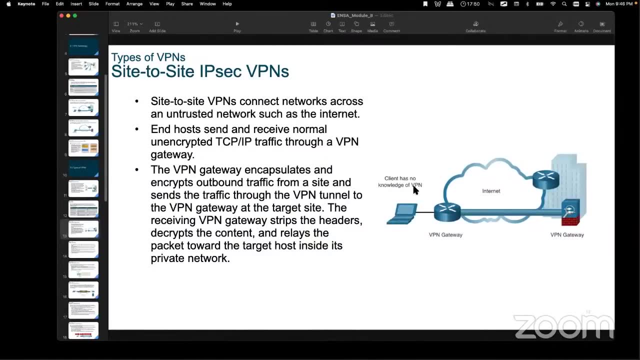 company firewall. that is called site to site VPN. OK, so when we talk about this protocol, which is called now, there are multiple types of protocol, as I told you. first is site to site VPN, so where client does not have any knowledge of VPN. so I will configure. 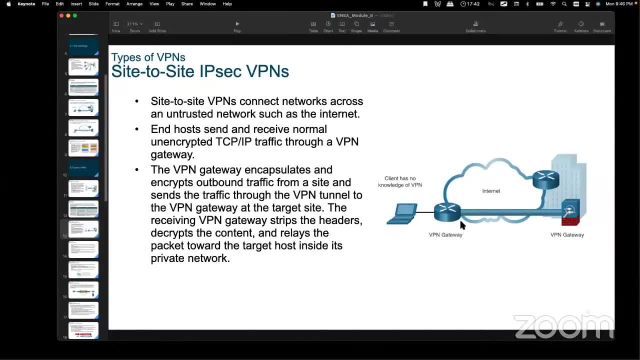 this router and this router. so over the internet, you will configure your site to site VPN. OK, so what will happen? this router is going to encrypt my traffic and forward that traffic to the destination. OK, so this is called site to site IP SEC VPN. and what if? 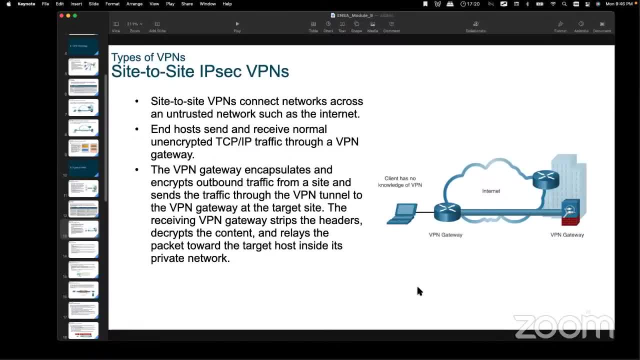 you will open a public IP over this VPN, over the, so these VPNs will be built over the public IP only, so we need two public IPs to configure this. OK, suppose you got IP 200.1.1.1 this side and you got 205.1.1. 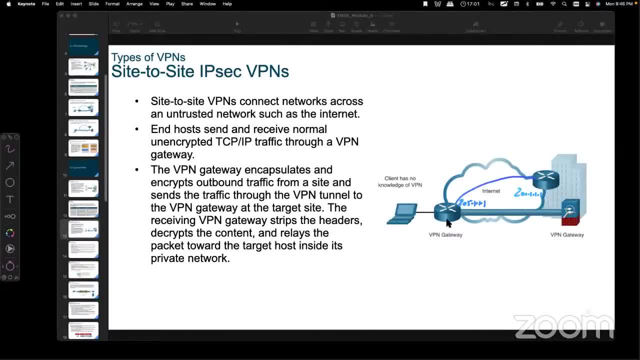 this side. so when you have public IP, then only you can build IP SEC tunnels over the internet, because you are making over the internet, right? so my question is: let's suppose if I'm trying to access internal IP of one branch to another branch, then a router, 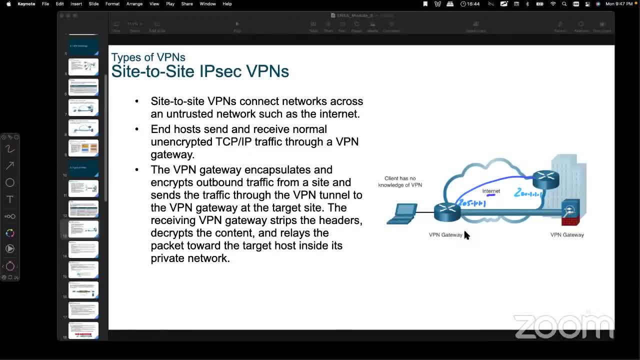 will make a tunnel between two remote locations. yes, yes, correct. so you have a server in Mumbai. suppose this is a server in Mumbai and you are sitting in Delhi, so your routers are already connected with VPN. when you want to share file to Delhi, to Mumbai, you do. 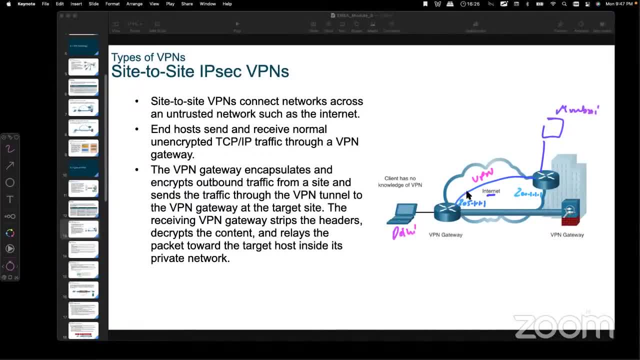 not have to create VPN again and again, so that is automatic process. once you build already, a connection is virtually, connection is already built between two locations. and if, with this VPN, I try to open a public IP, so that is a permission. so now, if your network engineer 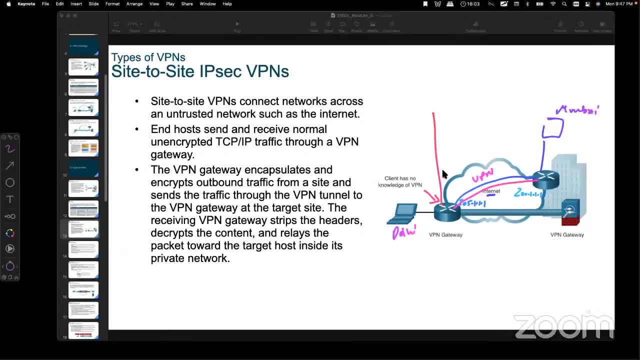 has configured to allow the public access. so when you connect with VPN, there are two methods. so some companies- what they do- suppose you are accessing a very secure server. okay, so you do a not want that user can access the website and user can access the server also. 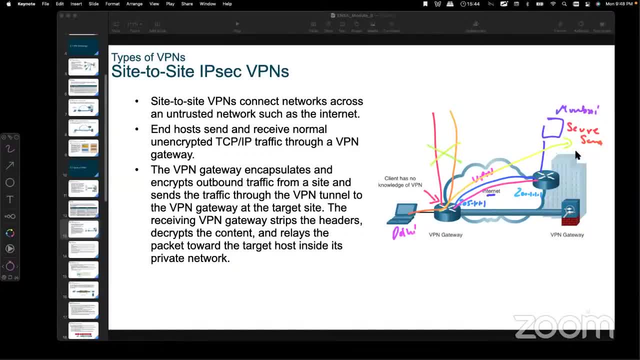 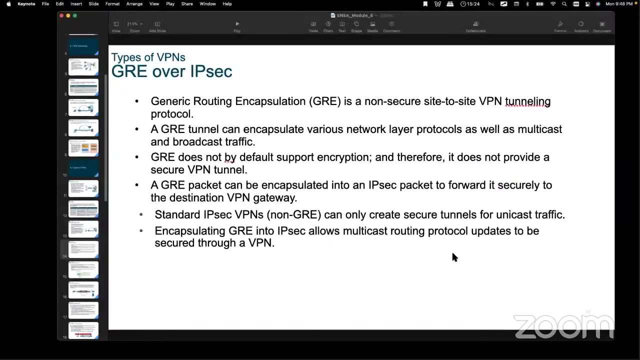 so sometimes they block the internet when you connect with the secure server. but some companies they give you access to access the internet and you can access the server also. totally depends on the company. okay, so now the next technology is also. this is also IP sec, but here. 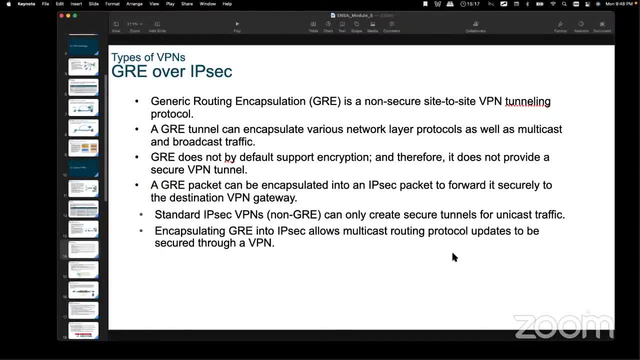 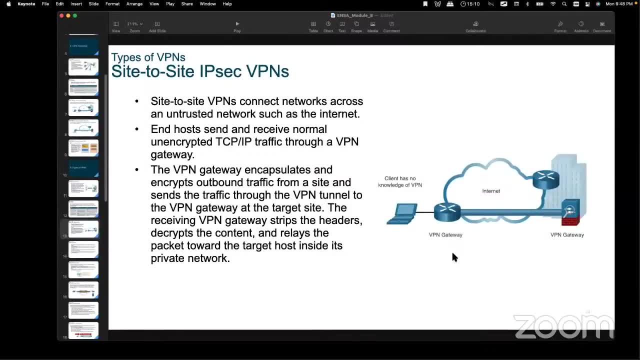 we are using a GRE tunnel. okay, so GRE is a non-secure tunnel. okay, so GRE is also like connecting one office to another, but it will not forward the packet like it is like same like side to side. you will. you need two public IPs. so then, 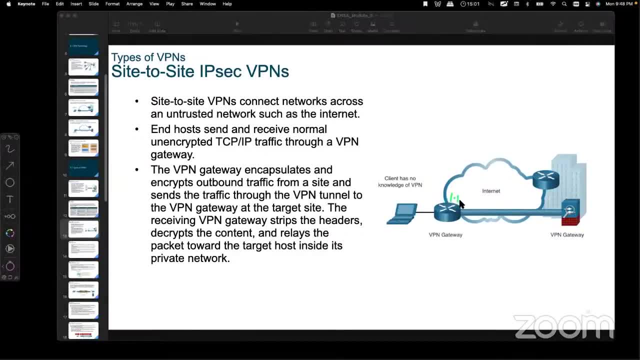 so when you have public IP here, okay, so suppose 1.1.1, 2.1.1.1. okay, so you can connect the GRE tunnel. but this tunnel is not secure. anybody can check what is going inside the packet, so this is a. 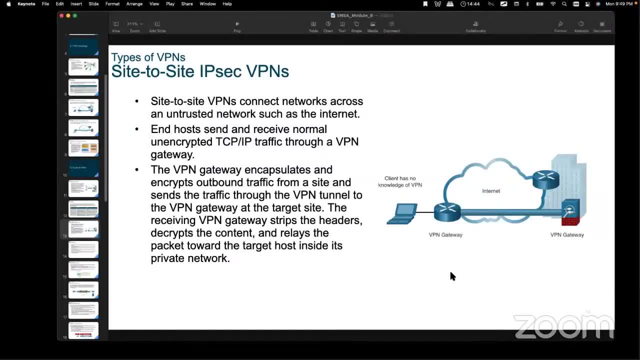 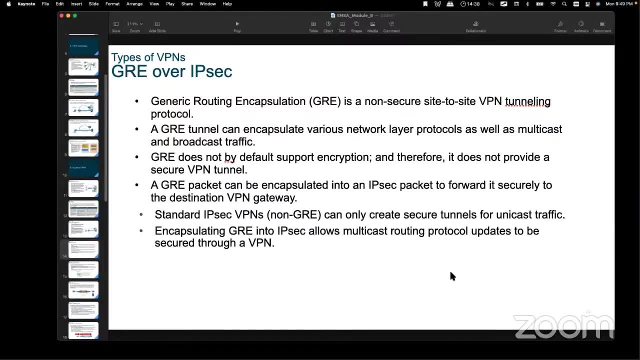 very old technology. GRE, like many people, used earlier GRE, but for security reason, so GRE does not like initially put security. they do not provide encryption. so, GRE, you can read this line: GRE does not, by default, support encryption and therefore it does not provide security, so it will. 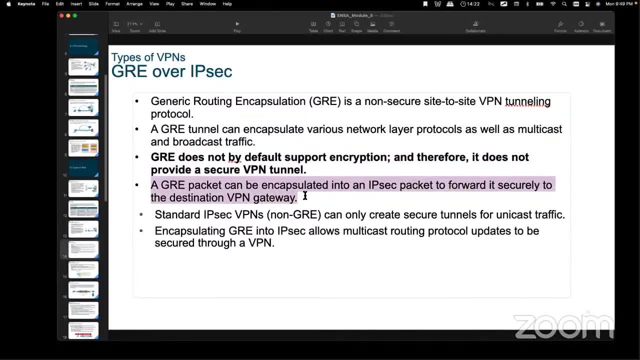 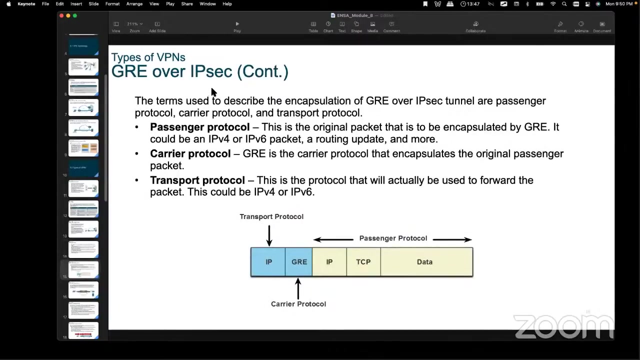 create a more secure tunnel in comparison to the normal GRE. so, if you allow, can I ask you one thing about, if you know, if lab we'll discuss later on, okay. okay so when we use GRE technology guys. okay so when we use GRE over IP sec. 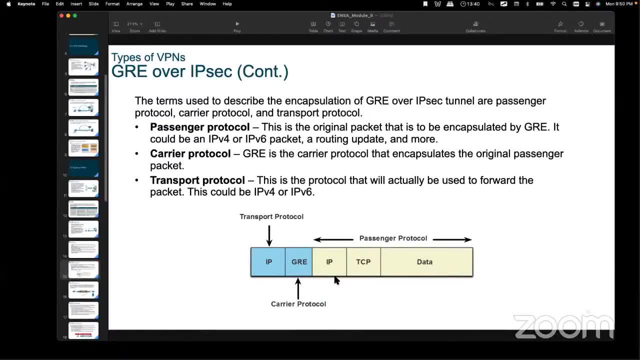 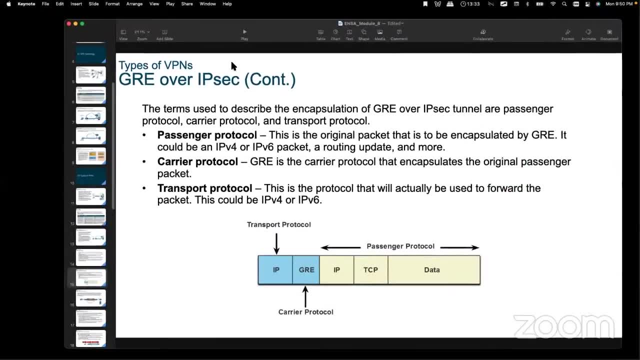 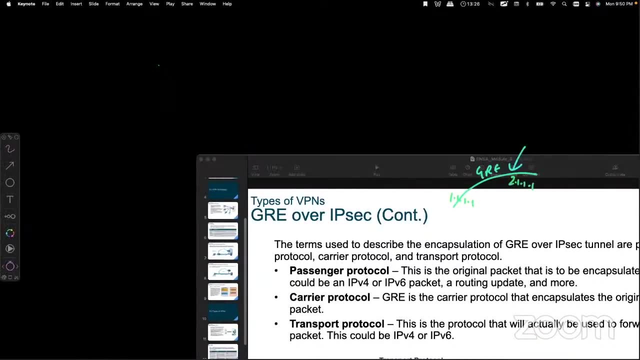 so first you are sending your packet. okay, so you can see GRE is a technology which will add one another IP, okay, so let me tell you. so, GRE, we will try to do that lab. also GRE in CCNA: okay, so many people they learn CCNA from. 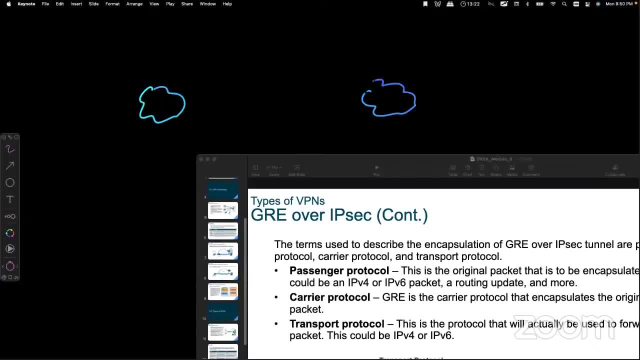 different places they come to know. GRE. never heard about that in CCNA. okay, suppose this is a Delhi router. okay, this is a Mumbai router. so over the internet, what will happen? you will create GRE tunnel. so you got a public IP here. you got a public IP. 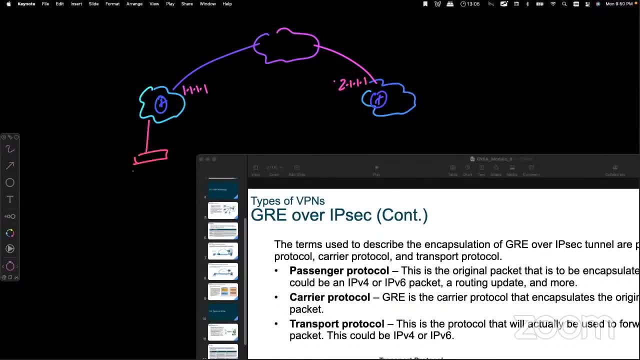 here, okay, but if you want to send your private network, so why? we are using private VPN so that you can communicate your private IP to the another private IP. so now, this is 2.1, this is 1.1, so I told you can we. 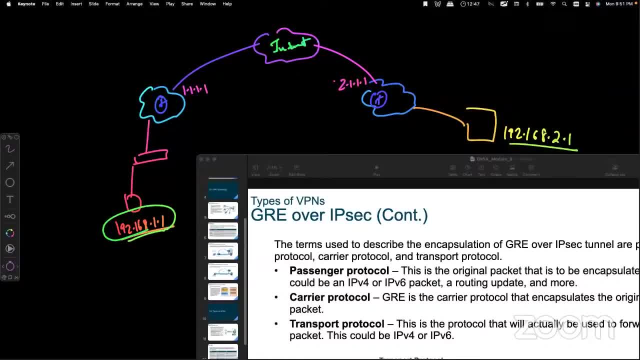 forward my private IP over the internet. yes, no, so what will happen? I am going to forward this IP, so this IP will be hidden inside this packet. okay, so GRE will add another header, which is 1.1.1, but this IP is hidden. so how? 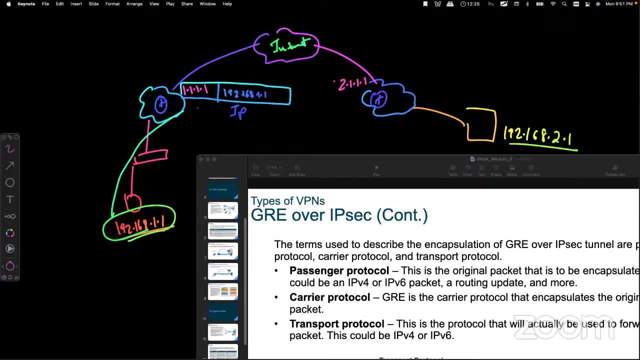 many IP headers we have now. this is one IP header. so when we use GRE technology, generic routing encapsulation, it will actually add one another new IP header which will put the public IP. so now we will forward the packet over the internet and internet will see that. 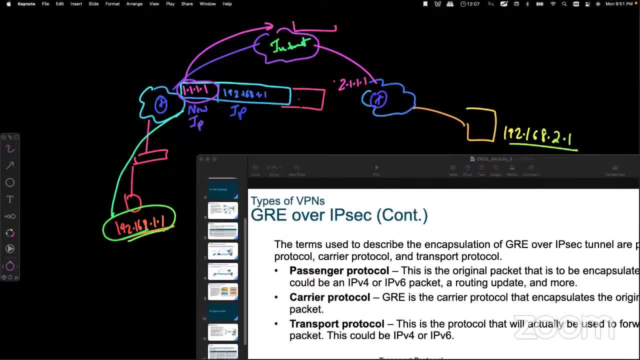 traffic is going from 1.1.1 to 2.1.1.1, but internally they are 190 to 160 to 1.1 and going where 90 to 160 to 2.1. so in one packet you 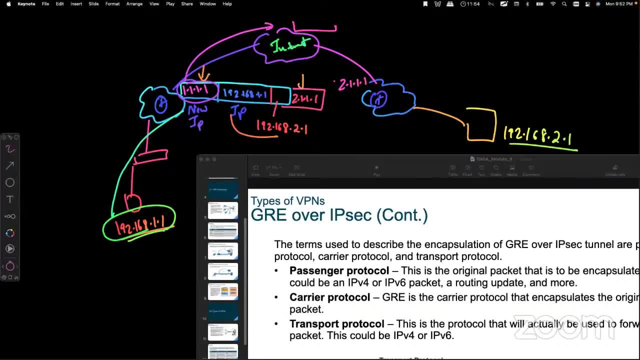 have private IPs and the public IPs both. but when the internet will come to know? traffic is going from 1.1.1 to 2.1.1. but inside that packet, what is there? the traffic is going from 190 to 160 to. 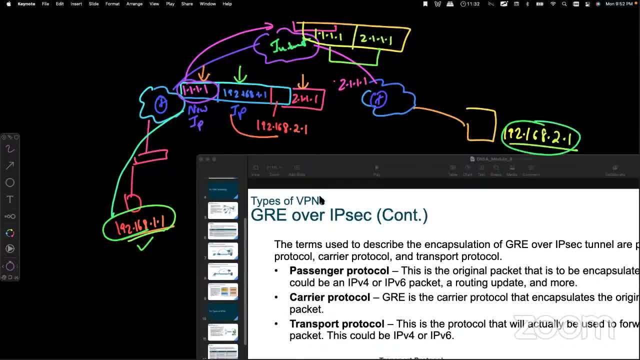 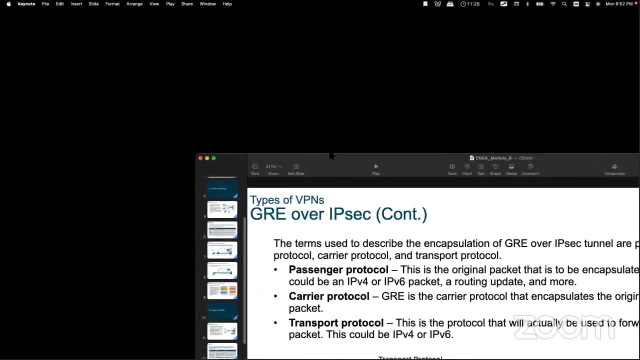 1.1 to 190 to 160 to 2.1, so this concept is called GIP. so now you can use IPsec and GRE, which can actually help you or the companies to protect your company network, but if you do not use IPsec, 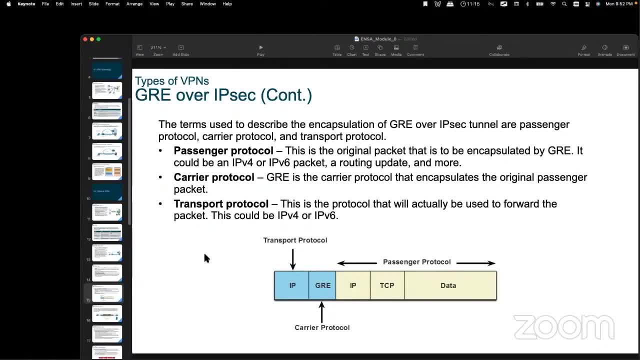 with GRE, so the connection will not be secure. so GRE basically encapsulate the original header. it will add extra information so you can see this is IP, so you can see here the normal where we are going. this is my actual original data that I want to go. 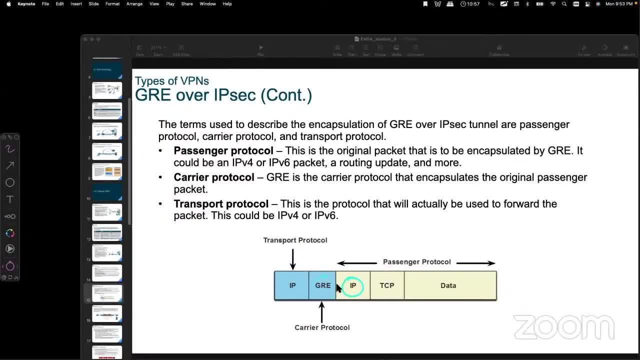 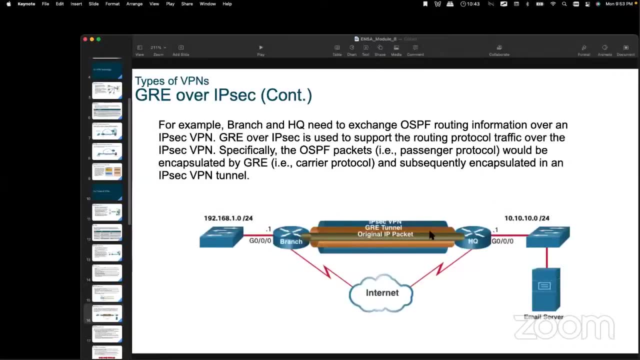 from private IP to private and this GRE header. so this is GRE, which is the protocol which is forwarding your information. so GRE is adding one extra, another IP, so that over the internet you will use the public IPs. so that's called GRE, so you can see here. 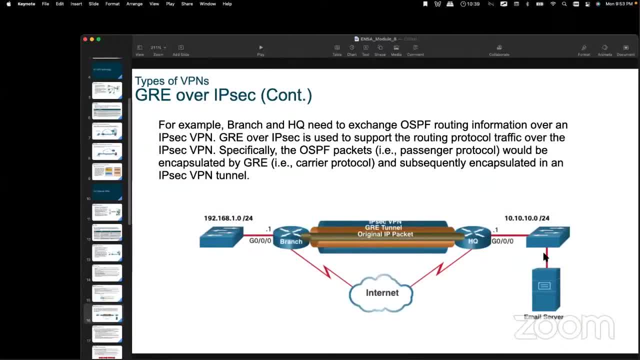 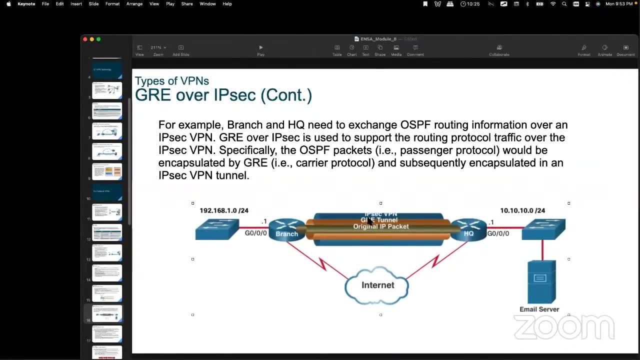 so this is happening: 192.168.1.0 is going to the email private server, but original IP packet is this and which is actually GRE tunnel or IPSec tunnel, is actually sending that original packet inside the tunnel. can you see that image, guys? yes, 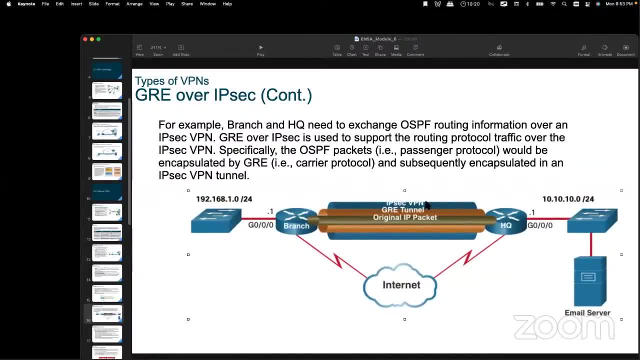 so this is the big pipe which is called IPSec, big water pipe, let's assume IPSec. okay, there is a pipe which is IPSec VPN and inside that there is another pipe which is GRE tunnel and then another pipe which is called original IP packet. so 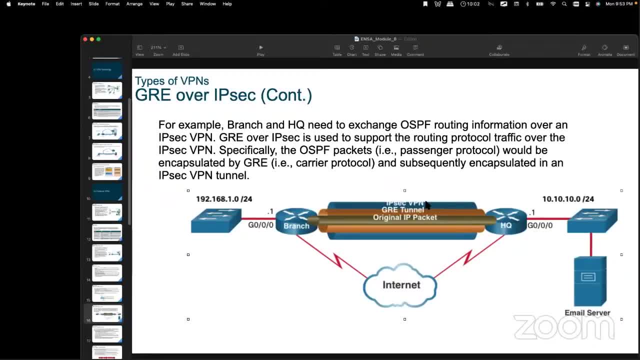 who is protecting my data, which is the bigger pipe? IPSec, which is securing my tunnel. yes, yes, hello, yes, okay, and IPSec is using which method? GRE, and inside GRE, which we are forwarding, we are forwarding the original IP packet, okay, so this is all industry and 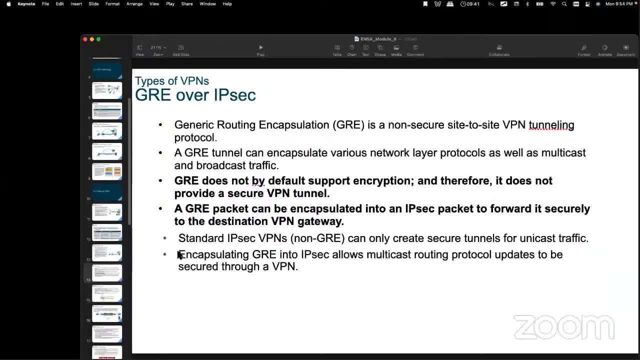 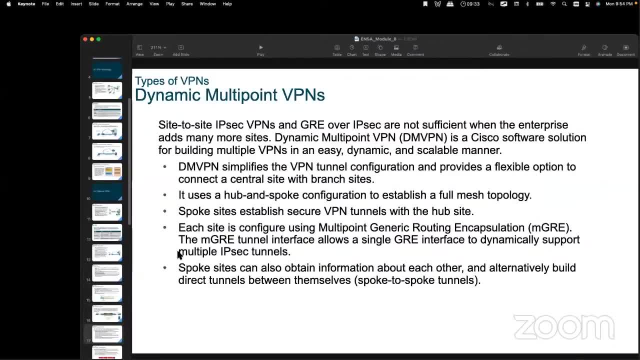 so another type of VPN, so two VPNs we have discussed side to side IPSec VPN- okay, and GRE over IPSec- okay. and the third is a very popular nowadays which is called a DEM VPN. so this is called a dynamic multipoint VPN- okay, which is. 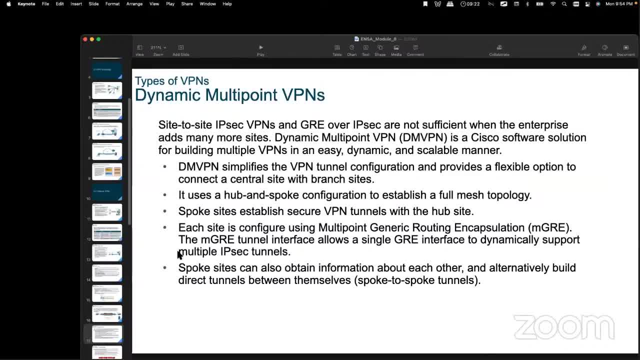 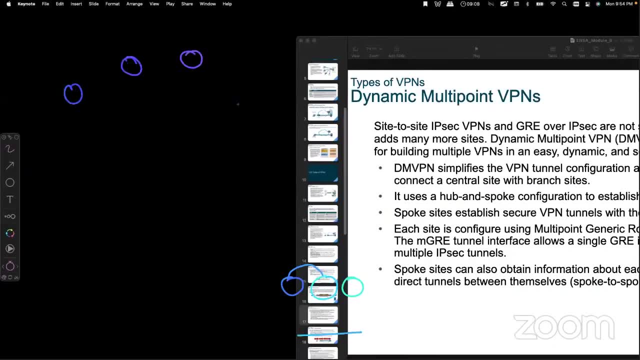 also used, and this is a concept of multi GRE, okay, multipoint GRE. so let me show you what is this DM, why we use a DM VPN, okay, so this is suppose you have 10 branches, guys. okay, you have 10 office. okay, over the internet, if 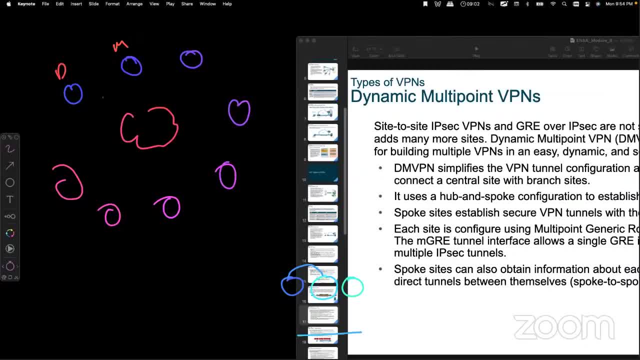 you connect to a 10 office from Delhi to Mumbai. you have to build a tunnel between this if you want to forward traffic from Delhi to this. so every router on every router. suppose this Delhi router wants to go to this Mumbai? okay, or this Mumbai router wants. 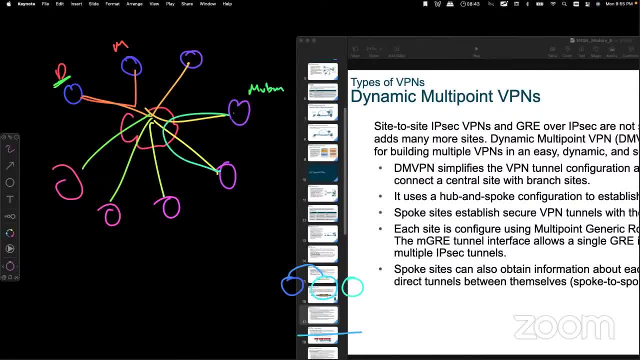 to go to this router. so they need VPN tunnel. like this, every router will have tunnel with every router. yes, we will have a lot of tunnels. suppose you have 10, so 10 minus 1, you need 9 VPN tunnels on every router. yes or no? 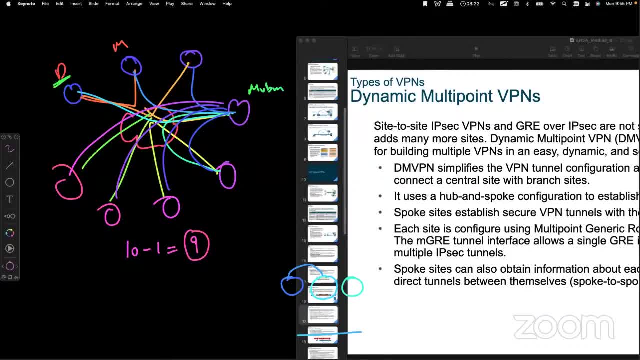 yes, okay, normally if you want to connect all the offices, every router, if you want this router can communicate with every branch office, then on every router you might have to configure 9 tunnels, but this DM VPN technology actually eliminating also when you have a 10 branch. 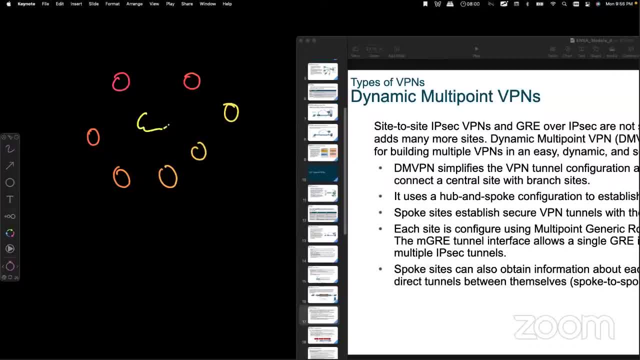 okay when you have a 10 branch office. so over the internet, just one tunnel is required on every router and because this is called dynamic multi-point VPN, this is called multi-point GRE on, with one VPN tunnel only, we can go to any of the branch, okay. 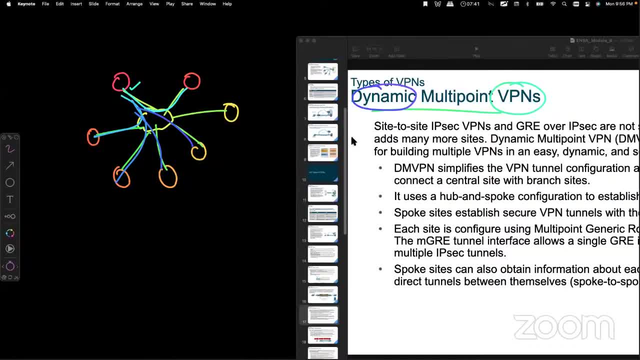 so it means the DM VPN is very good in terms of VPN tunnel and we buy with one. we can access all my branches. so tell me, which will you prefer? if you have 10 branches, you will go with the normal tunnels or you will use DM VPN. 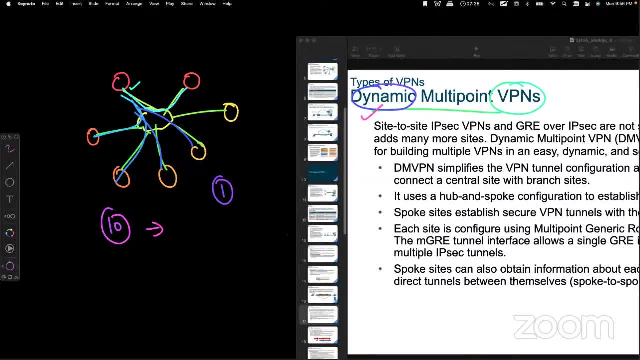 okay, just to inform you, Apple kind of companies are using dynamic multi-point VPNs to connect their offices. okay, so they have 200 plus offices all over the world, so most of the branches or connections they have connected with the service provider VPN. I told you with. 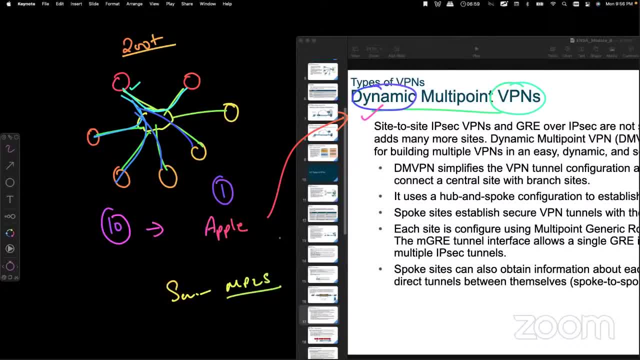 MPLS, but some third party sites or the customer sites or the retail offices they have connected with the DM VPN. okay, Apple store, hello, yes, okay, so suppose they have retail offices, they are selling the laptops and all. so they do not want high, secure, reliability in the? 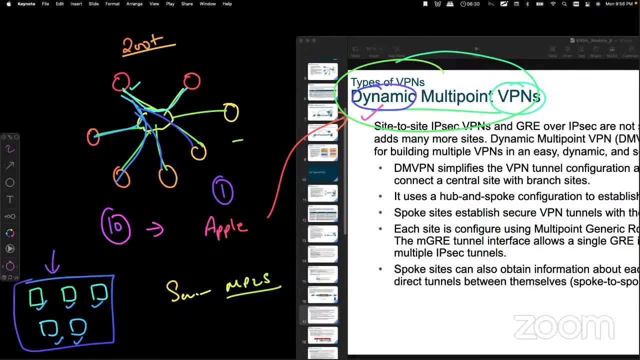 retail offices. yes, you want reliability. you want high speed in Apple actual offices. so, for third parties kind of sites, what you will do- because I do not want reliability in all over the internet- I will connect all those offices with the DM VPN. clear everyone. yes, yes, okay. 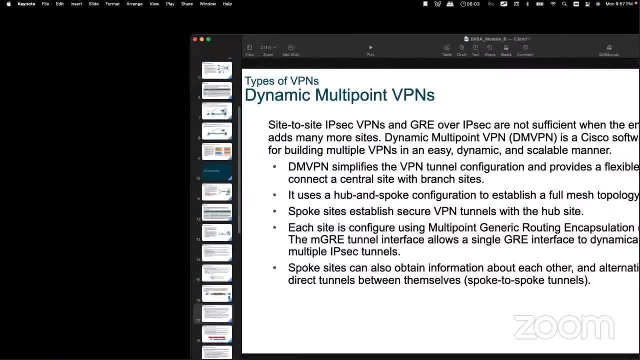 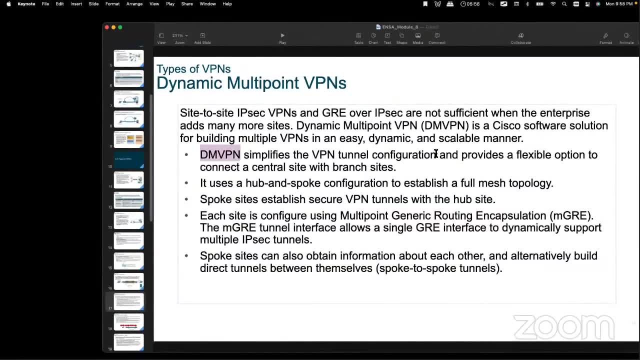 just you need idea. this is the objective of this class. okay, so DM VPN is a Cisco software solution. so DM VPN will simplify the VPN tunnel configuration. that you will not create a lot of tunnel, just you need to build that. maybe one tunnel will help you to. 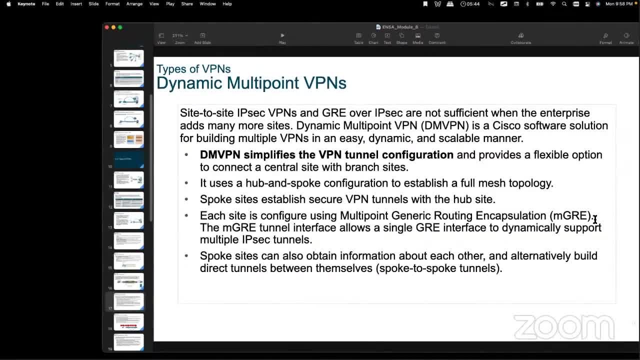 connect all over the offices. so DM VPN works on? which technology? multi GRE, the GRE we discussed. okay, it is working on this MGRE, which is called multi point generic routing encapsulation. okay, so this is the DM VPN. and when we talk about IP, SEC, virtual interface, 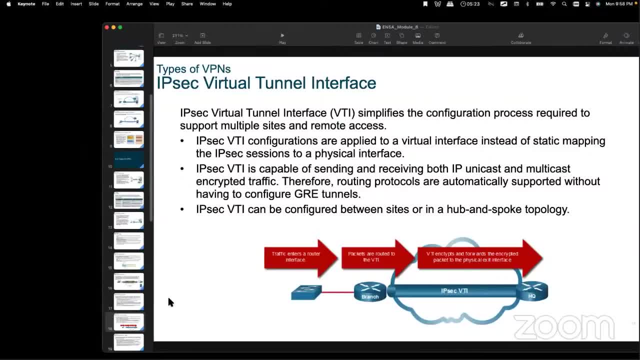 this is also similar to IP SEC. so IP SEC virtual tunnel interface simplifies the configuration and we are going to connect one office to another office. okay, that is like we are building a tunnel or virtual tunnel interface between one to one location. it is similar to like: 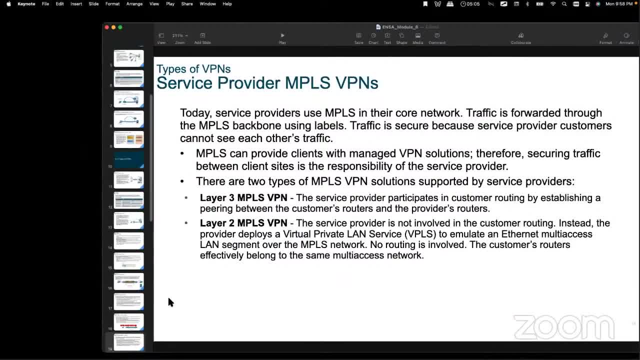 that only okay. but when we talk about service provider MPLS, VPN, these are the two VPN tunnels which is provided by service provider VPN or service provider MPLS. so MPLS is basically a technology where we are going to forward the information and we are going to 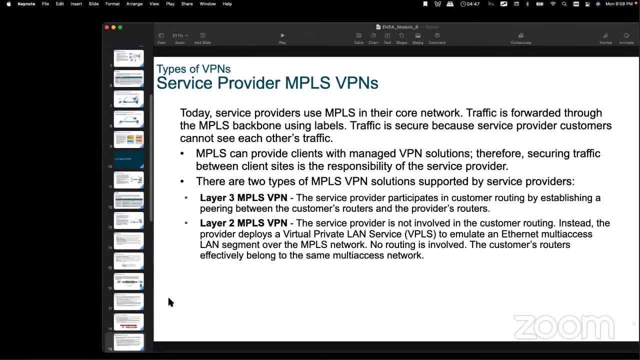 learn how ISP configure MPLS. okay, how ISP configure MPLS tunnels. so there are two types of. there are many types of VPNs. okay, let me tell you how many I know. okay, this is like there is a multicast VPN which is called MVPN, EVPN. 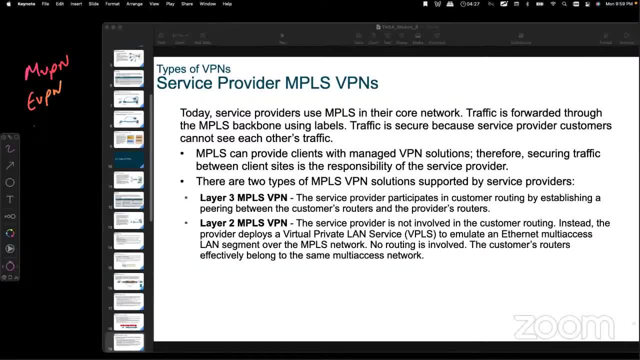 okay, okay, there is a. already I told you VPLS technology: L2 VPN- okay. L3 VPN- okay. so there are other technologies also. so these are, like all service provider VPNs: okay, the VPNs we discussed about the IP stack, DM VPN- okay, normal IP. 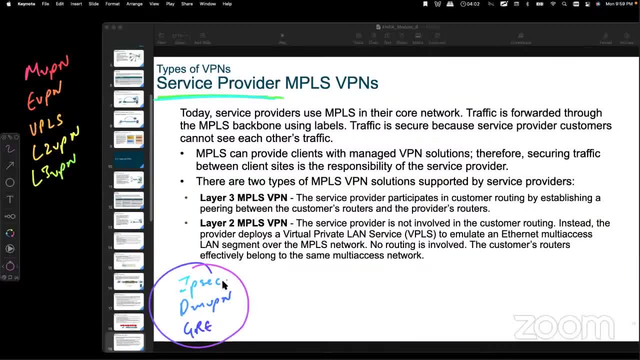 stack or GRE tunnel. so these all are enterprise VPNs and all these VPNs are all these VPNs are service provider VPNs. okay, so when you learn these technologies, it means you are going to work either for service provider, or either you work for Cisco, Juniper. these companies. okay, my 10-12 years experience into service provider- and I worked with Juniper, so Juniper networks actually meant what they do. they have a tag team, okay, technical assistance center, so what we do? so when? so when a big ISP, maybe ATL, ATL. 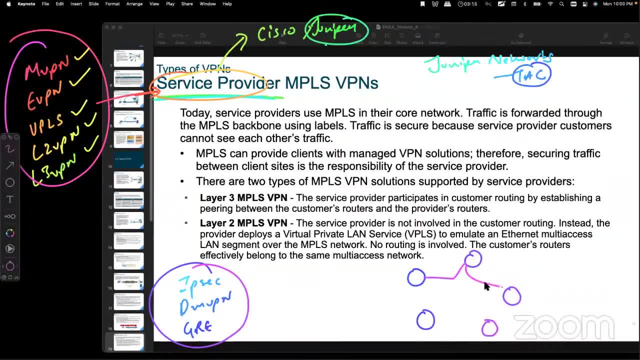 is connecting customer offices and ATL is connected connecting a lot of VPNs. so they are using Juniper or Cisco kind of devices. so now, if ATL is getting problem because we are using Juniper routers, if they get problem where they will ask the Juniper tag. 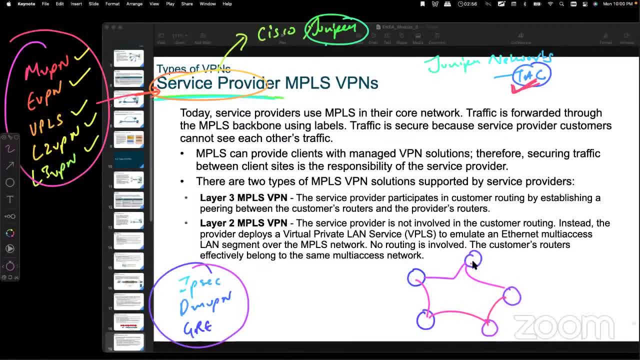 team. yes, so if they get all, if ATL, ISP get a trouble, if ISP get a trouble to connect their like routers with VPN or MPLS technology, so maybe there is some issue going on. so who will fix this issue? the company right, the OEM original equipment manufacturer? 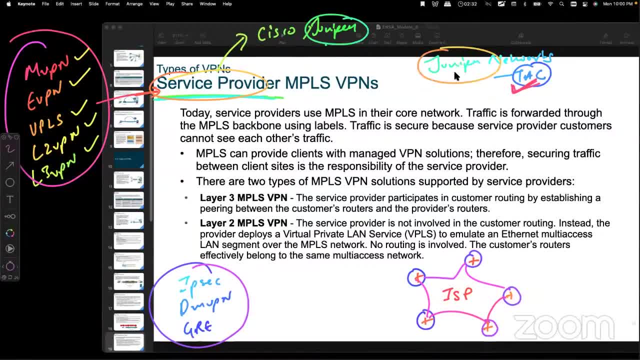 yes, the router company, right. so there also people with tag profiles. they need these type of knowledge: L2 VPN, L3 VPN or this stuff. so by learning this technology you do not get job into only in service provider, you can directly apply to these companies like Cisco. 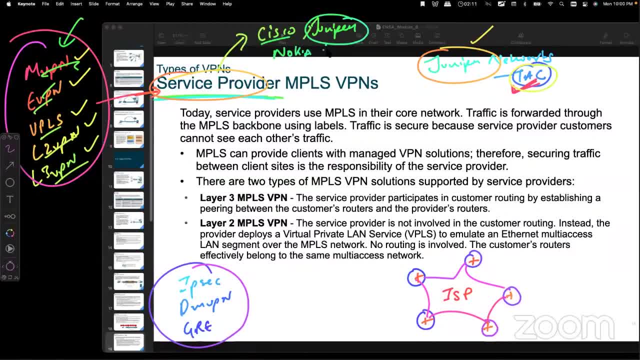 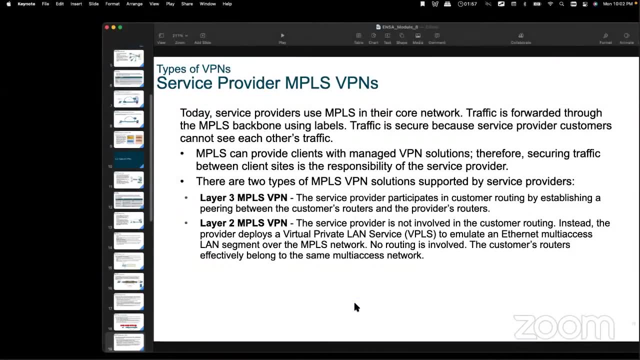 Juniper, Nokia, Alcatel. okay, so the Huawei, Sienna, so these all companies? also hire those engineers who have service provider knowledge. okay, got it. but trust me, I'm trying to give my best so that you will get an idea in a CCNA batch. nobody. 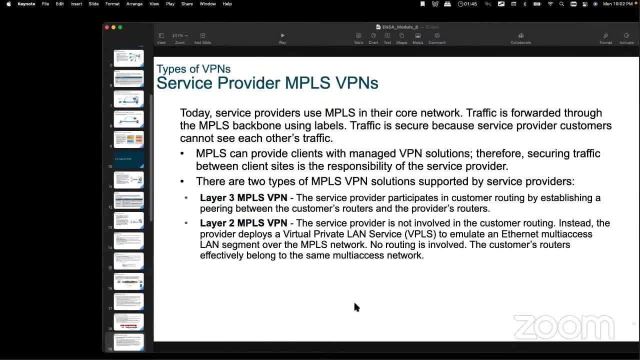 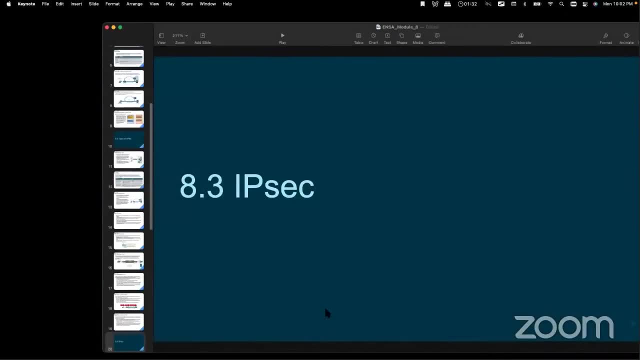 what you know as a CCNA guy, I'm sure, or those guys who are watching in YouTube, you many people. they do not understand what is going on. okay, so I hope you got information about the real industry today. okay, so let's discuss about IPSec. I'm 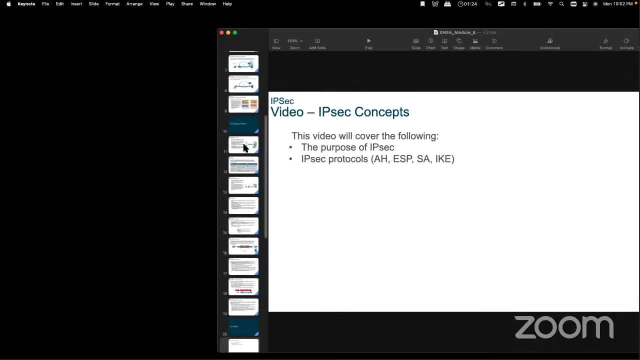 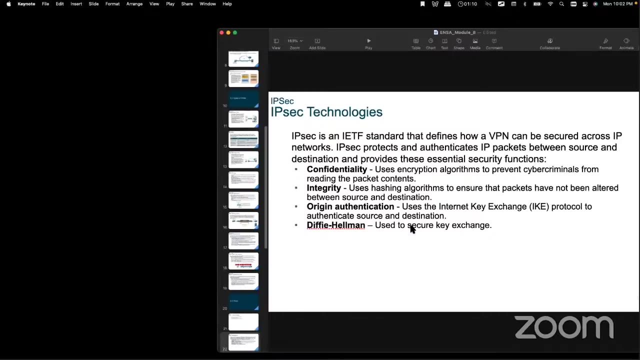 giving you little bit overview of IPSec also. so now we understand. IPSec is basically to connect my office with another office over internet with secure method and which is called IPSec. so when we talk about IPSec, IPSec is basically internet protocol security and which. 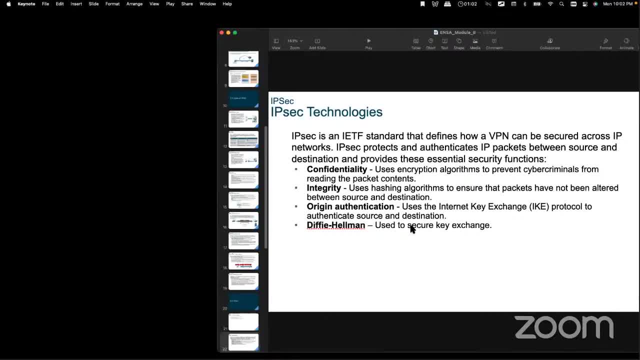 gives me four things. first is confidentiality. okay, confidentiality means no cyber criminals can check what is going in inside my packet. okay, that we are going to confidentiality means we are going to protect our data with the cyber criminals, hackers and all so that I'm going to encrypt. 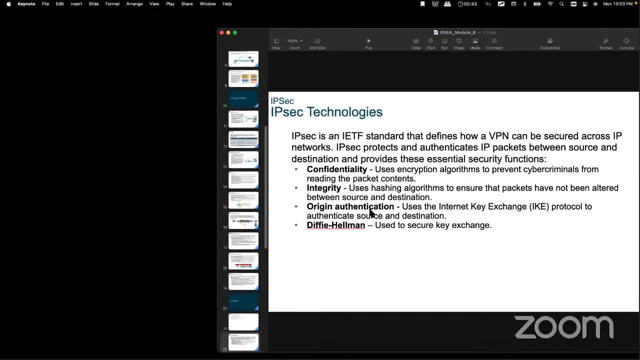 the data. okay, that is called confidentiality and that is provided by IPSec internet protocol secure. so the second thing IPSec provides if somebody ask an interview. so this is how you are going to say: IPSec internet protocol security is a protocol to secure the connection and 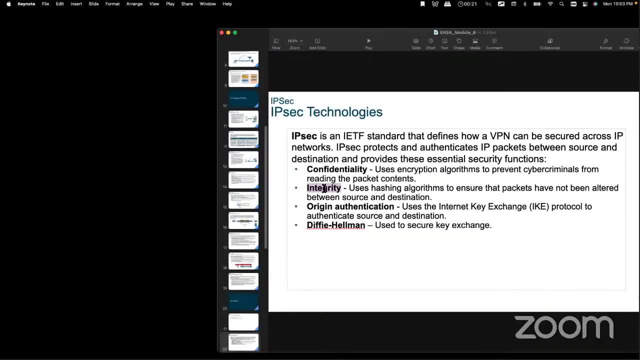 it provides confidentiality, that we are going to encrypt the data. second is integrity: that nobody can check or change the packet. here we are going. nobody can read the packet. let me write the simple language: read the packet. okay. nobody can read the packet. what is going inside? 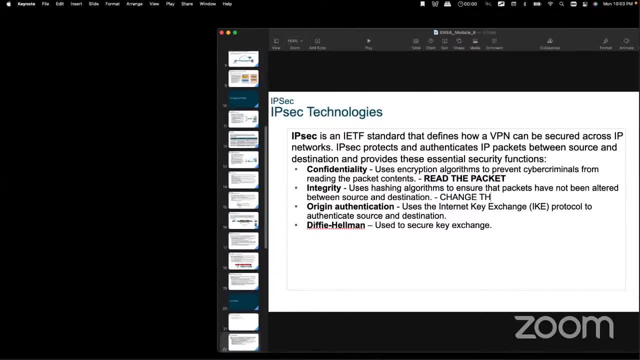 the packet. other, nobody can change the packet, nobody can change the information inside the packet which is called change the packet means we are going to use some hash algorithms so that nobody can actually alter the information, so okay. and third is origin authentication. that we are going to 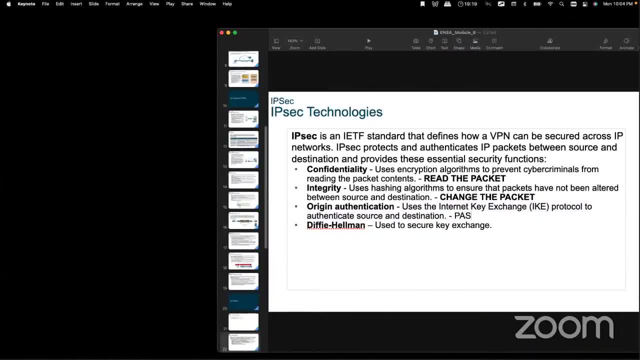 use some passwords. in a very simple language, we are going to use some passwords. if I set a password on one side- suppose I have a delhi branch- okay, if I am going to set a password here, that my password is cisco? okay, do not give this. 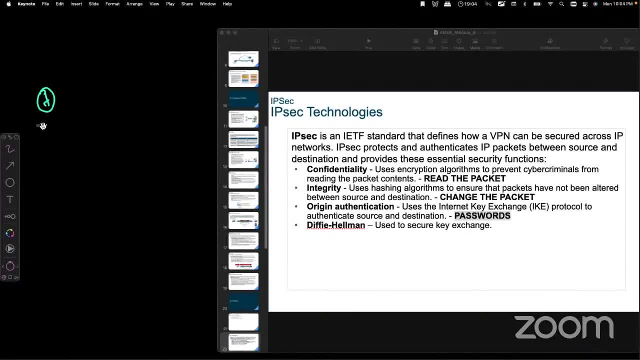 password, which is very weak password. maybe if I give nwkings 123, okay, nwkings 0113, hash 1, so if this is my password, that on the another side also I have to give one password so that nobody, if any attacker is there. 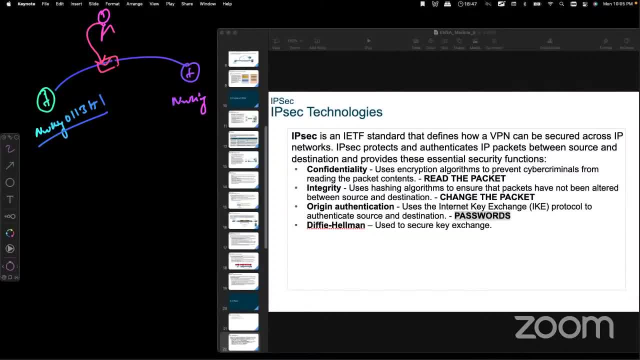 somebody try to steal the information so they to read this packet, to change this packet, so they cannot connect to my VPN tunnel until, unless they do not need, they do not have the password. so IPSec is also giving you authentication if you want to connect the router. 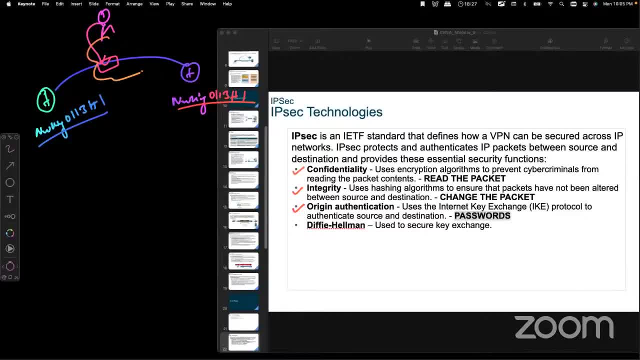 with another router or like one branch to another over the internet. so we have confidentiality. nobody can read the packet, nobody have the password, which is actually given by internet key exchange protocol, and there is another method also that these passwords we are not going to share to each. 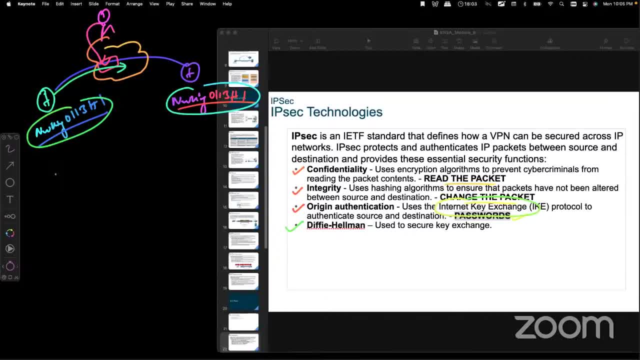 other, we will come up with the one shared secret password. there is algorithm called Daffy Helmet. okay, so this is another trick. this is a very secure method. so, like they will do some math, okay, I'm just giving an idea. so with the Daffy, 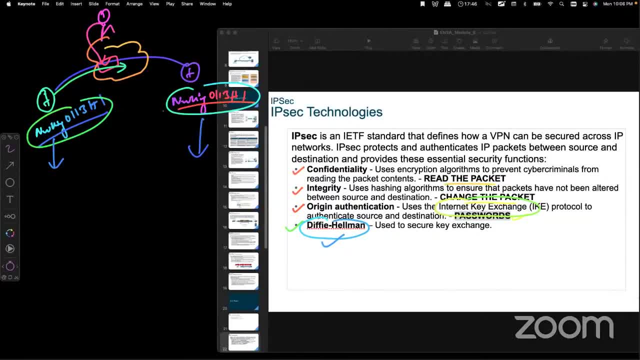 Helmet, they are going to do some math, so they will agree on one password. okay, suppose this is. this is the public secret? okay, but this is not the actual password. so router will calculate some math and they have their actual password. is suppose this 331 hash? okay? 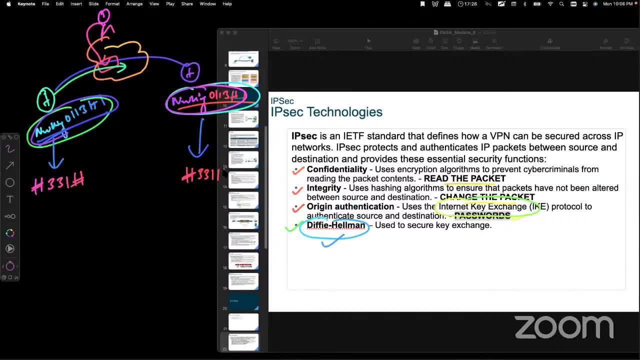 this is the actual password. so with Daffy Helmet algorithm, with this Daffy Helmet technique, we will not share the exactly password. we will share the wrong or some kind of password, public secrets. but if some, even hacker, come to know this password, no, they cannot. 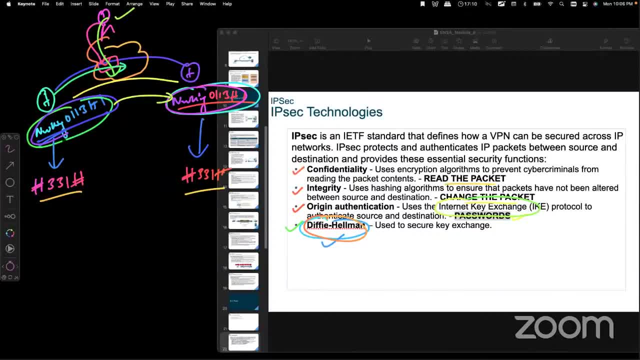 get the data because with this they have some internal math with this Daffy Helmet, but actual password they calculate inside their devices only. they do not share the private secret. this is called private secret. okay, so they randomly generate this private secret with this public secret. so 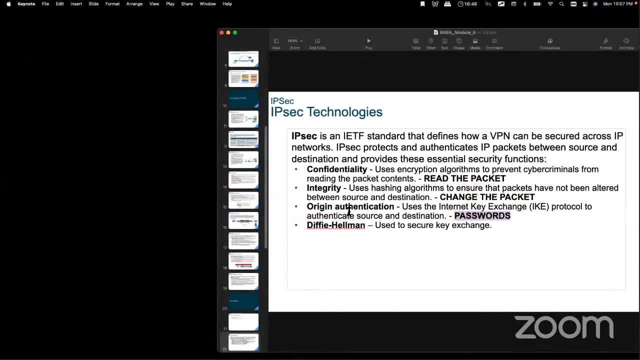 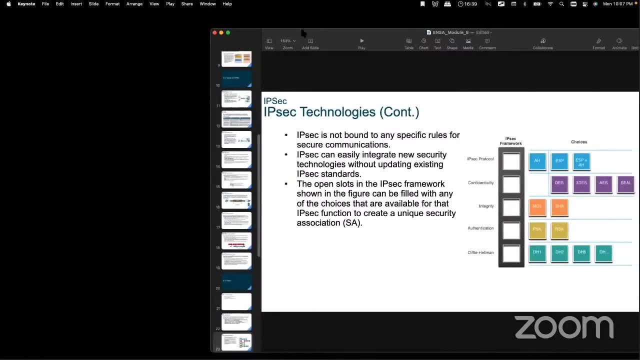 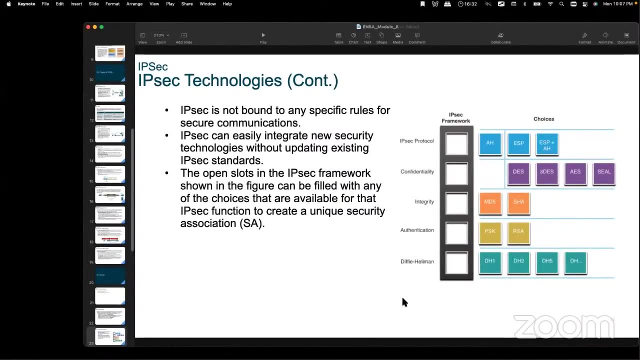 public secret. they exchanged, okay. so that's the basic concept about this, so let's understand. so now, if I talk about IPSec guys, IPSec is not a protocol, it's basically a framework, okay, like if you go to a shopping mall and suppose you want to, 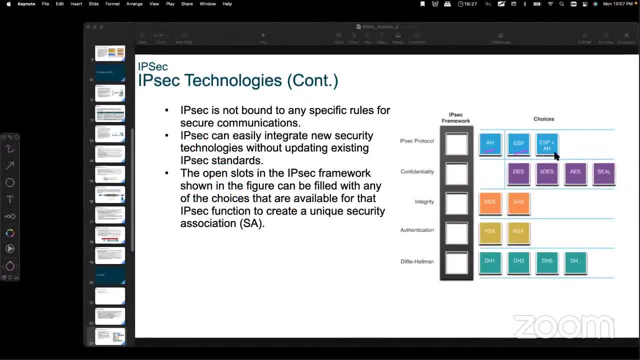 buy a milk, okay, there is another different, different brands available now. if you want to buy the nuts, the different, different brands available. if you want to buy some pizza sauce, maybe different brands available. so you have different, different packages. now you can choose this. now you can choose. 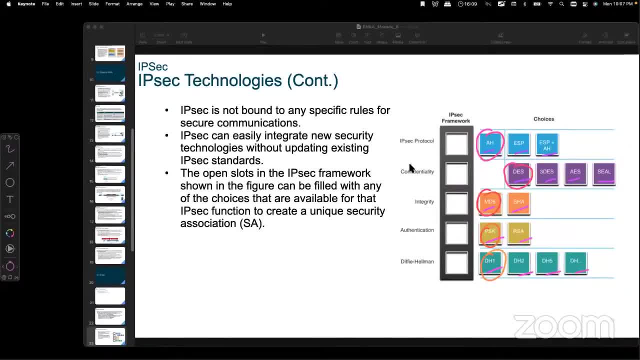 this, this and this and this. so this is how we are going to use confidentiality. okay, with IPSec protocol. so first you have to choose which type of like which protocol you want to forward the data. so this is called authentication header and this is called encapsulation. 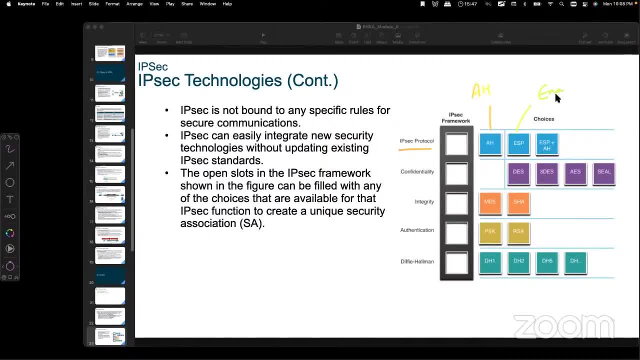 security payload, encapsulating security payload. this is highly secure. if I you want to understand simple way, so this ESP, you can check on google also about the full form. so if you send the data with ESP, the data will be also encrypted. so suppose you are sending a. 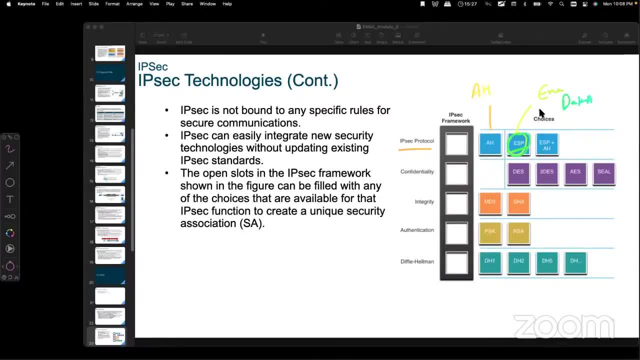 data. suppose you are sending a google file or any pdf file, so the actual data will also be encrypted. when you will send with ESP encapsulating security payload, but when you send with AH, it will only secure the headers, which is called authentication header. we will only secure. 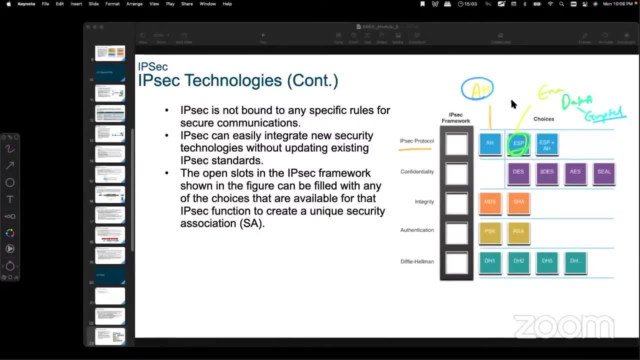 the information. ok, but we will not encrypt the data. but normally, if you talk about which is more popular, the ESP is more popular. so now, with confidentiality, these are the security method. ok, so every confidentiality means encrypt the data. ok, ESP is using and we are going to. 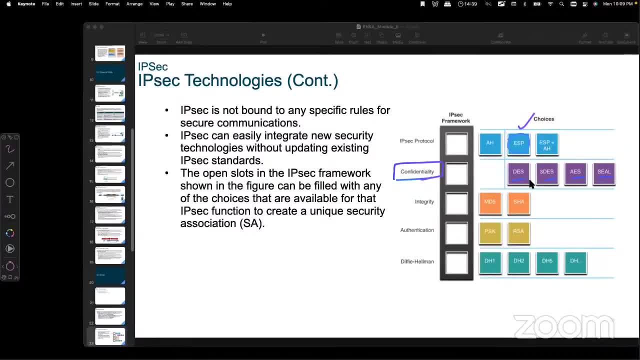 use these data encryption standard, DES, data encryption standard. so this AES is advanced encryption standard. ok, seal. I do not remember the full form of this. you can check it out. ok, this 3DS and DS. so this is 168 bit something. this DES is 56. 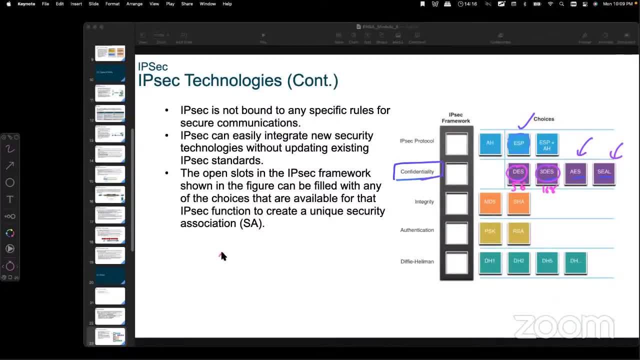 bit. so now tell me, if your password is maybe Cisco 123, ok or anything. but if you use DES, so DES is going to encrypt this data with 56 bit. maybe it will send this number. so this is the encryption, guys, this is the 56 bit. 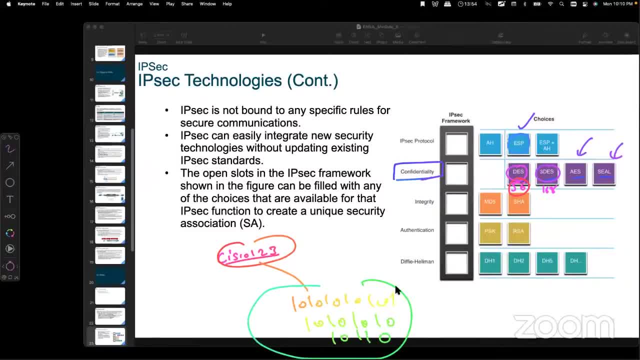 means 0 and 1, so this is the actual encryption. but if you use 3DS, maybe your encryption is this: ok, I am just typing very far, writing, ok. so what do you think which is more secure, guys? the 56 bit or 168 bit? 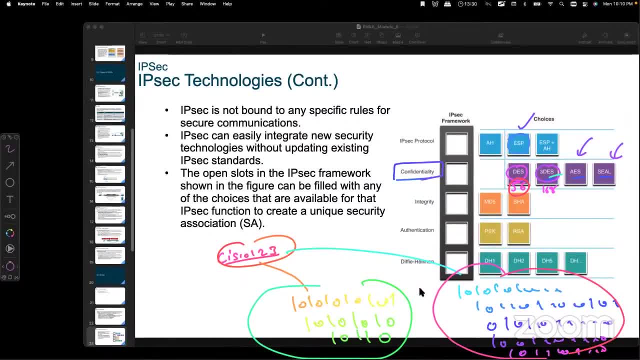 yes, 168 bit, yeah, ok. but if I am going to share the file from one router to another router, router 1 to router 2, if I am going to forward my traffic, so all data is going to add one another field of with every packet. 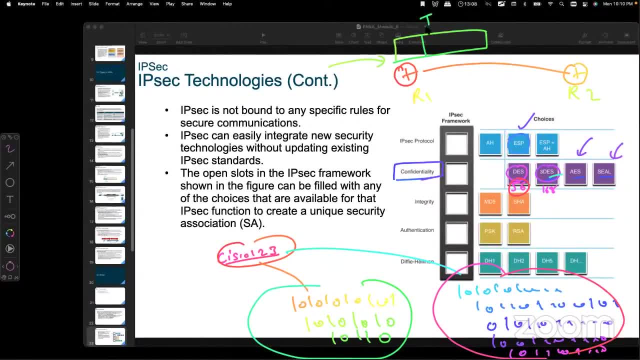 which what we will send from one router to another with IP sec. we are going to use 3DS. with every packet, 168 bit will be added for encryption. so it means whatever information you are passing. so your packet header is getting increasing and you will able. 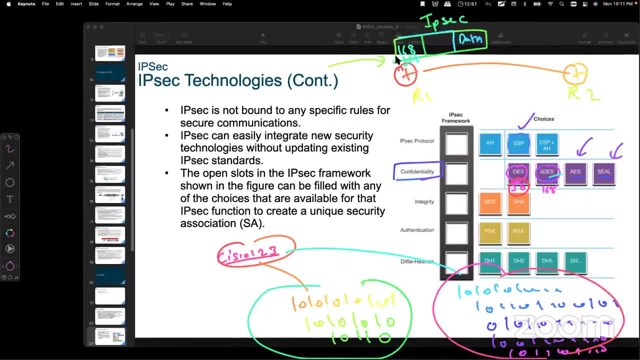 to send small data in each packet and if in every packet, if you are not able to send big, much data, what will happen? the reliability will suffer. yes, are you getting? if you put a lot of encryption, guys, but you can only send the limited data, you are. 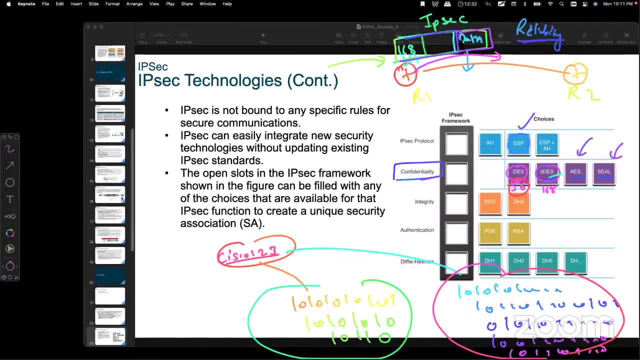 actually protecting your data, okay. but the problem, what is happening here- that you are not able to send a lot of data. so sometimes, if you need normal security, you are not actually sending a lot much secure data. so you can go for ds, only ds, also, this is. 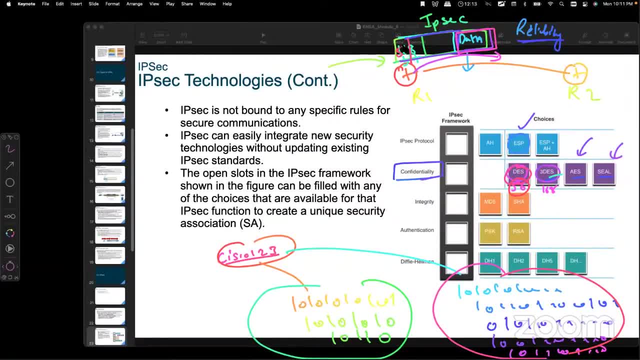 also secure. but instead of 168, it is only going to take what? 56 bit of encryption. that is also secure, but if you want high security, you can go for 3 ds. are you getting now? yes, sir, yes, sir, oh man, this is so amazing protocol. 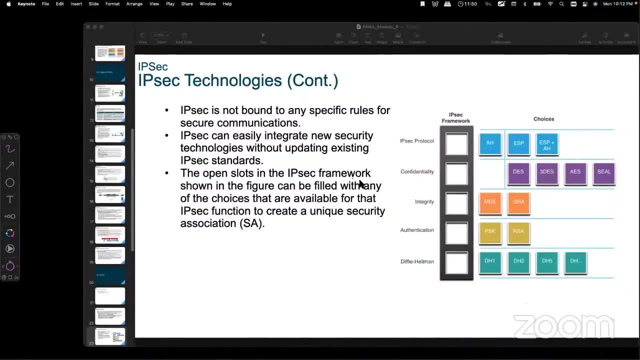 okay. so now the second is. i told you, integrity. what is integrity here? what we are doing? confidentiality is to encrypt the data so that nobody can read. yes, integrity is that nobody can alter the data. we will send the the hash codes, hash algorithm, whatever data i'm 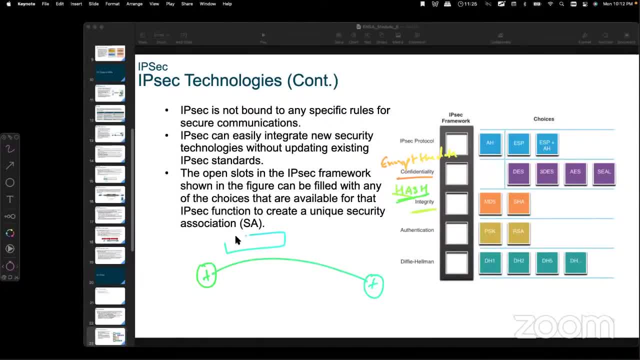 going to forward from one location to another. okay, first we will have the 3 ds or something like that, but i'm using, suppose, md5, which is called message digest 5, and this is a sha sha means sha only. okay, secure hash algorithm. i think yeah. 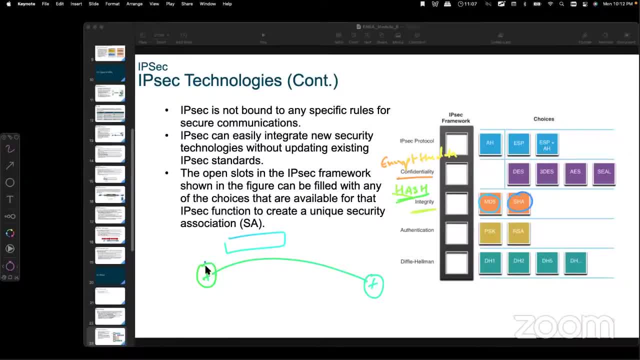 so md5 is also going to whenever you send a packet. so this packet is going to generate one code, okay, which is called hash. suppose this is my hash algorithm. okay, this is one hash. so if this number is, we are sending from this side, from delhi. 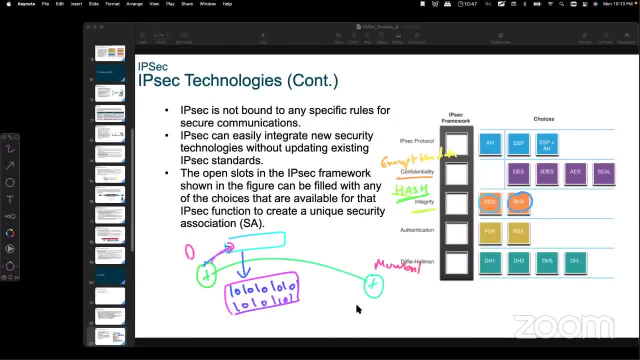 mumbai got to know this message. okay, 101 same thing. so if everything, even single 01, everything is same, it means both the side. hash is same, yes or no. so the hash is same both the side, if anybody try to alter this data. so what will? 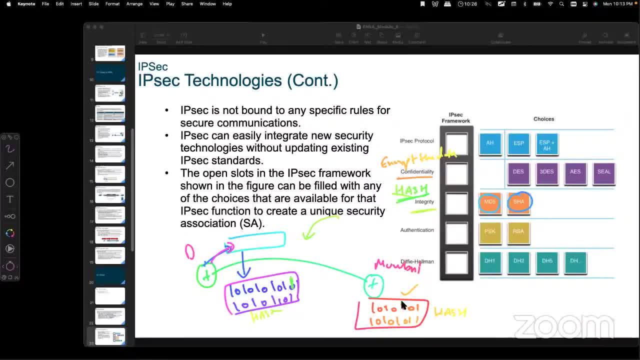 happen? the hash numbers will change, yes or no. if anybody try to steal information, what will happen? the hash will be changed and if hash values are not same, the mumbai router will discard. this packet are you getting now? hash is basically a secure number. okay, so the 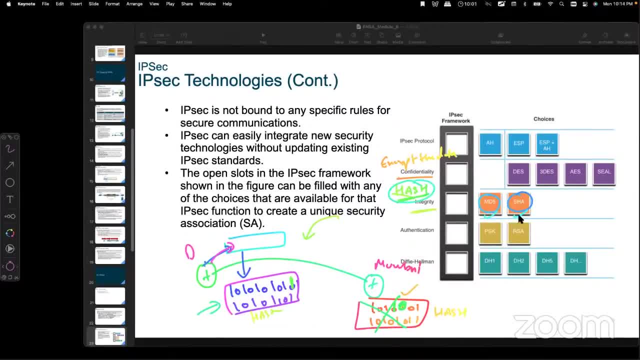 hash, basically md5 and sha. it is going to generate one number, maybe 0, 1, 7, 6, 2, 3, 5, like hash, 1, 2, 3, like this number. so if this number from source side and from the destination side, 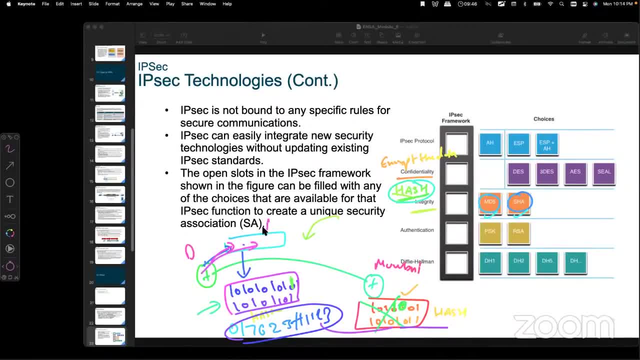 if both. when you send a packet, you send a hash here, yeah, you send a hash code here, and when the destination will see, okay, and it will see okay, the hash is the same or not. okay, so the hash number is: just suppose I am sending you a. 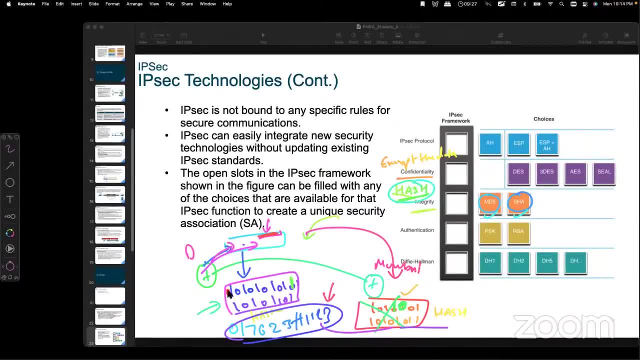 courier. but I will just mark here a red with some what we call. I will just mark: suppose this is a courier, okay, and I will put a glue here, okay, and maybe I will just mark here that is some red dot, that nobody, whenever somebody try it to. 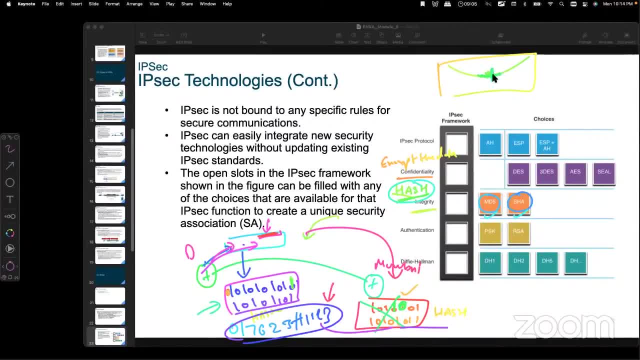 open this. okay, so this glue or this mark will be like: will tell that receiver that somebody try to open this right. the same way you are putting a number or secure hash so that the receiver router will come to know. okay, this code is same, so this is. 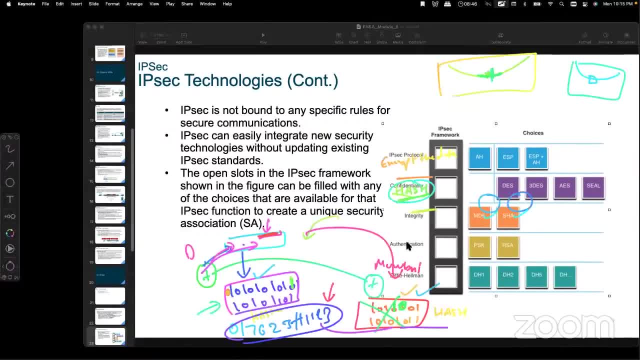 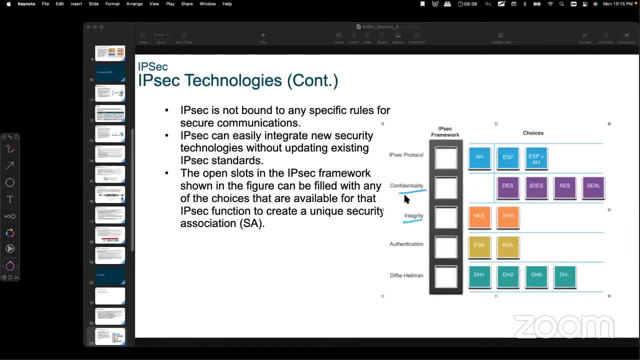 how they protect the integrity means the sender and the receiver is same, okay, and nobody try to send or alter the data. clear, yes, okay. the third method is authentication. so one is called pre shared key and one is called rivest shemeral min edelman even. 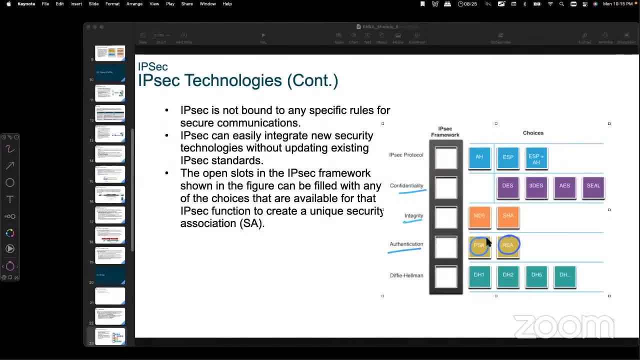 tongue twister. okay, so these are tongue twisters. pre shared key means if you use psk, psk is pre shared key. you will just enter a password: cisco 123 hash. like this, and on the other end also, you have to send cisco 123. 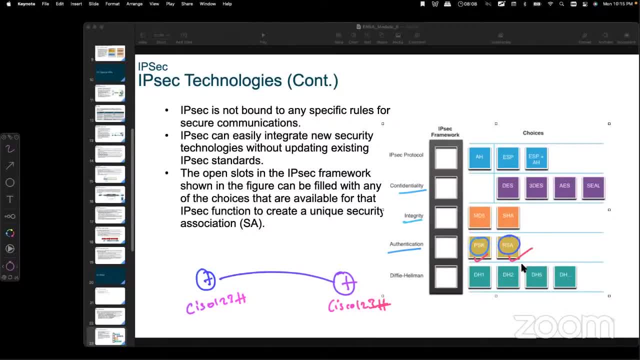 hash. this is called pre shared key. but when you use rsa, okay. so when we use rsa, rivest shemeral, min edelman- these are three scientists who made this. remember? the ssh protocol works on rsa algorithm. yes, sir, yeah, so this is the same algorithm. we. 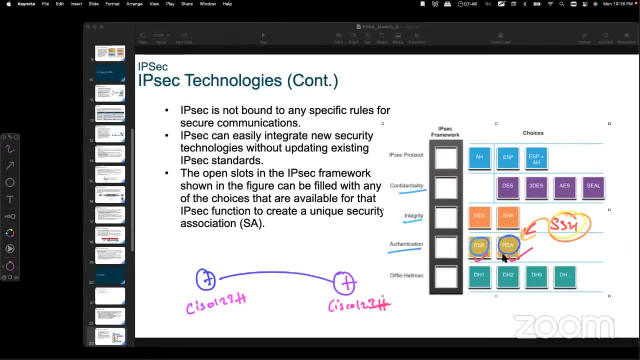 use for secure shell, so rsa and psk. if you use rsa, so then you need to generate the digital certificates, like we generate on ssh, so we can use rsa also for authentication. but yes, pre shared key is better. we can put a password here we can add. 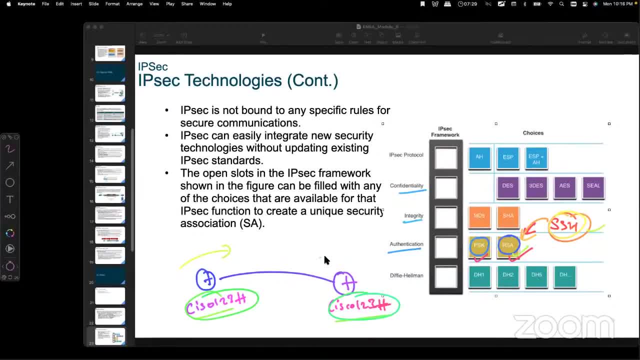 a password here and that's it okay. after that, these are the defi helman. so there are different, different ways. defi helman one, defi helman two, five and six okay nowadays, maybe new versions also. so if you check the security, if you use, 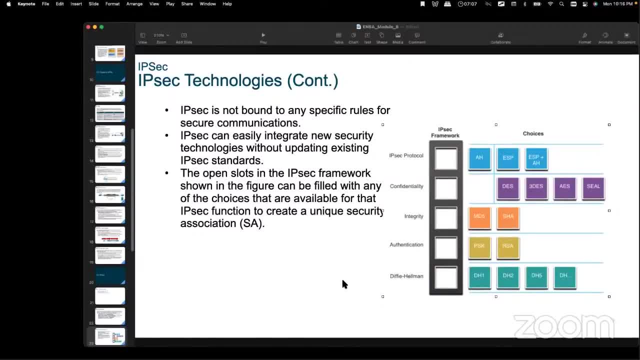 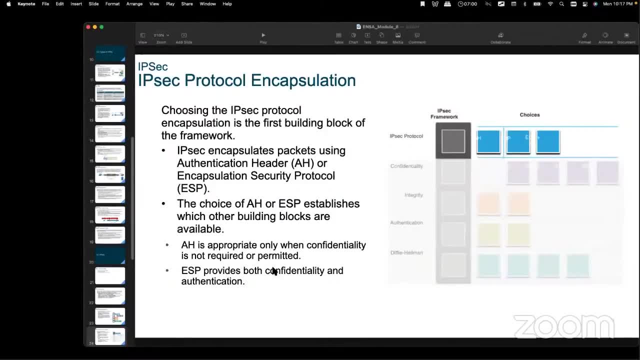 one, two, three or one or two. so there is a difference between the encryption method. so now you can see with the slides. also, ipsec uses authentication header and the esp encapsulation security payload. so ah is appropriate only when confidentiality is not required and esp provide both. 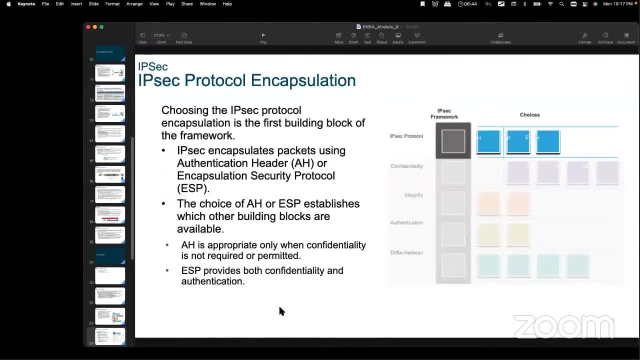 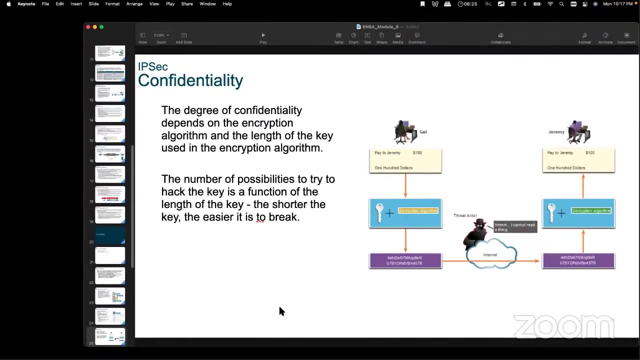 confidentiality and authentication. it means it is. also it is going to encrypt the data. if somebody ask an interview, what is esp and ah? esp, secure the, encrypt the data also, but ah, just encrypt the headers, not a data. okay, so this is confidentiality, guys. i told you this. 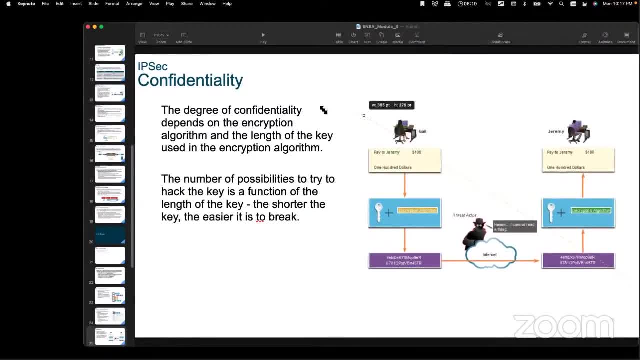 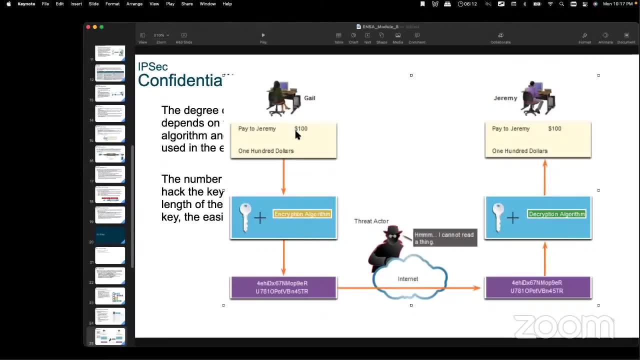 is where suppose this? you can take this example that this user, gail and jeremy, okay, so this gail has transferred one amount, 100 dollars. so this encryption algorithm is going to encrypt that hundred dollar transaction into some code. but if somebody try to the threat. 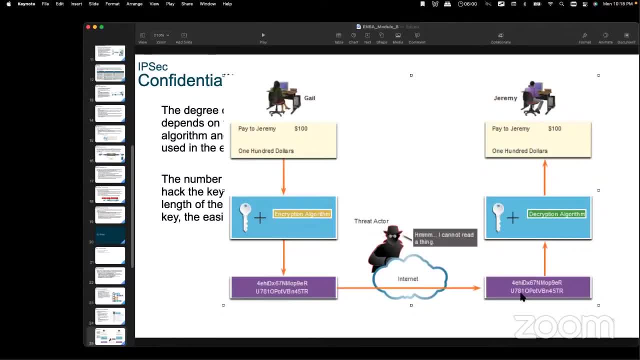 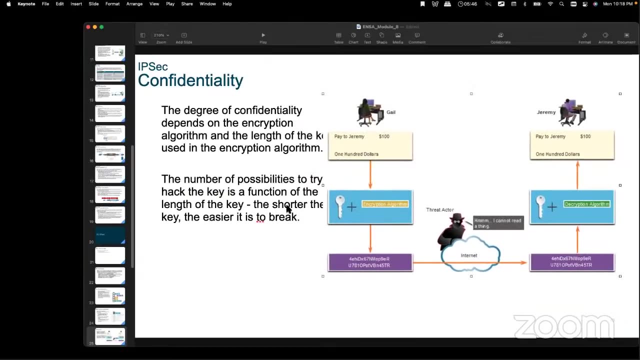 or intruder, so that intruder cannot read this data, and there, on the other end, the decryption algorithm will actually tell: yes, the amount is getting transferred. so this is called confidentiality, confidentiality, okay, confidentiality, both, sorry tank twisters. okay, let's go ahead. so when we talk, 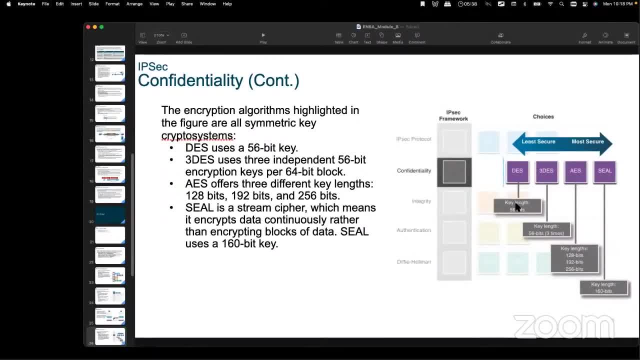 about confidentiality. okay, so ds, i told you 56 bit 3, ds is 56 into 3 and if you calculate it comes around the- i think 168 or something you can calculate, and as is a 128, 192 and 256, and seal is: 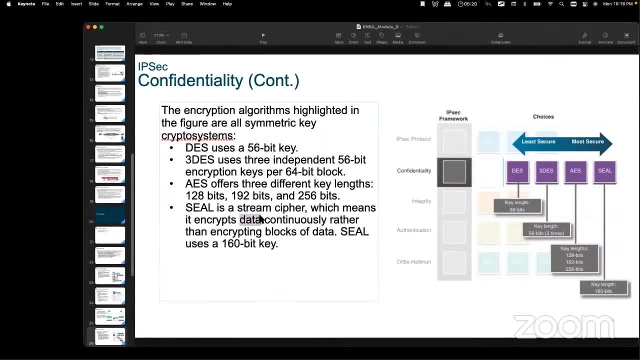 basically a stream cipher- this is the full form, i think okay, which encrypts the data: 150, 60. so the least secure is ds, the high secure is seal, which is, but syscode router do not. i think they support the latest devices but the normal syscode. 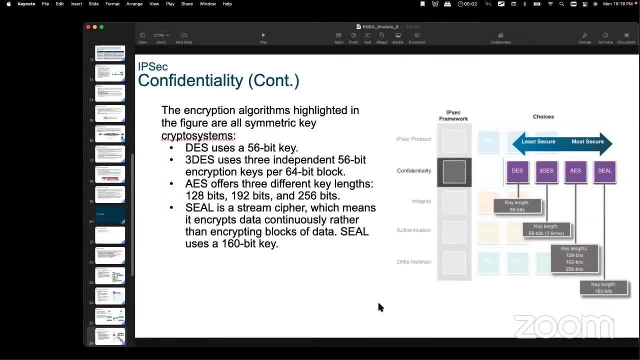 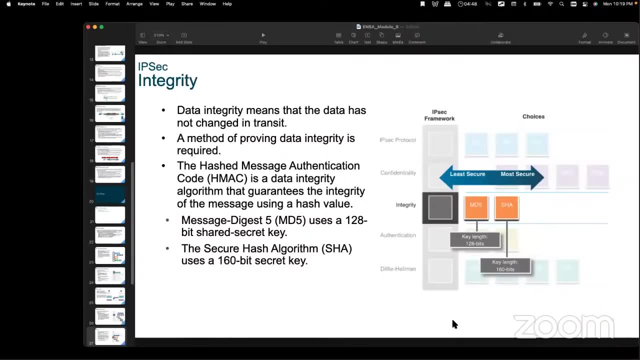 devices. they support 3ds and as so. when we talk about confidentiality, which is actually going to encrypt the data- okay, so it encrypts the data continuously- and when we talk about integrity, integrity is shy- is 160 bit, md5 is 120 bit the shy. 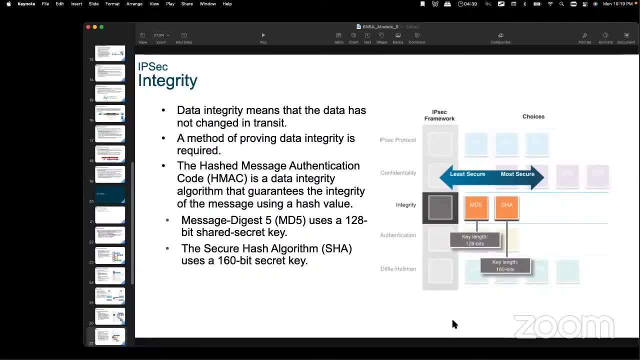 is more secure, which is called secure hash algorithm, and these two hash algorithms are used for data algorithm. that guarantees integrity, that nobody has changed the packet. nobody can change the packet because whenever you send a packet you will put a hash message authentication code with every packet. you 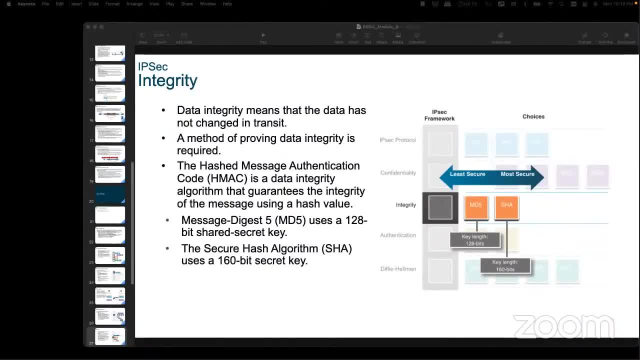 are going to send hash mac in ipsec and when you will forward that h mac will be actually a data or it is like a encryption. okay, so there are some formulas which is going inside the ipsec, so this is also called hash values. also, i'm 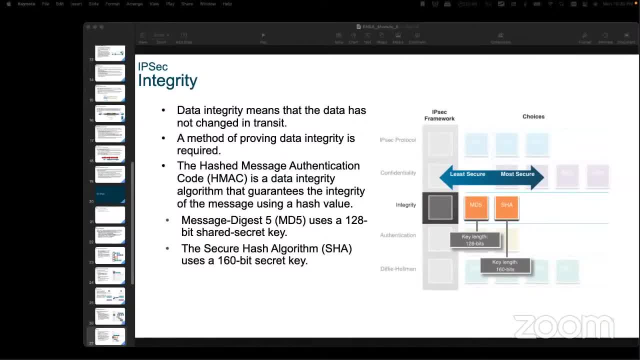 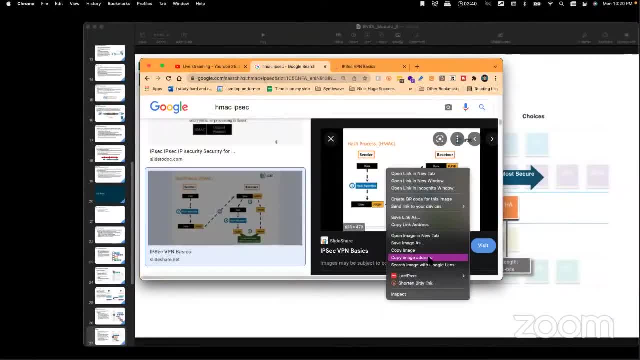 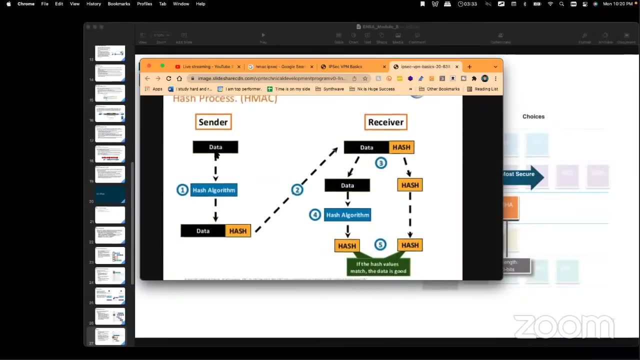 trying to show you something. okay. so i just, yeah, you can see, i am sure you guys can see this okay. yeah, so you can see here, guys. so whenever we send a data, we also add a hash algorithm, which is md5 or hash. so whenever we with 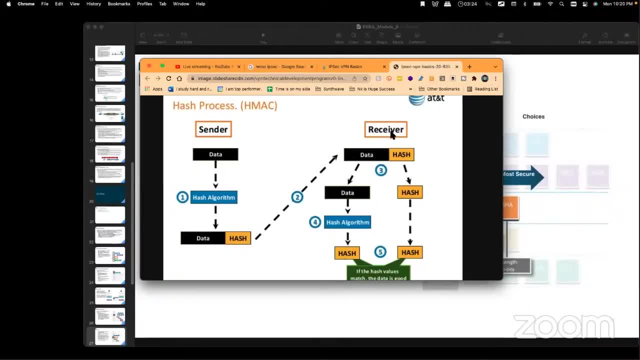 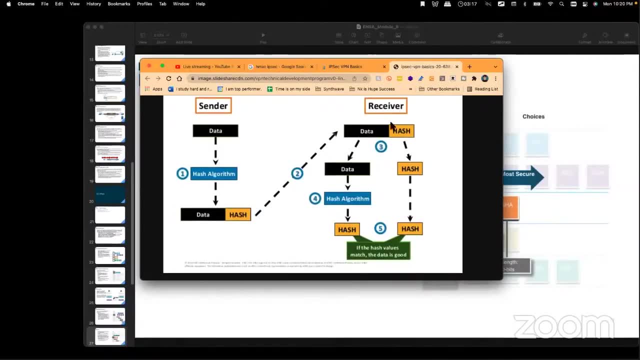 the data, we will send a hash value. and when the receiver receive the data, so it is going to check the hash values. so because there is hash value in the data also and there is a hash also, so now inside the data, hash value and the hash value. 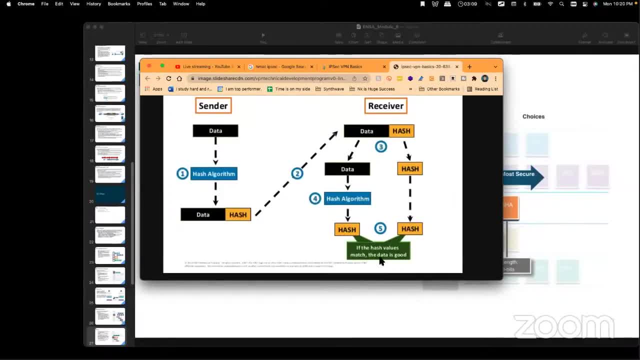 we sent. so if that is matched, so the data is good. if that is not matched, the data will be not accepted. okay, so it means. so whatever hash value we are sending from here, that hash value copy is inside the data and when we receiver received it. so 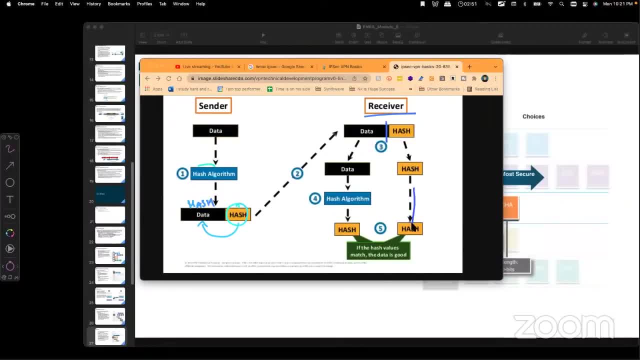 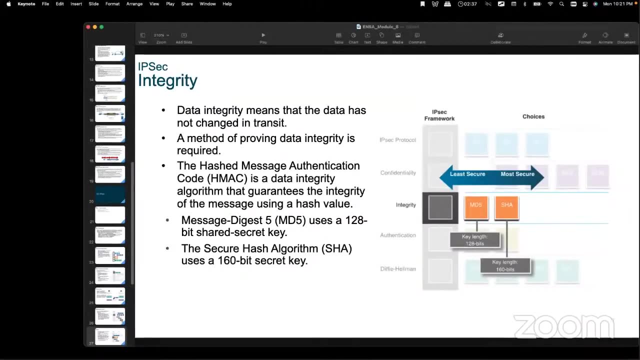 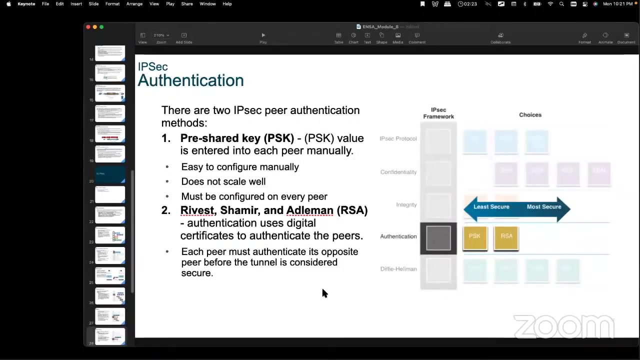 the data and hash will be matched and if that is matched, the data is good. else the data is bad or the packet will be discarded. is this clear, everyone, hello, hello, hello. yes, sir, good, okay. the third thing is authentication. I told you we will use the pre. 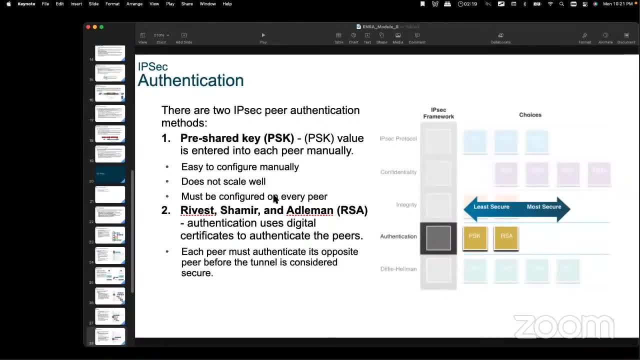 shared key which is, like, easy to configure and must be configured in every state. so if you use this algorithm, which is RSA, so we will use digital certificates to authenticate the routers or devices. okay, this class is very important because even if you go for AWS, Azure or 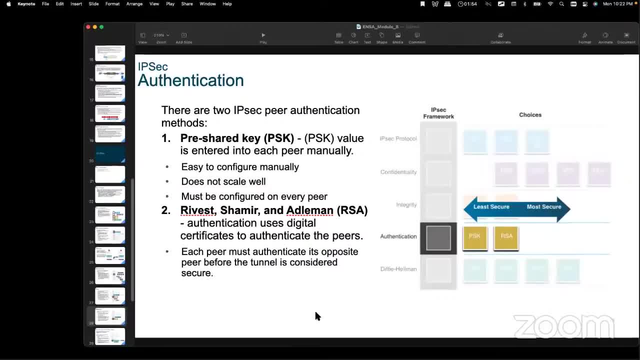 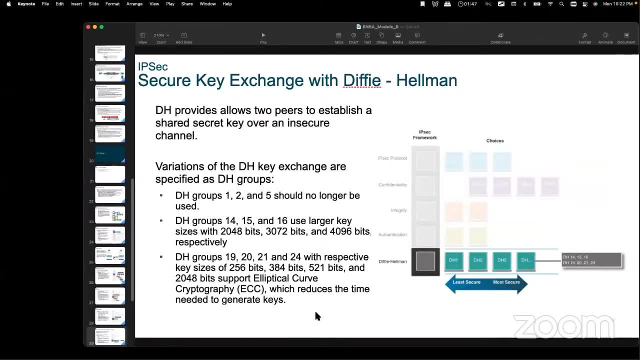 any kind of cloud platforms. also, all the tunnels are created on this protocol, IPSec. okay, so till the time you do not understand very well, keep learning this. I am sure this is the most simple IPSec class ever as anybody has taken. I am sure if you, 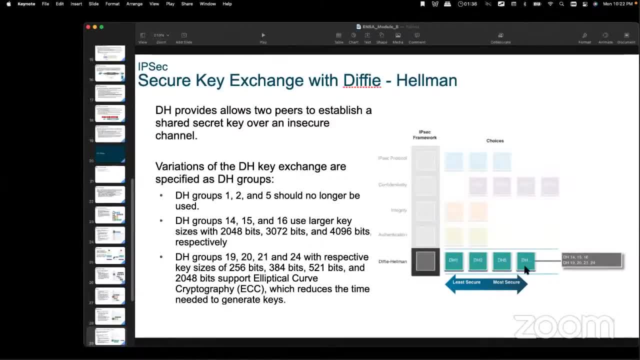 guys tried earlier. okay, so this is DeFi Helmet 257 and these are 14,, 15,, 16,, 19, 20- a lot many available. so if you use DeFi Helmet, what will happen? the two peer remember that thing that we. 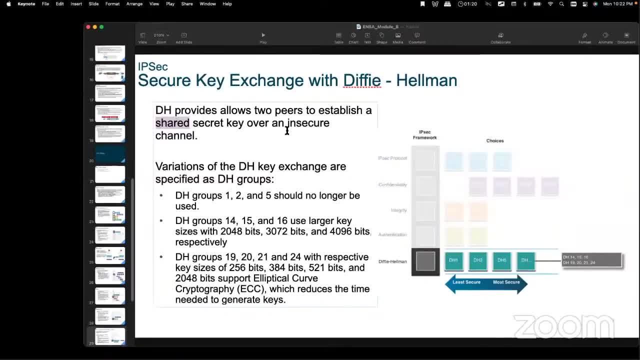 are going to share the secret keys, okay. so DeFi Helmet provides allows two peer to establish a shared secret key over an insecure channel. it means that we are going to agree on one number, okay, and that number will be not shared. the private key will not be. 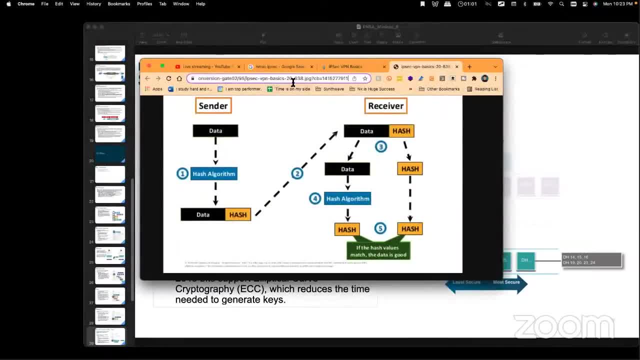 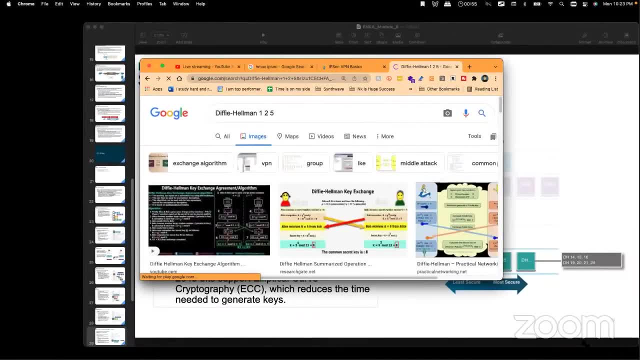 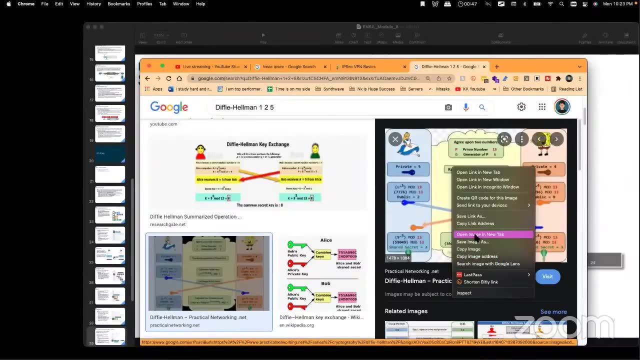 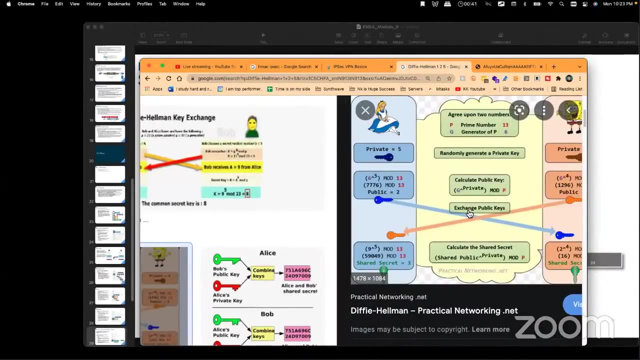 shared. let me show you that. also. the DH DeFi Helmet 125 like this. okay, so this is the actually concept. okay, the image is very small so I'm sure you guys can read this. this is so you can see. these are two devices. okay, do not. 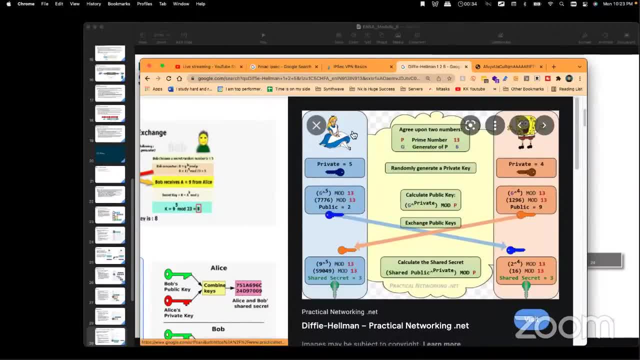 see here the girl and this cheese, kind of stuff. so just understand. these are two devices, so both are going to generate a prime number. okay, so both will agree on prime number. so one agree on 13, and then there is called a generator which is like a. 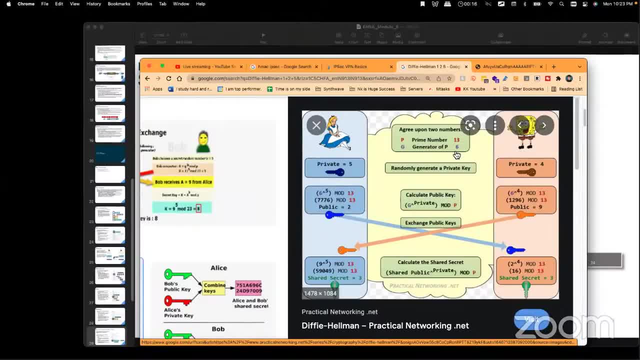 random generated by devices, like six. okay then. so then both the devices are going to generate a private key, so you can see: private key five, private key four, and there is some math which is like six to the power of five, which is this number generator, and we 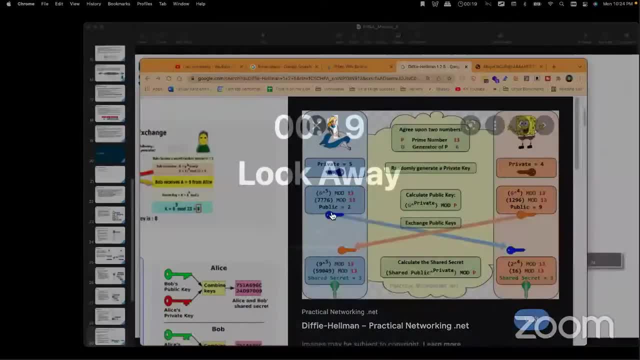 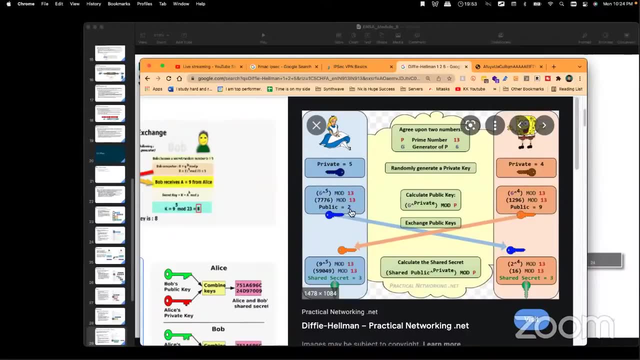 will have the power of five, which is a private key, and then we are going to mode this with 30 number and when you calculate there is a value which is called public key. so this public key we are going to share with both devices, but this public 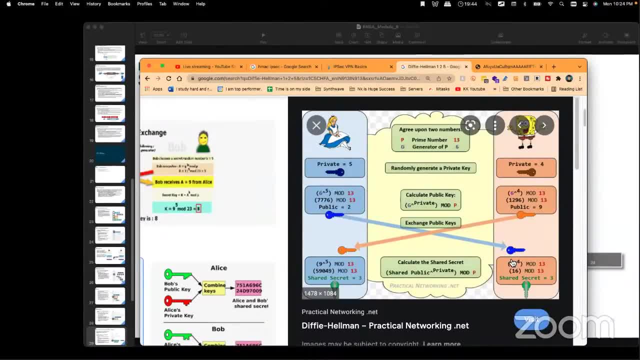 key. nobody can modify this public key because internally, the defi helman is when you share your public key and when this router is going to share the public key, the router is going to agree on the shared secret. can you see? the shared secret is same of. 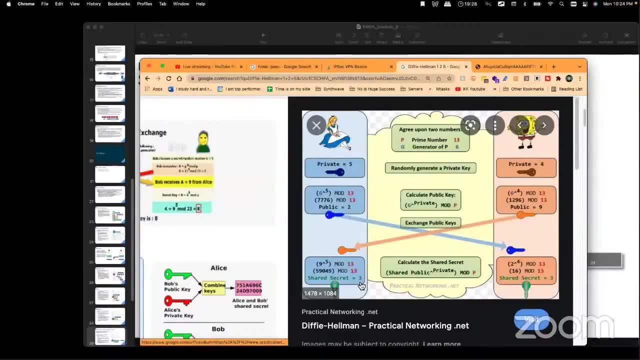 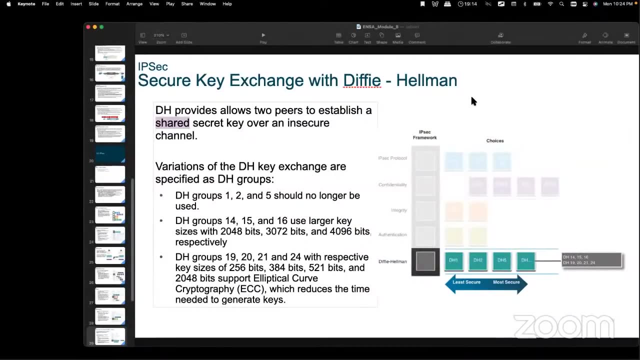 both the sides. can you see that guys shared secret three. shared secret three. right, so then they will come to know. okay, this is my shared key, and if shared secret number is same, it means we have actually transferred the keys very well, and now we are actually sending. 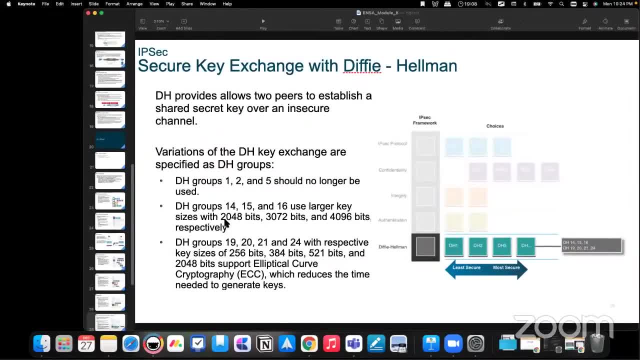 the information correctly. so if you want to share the keys with the normal method, so one to five, you can use. but if you want high security, 2048 bit, if you use this defi, helman 15, group 3078, so can you see the? 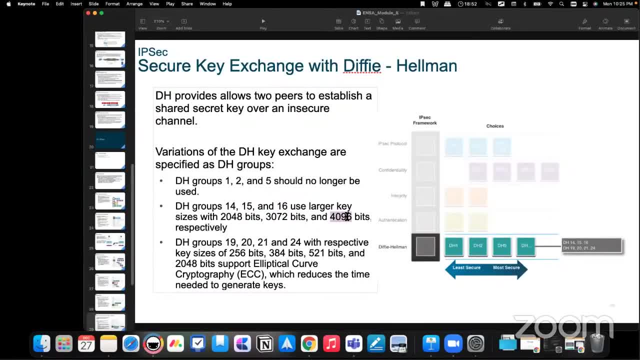 number is increasing, the bits are increasing. it means whenever we are going to use all these methods. so this is all going to secure more. if you use a defi helman, yes, tell me. so that is basically a cryptographic year, okay, so prime number you have to. 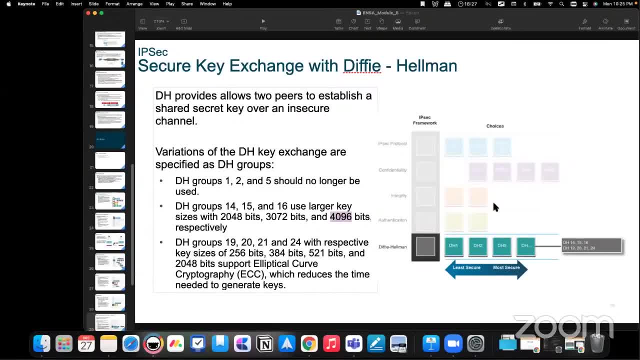 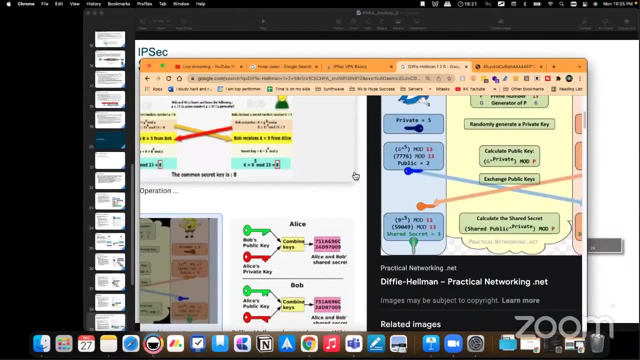 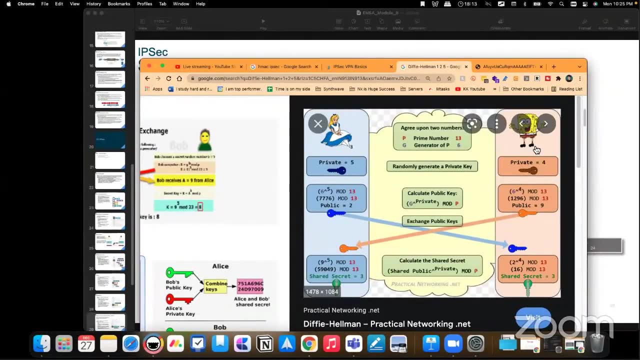 learn like cryptographic books. if you want to completely understand that prime number is basically like what i have understood till now, that both devices will agree on prime number, that agree upon two numbers. can you see that agree upon two numbers? yes, devices will agree on two numbers, one. 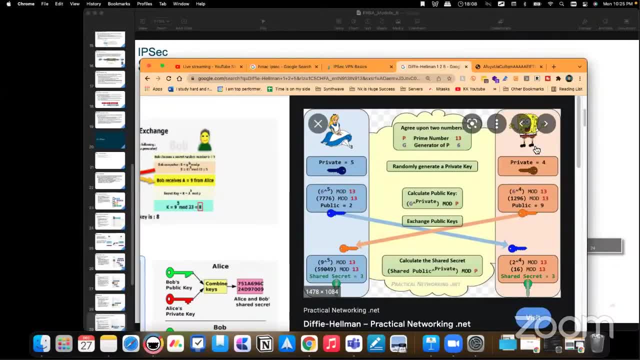 will be called prime number. one will be called generator of prime number which is six. okay, so this is generated by both the devices. and then there is is some formula which is like this: g into private key and mode with the prime number. so g is generator which. 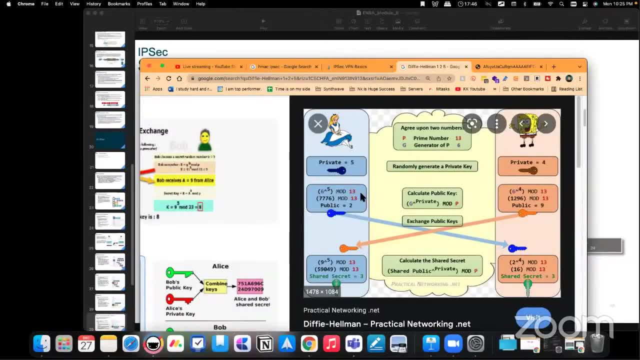 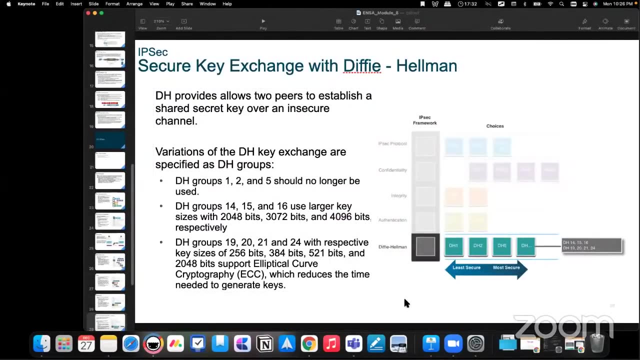 is six, private key number five and the mode is thirteen. and then they have, they calculate this number: public value two. okay, so this is internal formula. i'm just showing you, to elaborate it more, how it is actually working. but actually, that's you. if you learn the 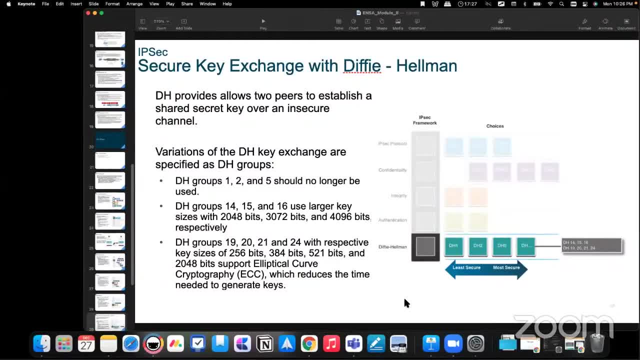 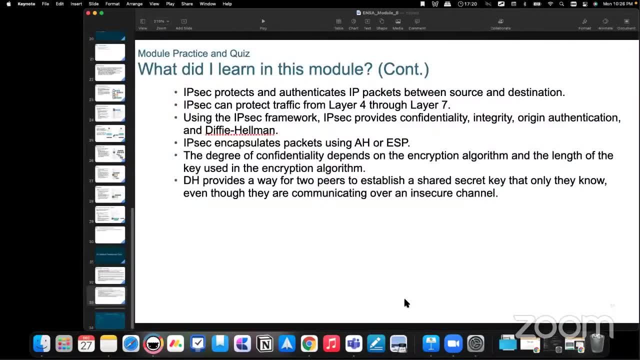 cryptography, cyber. okay, so this is ipsec, guys, if you understand this, like i'll tell you, ipsec protects an authenticate ip packet between source and destination. in ipsec, we encapsulate the packet with either ah or esp, which esp is more popular, and when we talk, 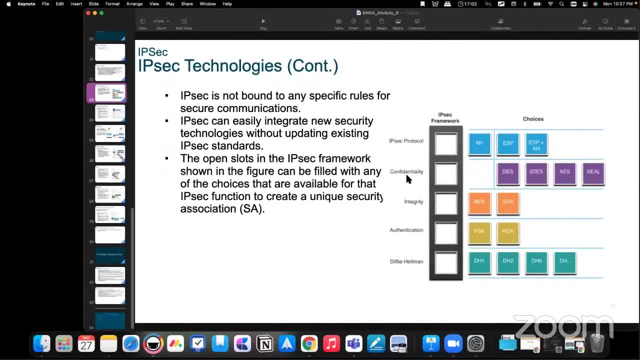 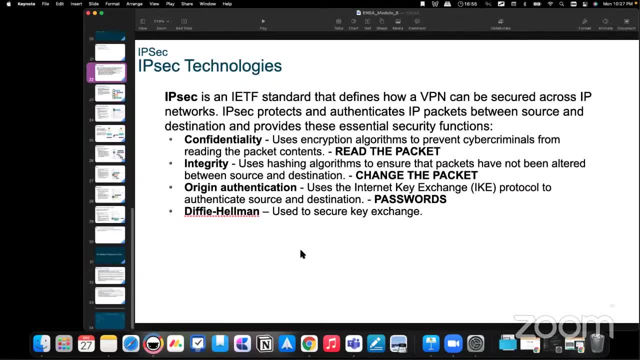 about ipsec. ipsec provide confidentiality, integrity, authentication and fv element to secure the keys in a very appropriate manner or secure the key exchange. so you can see here. so let's revise. confidentiality uses encryption algorithm to prevent cyber criminals to read the packet. integrity means hash values. 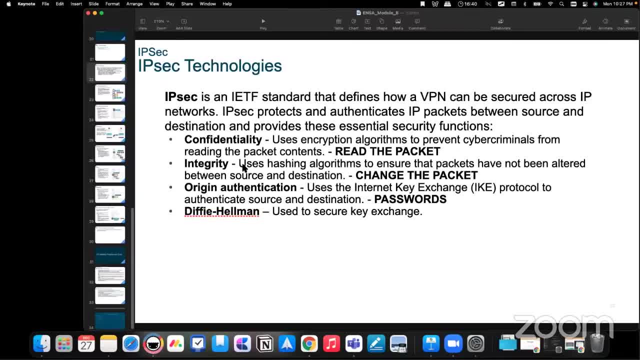 okay, remember that it will divide and inside the data it will match the hash. if the hash values are same, it will accept. if the hash values are not same, it will reject the packet. okay, this is useful when you want that. nobody will change the packet then. third, 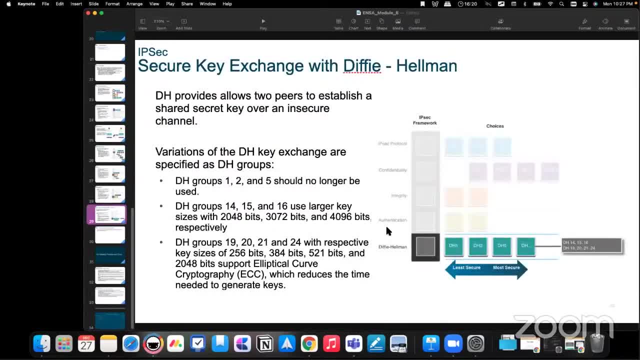 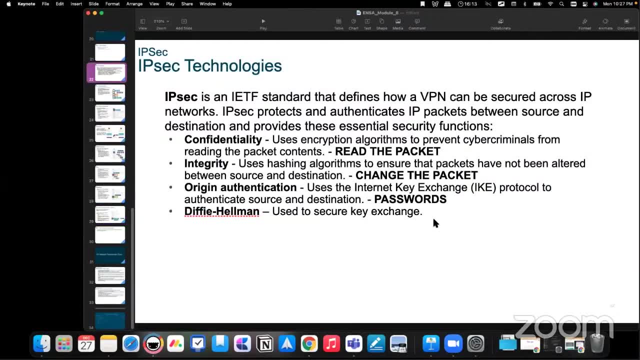 is about that key exchange. okay, that is called authentication. so authentication is basically: we are going to set a password from one side and the similar password you need on other side, and then the defi helmet method, that we are going to use the secure method to exchange. 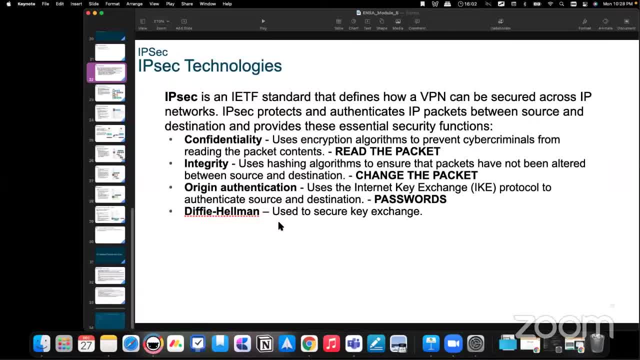 the keys, because if key is actually copied so maybe the data will on the risk. so we are going to protect the keys. so this is the key. who will secure these keys? whatever password you will set here, the keys will be secured by defi helmet so that 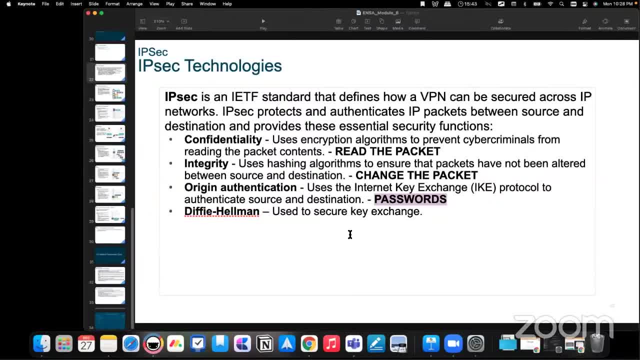 they will randomly generate prime number and the generator, then there is a formula, something okay. then they will come on and agree on the shared secret and this means that, yes, we are successfully secured the keys. okay. so, guys, this is all about today's session. I hope you guys. 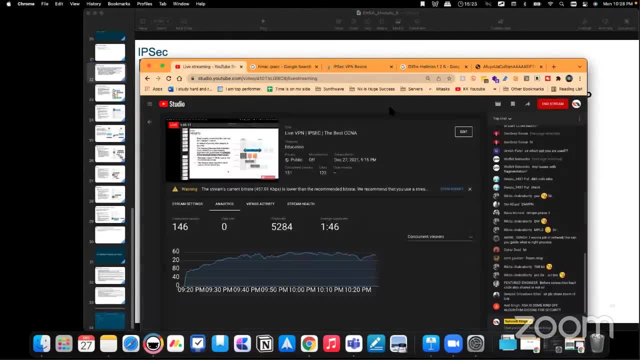 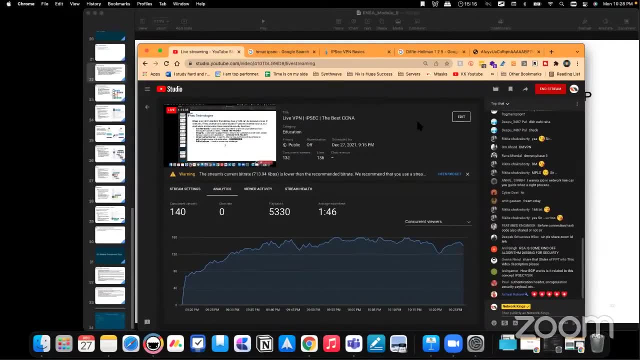 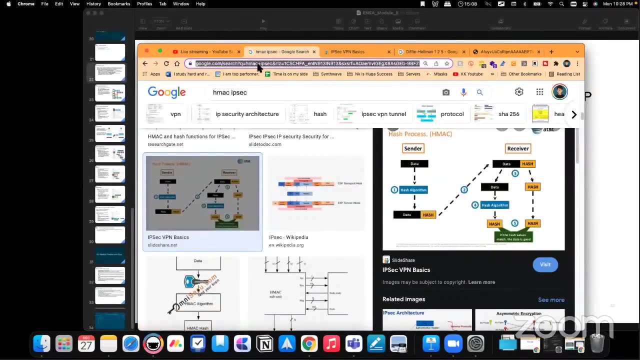 enjoyed this, right? no, no, like. this is not part of growth, this is not part of network, this is for cryptography and all, and why you have to like yes if you have more interest in knowing the defi helmet. okay, so you guys? yeah, so defi helmet. 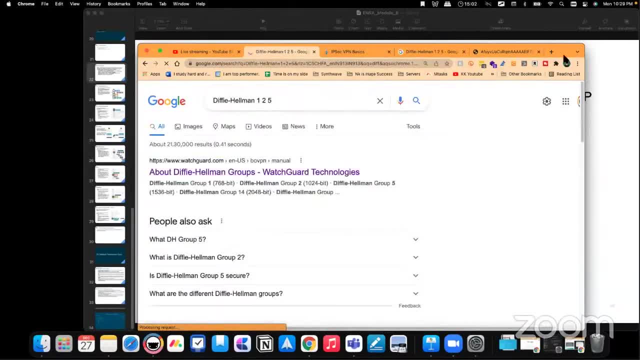 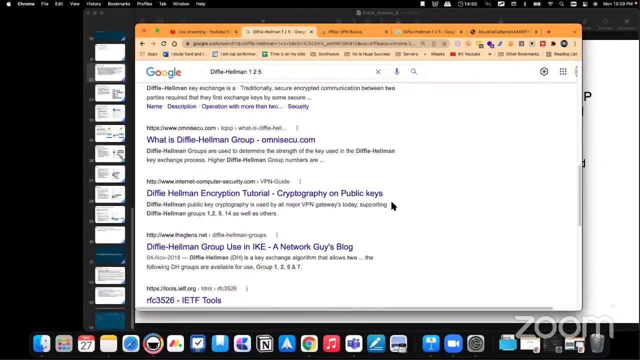 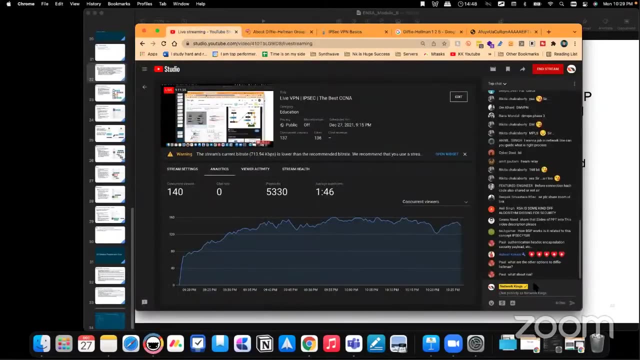 videos on youtube. we have not made defi helmet videos so you can check maybe some other youtuber videos, so, or maybe somebody has tried to okay, okay, sir, sir, please, let us just repeat: in sure, sure we will. we will share interesting here, sir, yes, no. 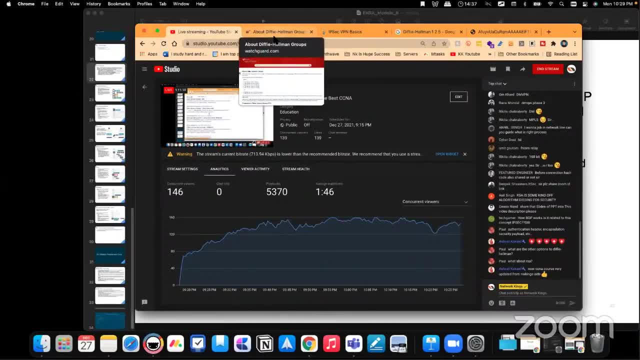 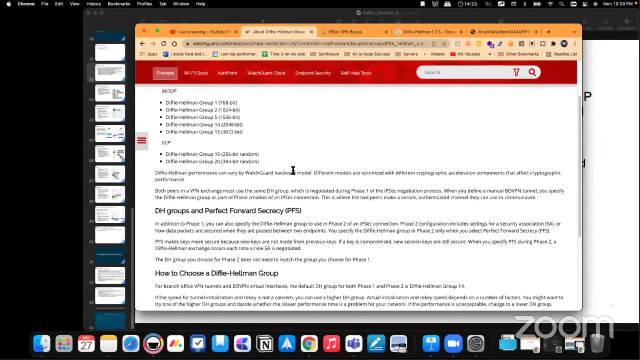 issue? no issue, I have already shared my information. if you want more in depth, because I am not from security background, maybe when you learn firewall, you can ask your training us at that time. okay, yeah, but yes, trust me, this is the highest in depth level of IP. 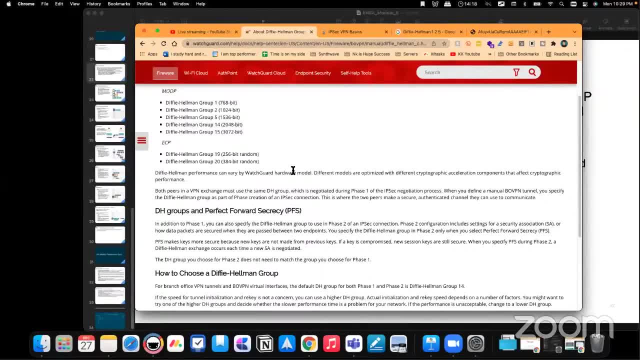 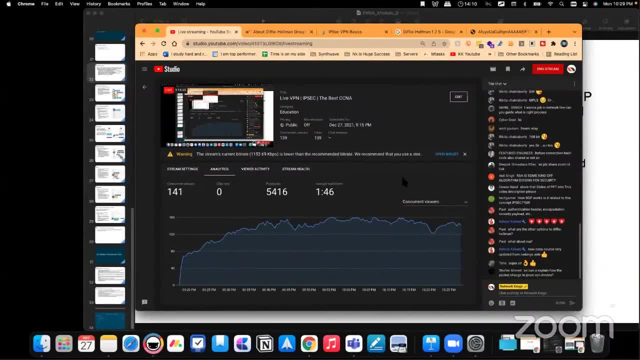 sec today. what we have covered, the people who learn: yeah, yeah, so it means now you are good at security, you should make your career in cyber security or security. yeah, so what we did here we understand. we understood the IP sec how it works, but how we are, 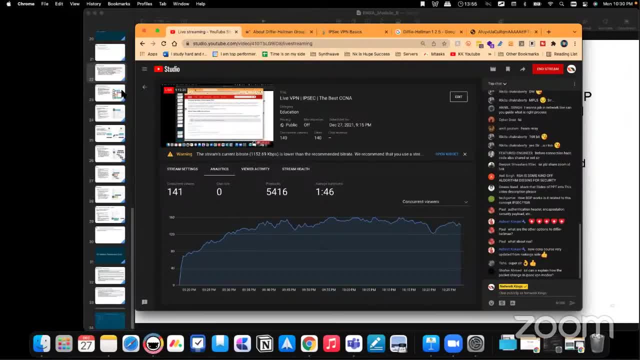 going to make IP sec tunnels and all that is a part of CCNP and maybe I'll put it on YouTube also. but that's not commitment, because my next CCNP batch coming soon and IP sec is always the last topic- maybe two, three months, you guys. 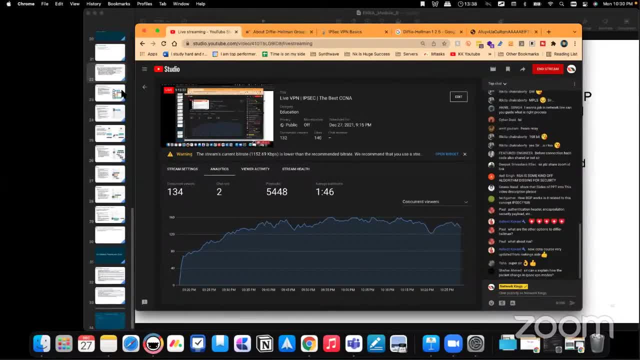 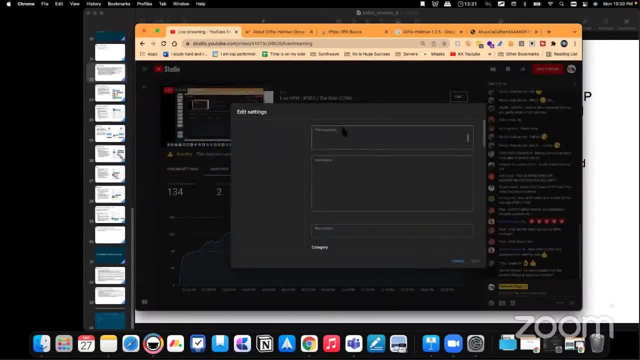 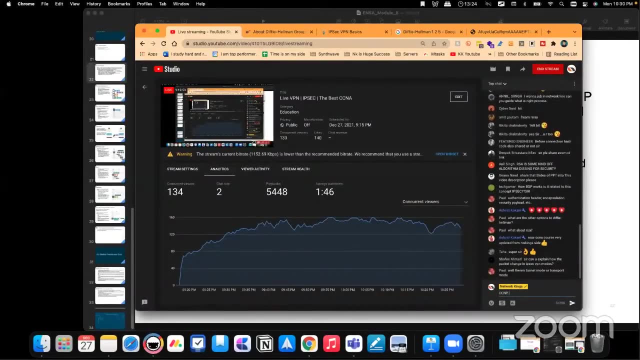 have to wait for CCNP, IP, sec, okay. so how? okay, guys. thank you very much. if anybody is interested, like we, I am talking to the YouTube guys, those who want to. yeah. yeah, sir, for resume I requested, please give me. okay, I will share the resume template. 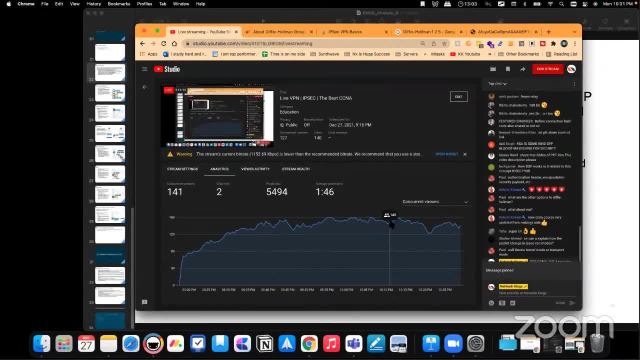 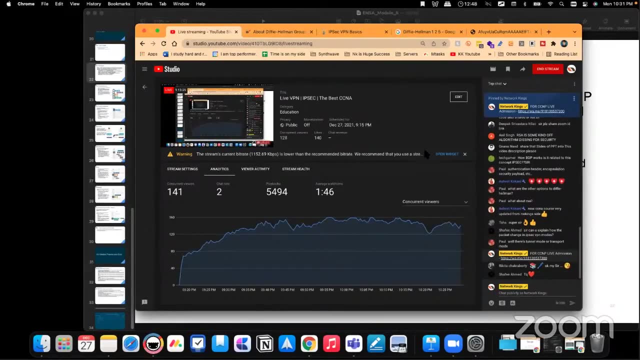 with you all. okay, okay, I'll share, but I I do not have a dog file, I have this normal template file. okay, okay, okay, yeah, thank you, okay guys, thank you very much. see you all. bye-bye, good night, good night, okay, thank you sir.